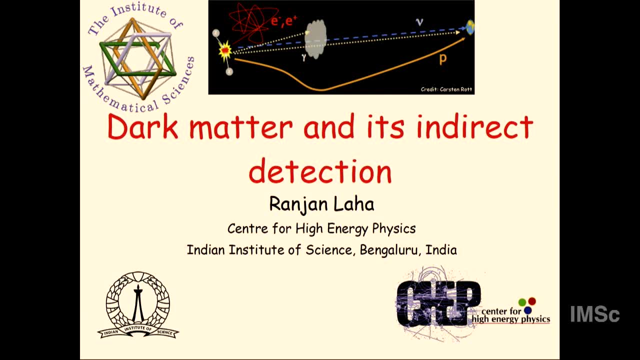 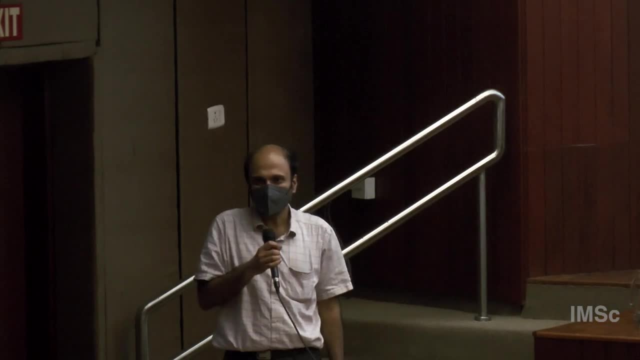 not even two years. So before that he did his PhD at Ohio State University and after his post-doctoral stints at SLAC or Stanford University he was a joint position there and University of Mainz. and then he was a fellow at CERN, post-doctoral fellow, and then thereafter 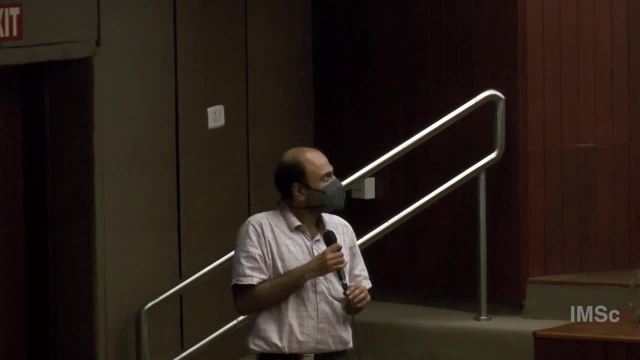 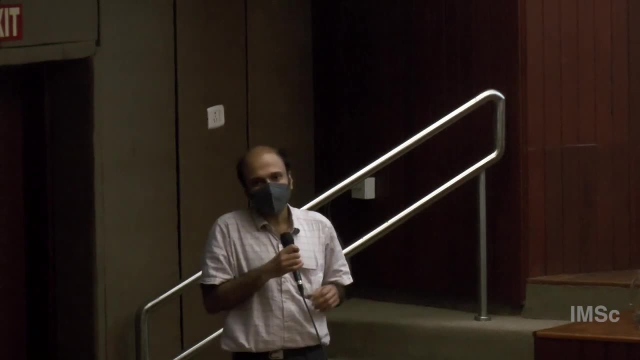 he returned back to India. So he works in very interesting topics on dark matter, its indirect detection and many other topics in astroparticle physics, which is a very important area of research current times because in the next decade it will be a very important area of research, because in the next decade it will be a very important area of research, because in the next. 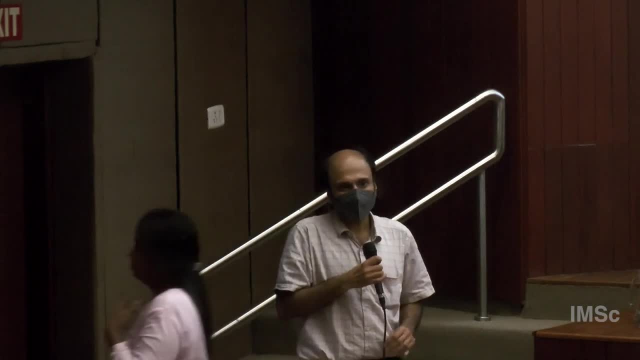 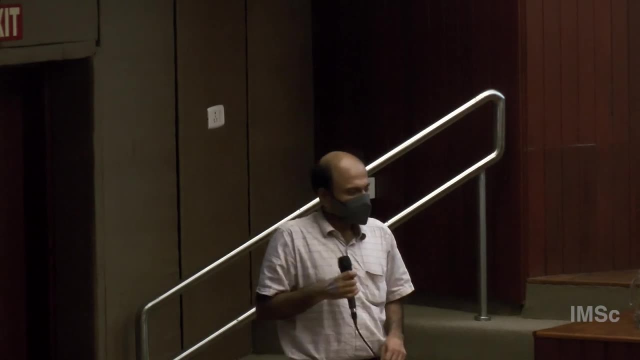 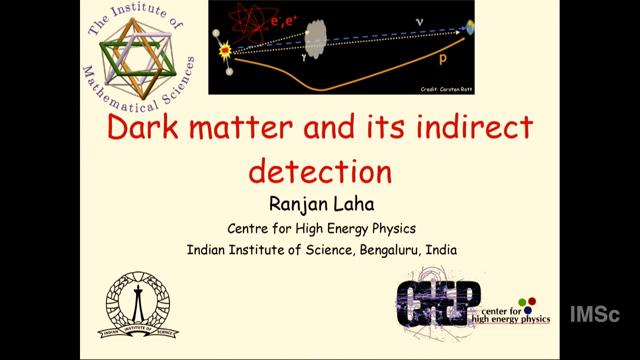 generation, we will have a lot of experimental efforts towards detecting such particles, and so he is working on several such topics, but today he decided to tell us more about dark matter and its indirect detection. So, Ranjan, please, Okay, good. So as faces, or in fact, as human beings from time eternity, we have asked a very basic. 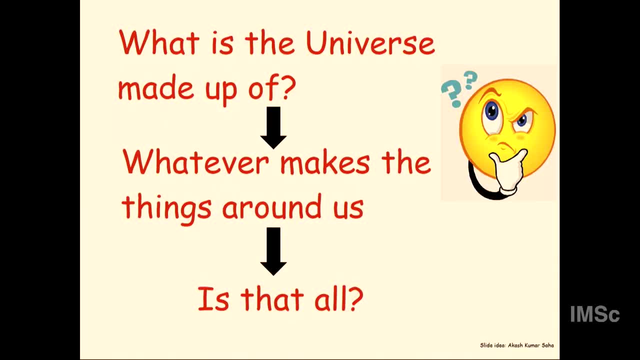 question: What is the universe made up of? Right, This is, I mean. you look up at the sky, you look everything around you and you will ask this question: what is the universe made up of? So, for as long as human beings have existed, till until, say, last few decades, the answer was: whatever makes the things. 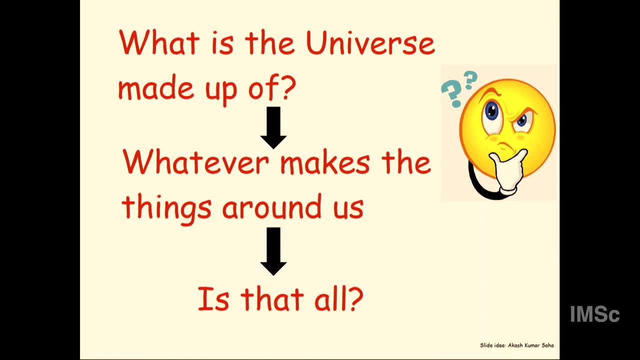 around us All right? Turns out that you could have asked the question: is that all Does the universe? is the universe made up of things we can see around us? And that would not have the opportunity to even answer that question. The last few decades in physics and science in general has late. 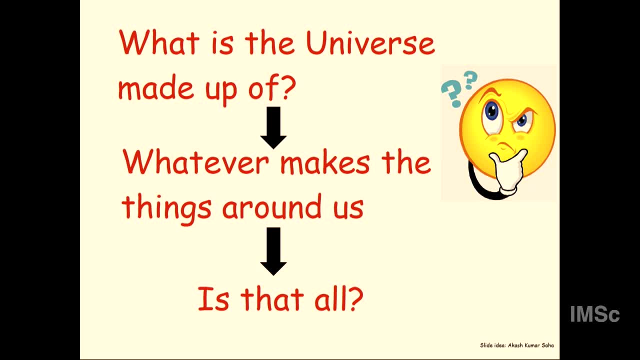 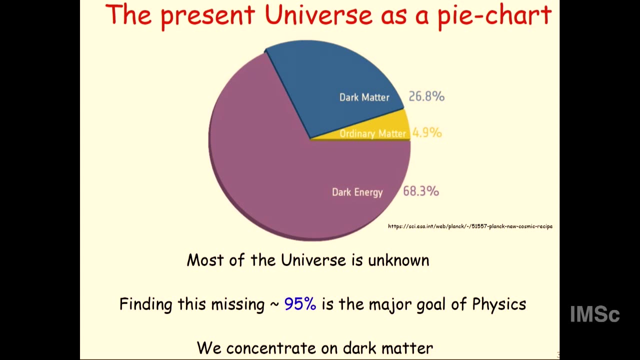 revolutionary noodles. we can now answer this question. Is that answer is all? All the answers is no Right. One thing can do due to remarkable measurements of the cosmic microwave background that is basically a light, that is person from big bang. big bang is the start of the universe. you can think of it that way. 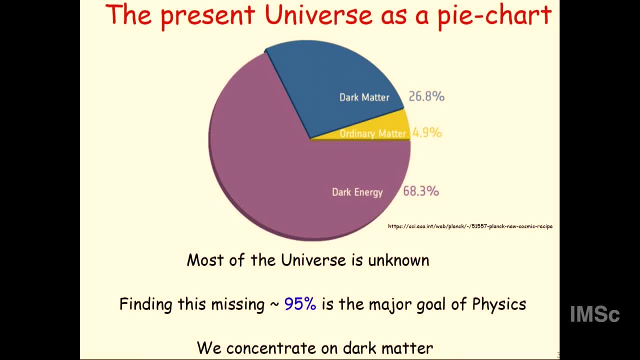 is to measure the energy density of the universe, and this is the pie chart of the energy density of the universe. all right, so everything that you see around you, right, everything- makes up about 4.9 percent of the energy density of the universe. this number is known to a precision less than one. 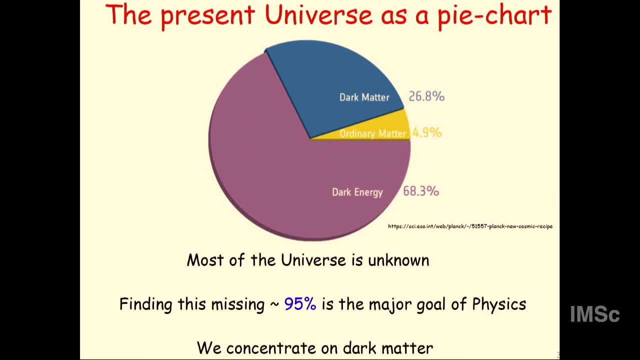 percent, all right. the remaining 95 percent is something which we do not know anything about. all right. something like 27 percent makes up dark matter. this number is known to a precision of one percent. 1.5 percent, roughly, all right, and the remaining is something even more mysterious. 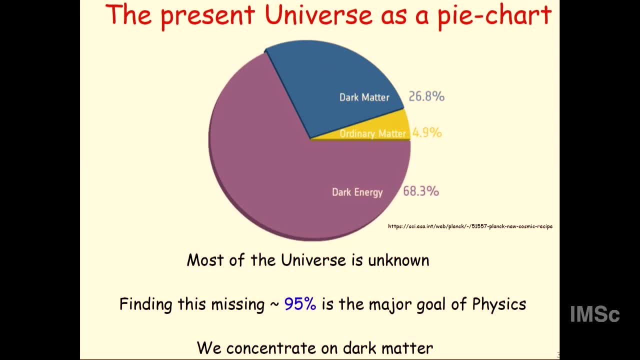 called dark energy, which makes up 68 percent of the energy density of the universe and that is known to a precision of 1.5 percent of the universe, and that is known to a precision of, again, two percent accuracy. this number, this number is known to two percent accuracy. so these 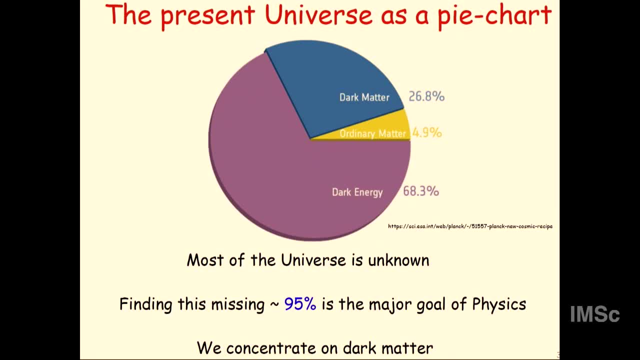 are numbers which are measured, measured extremely accurately, from cosmological observations. right, and this tells you that we only know five percent of the universe. all right, the remaining 95 percent is completely unknown, and this is something we have only known for the last few decades. all right, this, this, this pie chart, was made only in the last few decades, like all the. 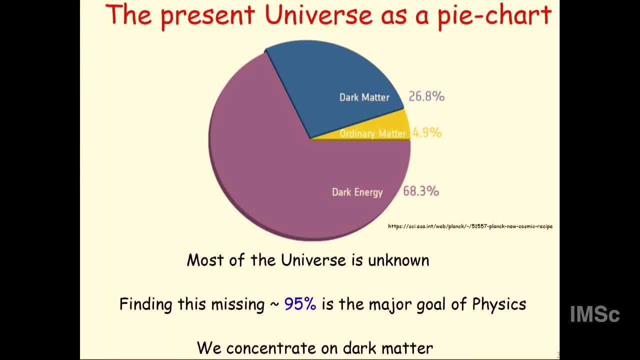 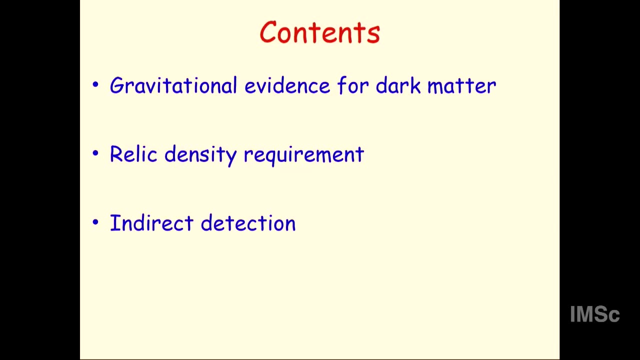 human beings have been existing for a long time. so finding this missing 95 percent, all right, this dark matter plus dark energy is one of the major goals of physics. all right, in this talk, as you already noticed, i'll be talking about dark matter. okay, so so i will first give you gravitational evidences for dark matter all. 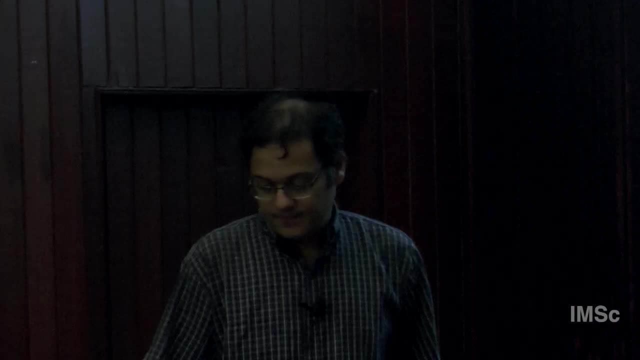 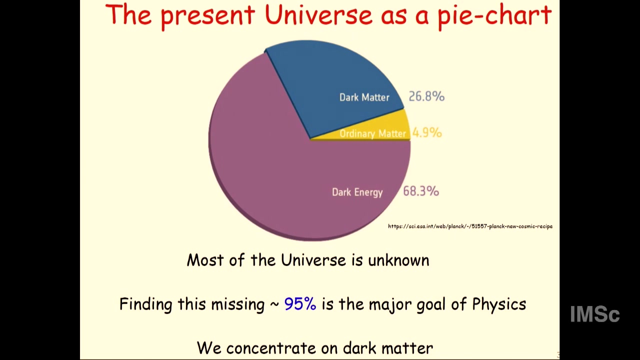 right. there are numerous evidences. i'll just concentrate on two of them. okay, then i'll talk about the relic density requirement. what does that mean? that means, i mean, how do you get this number? all right, this number, as i said, is known extremely precisely, to one percent accuracy. how? 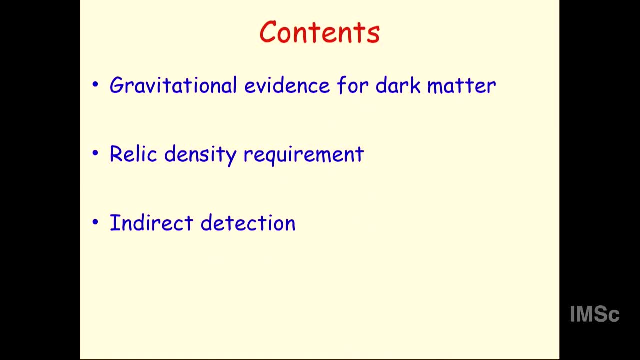 do you get it right? i'll tell you one example of how you get it, and then i tell you one way to answer the question. what is dark matter? all right, we know that it exists, but if you ask a very basic question, what is dark matter? what is this made up of? right, this laptop is made up of electrons, protons, things. 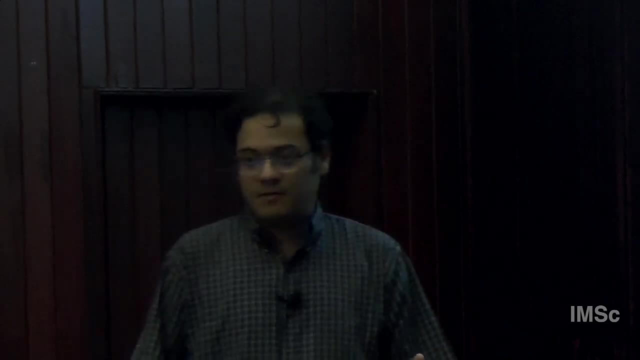 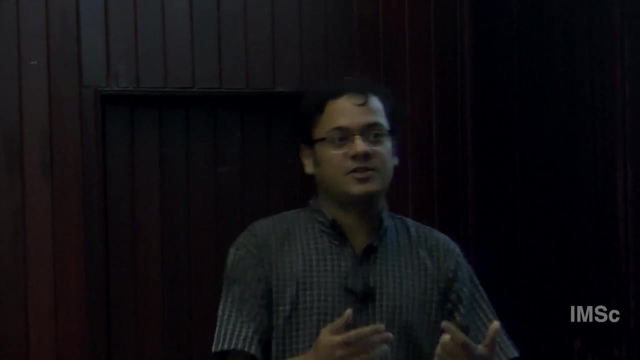 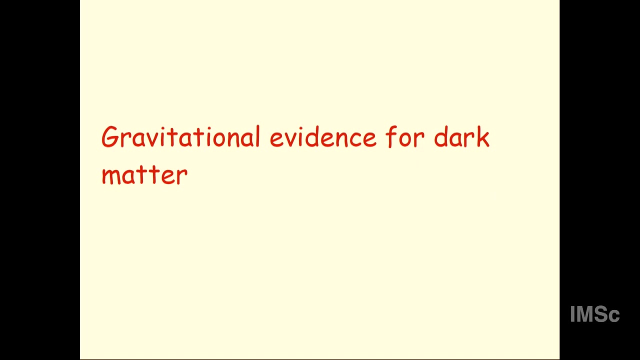 like that. right, so you can ask a very similar question: what is dark matter made up of? we have literally no idea. all right, indirect direction, as i will uh tell you, is one way to answer that question. all right, okay, so let's first talk about gravitational evidences for dark matter. this would be evidences: 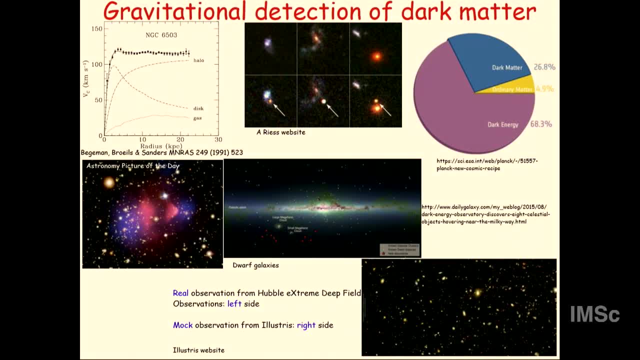 by the way, not evidence, okay, so this is a very busy slide. all right, i intentionally made it very busy, simply to show that there are many evidences for dark matter at various length scales, and two of them i'll explain in some detail. the remaining i'll not explain in detail. 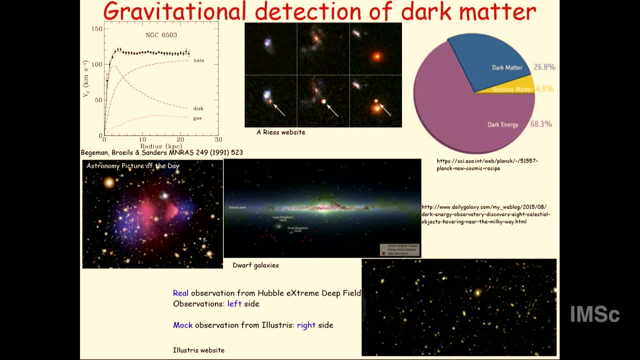 all right, but feel free to ask questions. so this plot, this is the rotation curve of this galaxy, ngc 6503, some, some name of some galaxy, right? what is plotted on the x axis is the radius, is the distance from the center of the galaxy, Its. 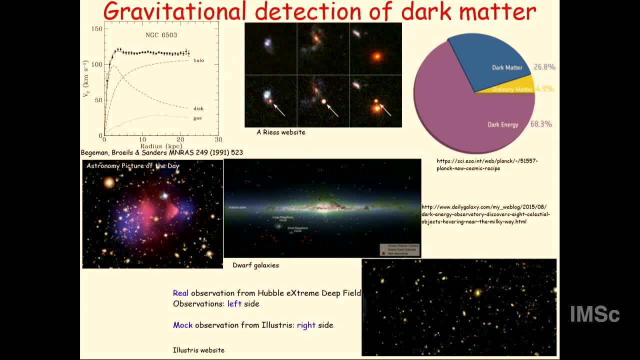 units are kilo parsec. One parsec is three light years, If you forget that three this is like thousand light years roughly, And this is circular velocity. So that means we see stars and gas in that galaxy moving around and you measure the velocity You can. 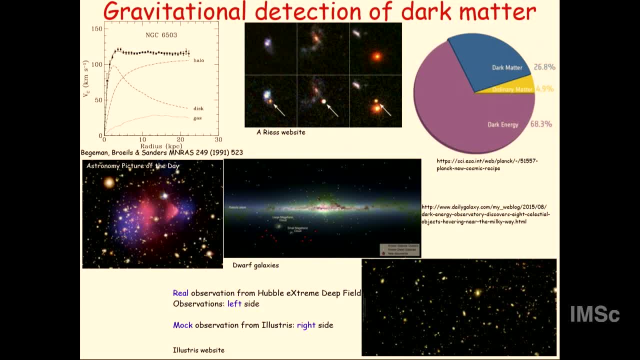 measure that. You see this data. This is the data And I will explain this in some details. I will just skip this. But the point is this is an evidence of dark matter. at scales of, say, tens of kilo parsec, Again, that means 10,000 light years, roughly up to a factor. 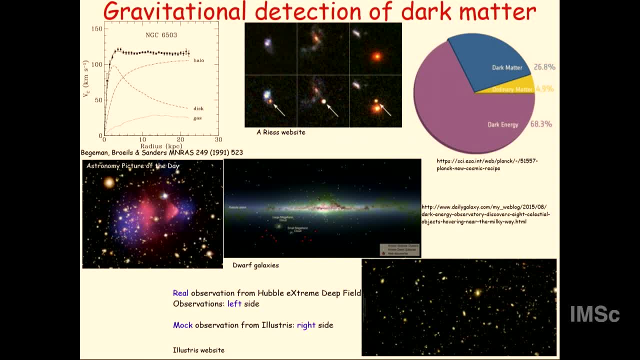 of three. So that means if you do astrophysical observations at the scale of 10,000 light years roughly, you need dark matter. In fact, even at smaller length scales you would need dark matter. But this is just from this you can get, at least whenever you make astrophysical. 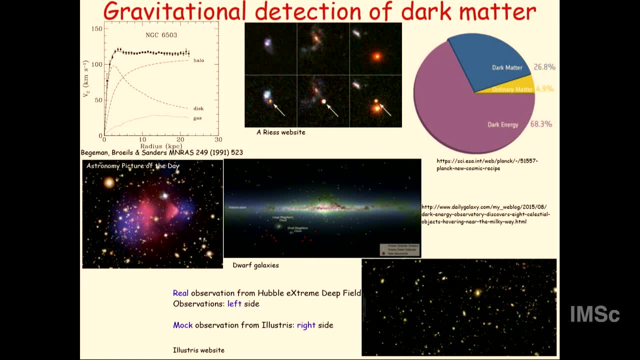 observations at the scale of, say, 1 kilo parsec or more. you need dark matter: 1,000 light years or more roughly. You mean beyond this. That is a great question. Good, So turns out that this is an evidence of dark matter, This halo thing that you see. I will explain. 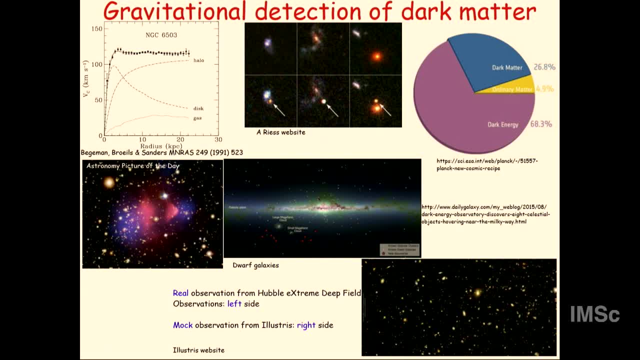 in the next slide is an evidence of dark matter. We do not know where it falls off. We have never seen the rotation curve, but it has to fall off because that is the finite. This is basically remember. Vc is square root of this circular velocity standard thing. 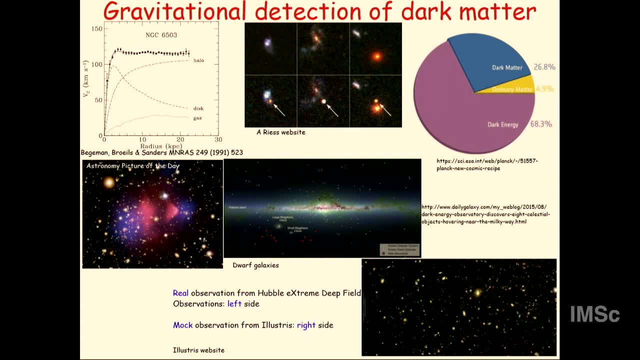 So it depends on the mass. So we know it should fall off. We do not know where it falls off, simply because there are not enough tracers. I mean, how do we measure this? We measure this by looking at stars and gas moving around it. There are not enough stars and gas away. 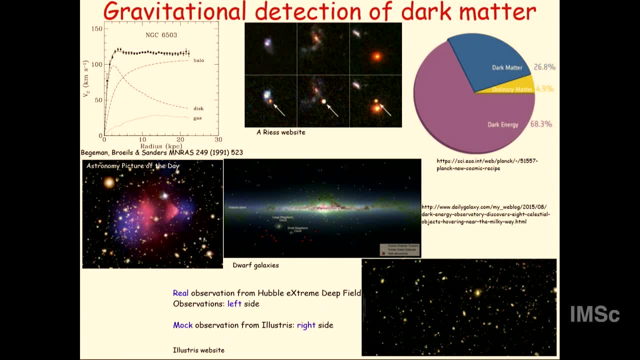 So that is why we do not know. So the maximum we know is that it is up to. it is up to say, roughly 20, 30 kilo parsec, But the dark matter halo should extend to up to 100 kilo parsec, 100 or 200 kilo parsec. 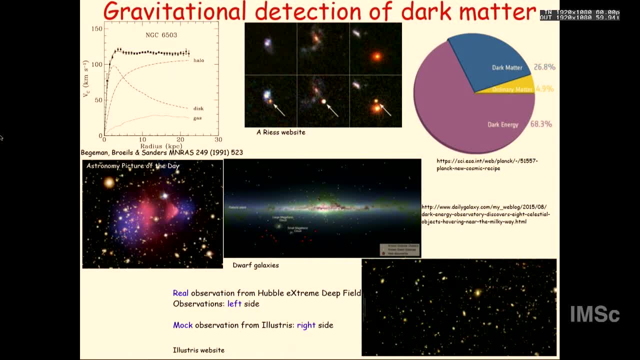 for individual galaxy, But the precise number we do not know, but that we know from simulations. There are various ways to find it. In fact, beyond this, I mean, there are not much mass there and you can figure out some other things. Good, So this is one proof. The second proof: 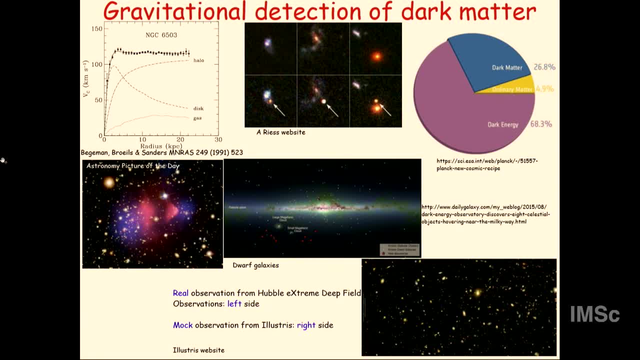 which I will go over in some detail, is this: This is bullet cluster. I will tell you in more details what that is. Basically, what you see is two clusters. What are clusters? Clusters are 1,000 galaxies roughly bound together like they are gravitationally bound. 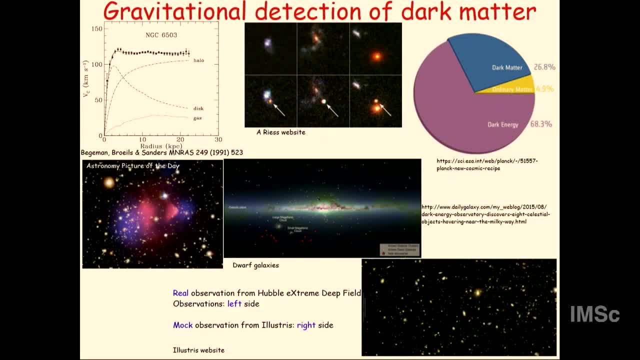 They collide, and I will show you in some of the next slides where you see that most of the mass is actually not in what we see, what we can observe electromagnetically. This is not the only merging cluster that we know of. As far as I know, there are roughly 70. 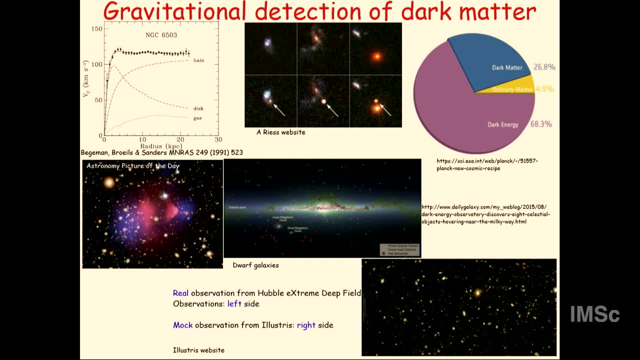 merging clusters In all of them. if you do the analysis, you find that you need extra matter. Good, So this is evidence of dark matter, Thank you. Dark matter at the scale of mega parsecs: 10 power, 6 parsecs, Let us go here. So this: 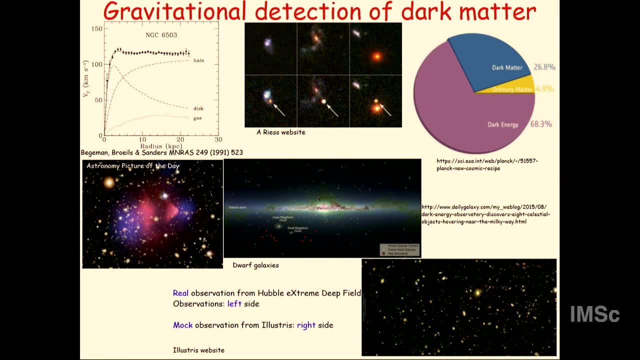 is from this website where, basically, we look at supernova 1A. So supernova 1A is one type of supernova. You do not need to know the details, but the thing that you need to know is that the luminosity, or in other words, the light coming out from the supernova, that 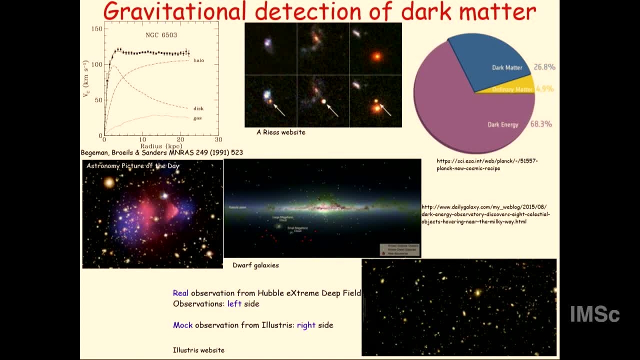 supernova. that class of supernova can be standardized in the sense that you can say what is the intrinsic luminosity. You can do that And this is actually what you gave Adam Ries this work gave Adam Ries the Nobel Prize right, So it is very difficult work. 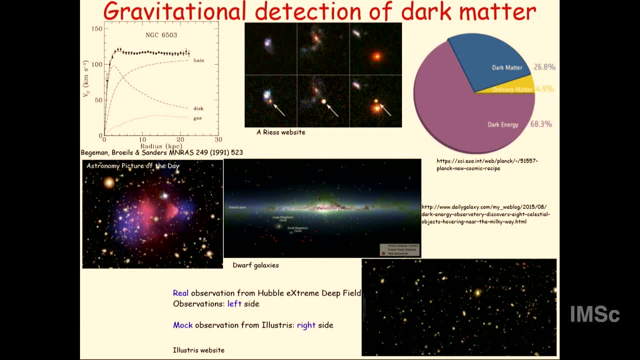 but you can do it. Using this, you can show that there is dark matter at even larger length scales than this. This is ten-th of kilo parsec. this is mega parsec. this tells you even hundreds of mega parsec or even more even, giga parsec. This is an artist impression of our Milky Way galaxy. 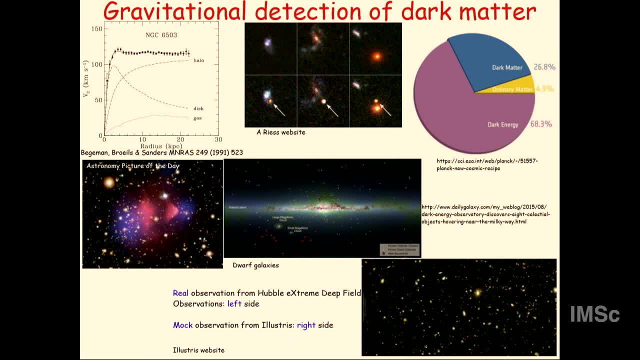 from the side. Suppose you went out of the Milky Way. you took a picture. This is how it will look like. So this is the galactic center, this is the galactic bulge, this is the galactic disk. So there is a disk and there is a bulge like a ball, And all these. 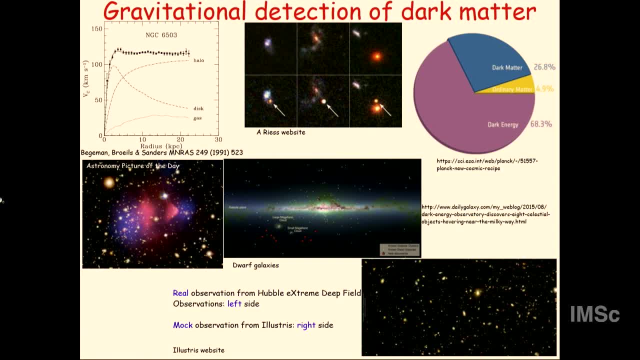 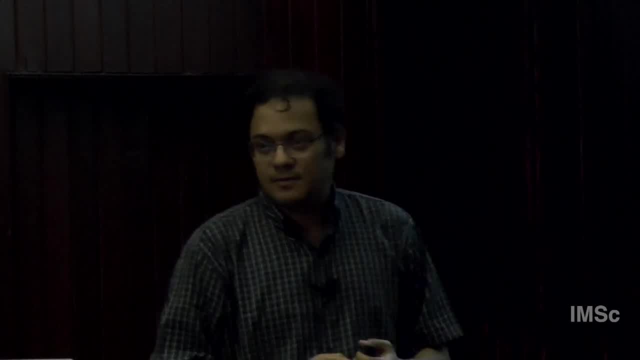 lights that you see. some of these lights are Milky Way satellites. That means Milky Way is a big galaxy. Around the Milky Way there are satellite galaxies, small galaxies with masses less than factor of 10 or more smaller than the Milky Way. They move around. 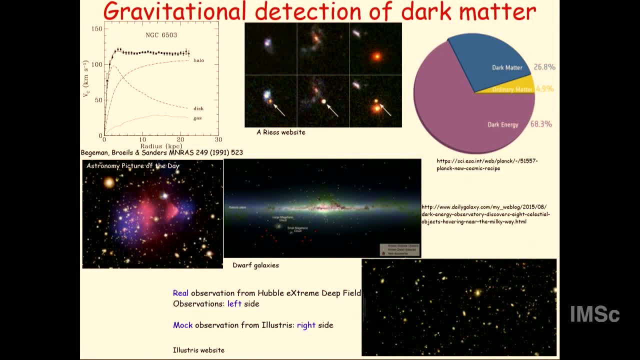 the Milky Way. So these galaxies move around, these large Magellanic clouds, small Magellanic clouds, and there are other ones. These are two of the massive satellites. They move around the Milky Way. In order to properly account for their motion, you need dark matter around. 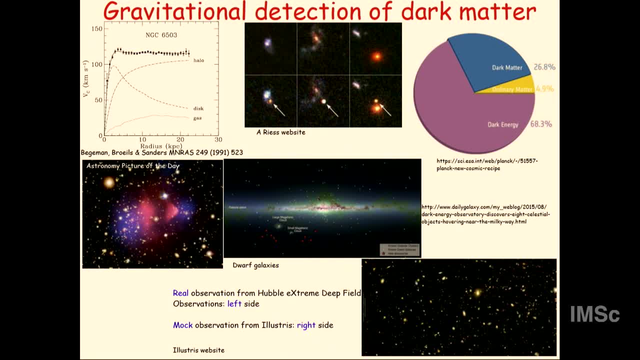 this. So this is a proof of dark matter at hundreds of kiloparsec. What is the size of those galaxies? Which one? Oh, LMC, LMC and SMC. these are roughly factor of 10 smaller than the Milky. 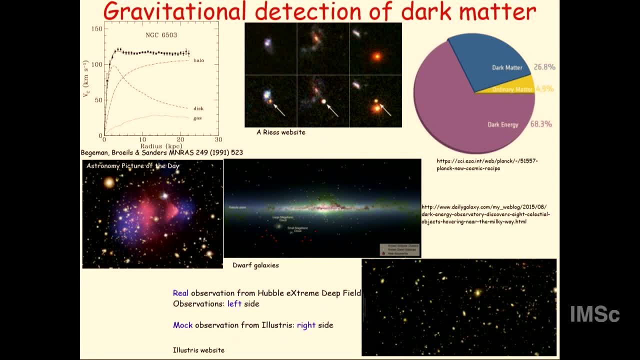 Way in mass. So Milky Way has a mass of roughly 10 power, 12 solar mass. We know that number very well within a factor of 2, by the way, These are 10 power 11.. Large is large, small is small. So they are: 10 power, 11 solar mass, slightly less, something like. 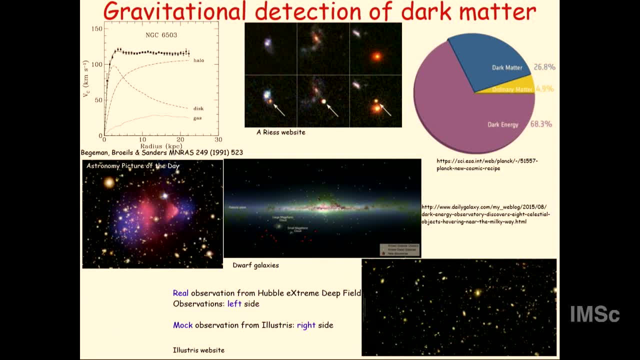 that And the size is probably factor of few smaller than the Milky Way. How much is the mass of parsecs? Parsecs, Okay, good. So the Milky Way dark matter, halo, right. So you have to first ask the question: is size of what? Size of what we see, baryonic disk, or size of the dark? 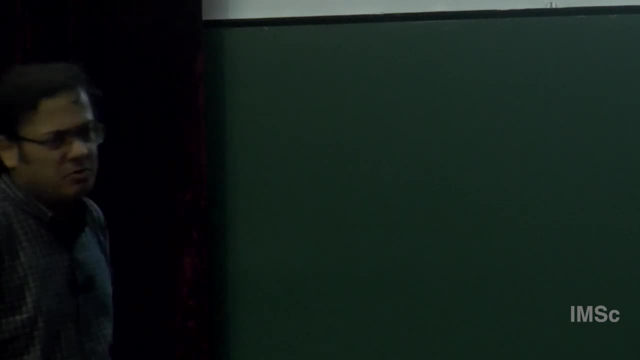 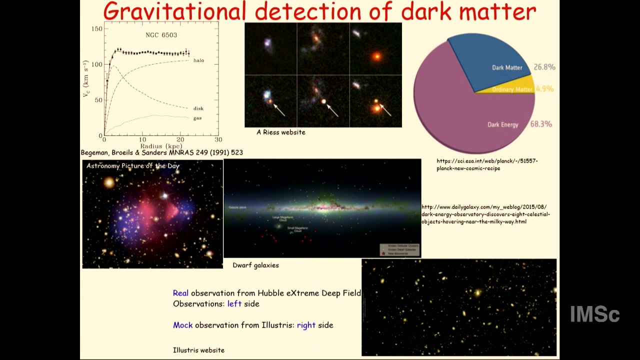 matter halo. So the size of the dark matter halo of the Milky Way is roughly 100, 200 kiloparsecs. The size of these guys dark matter halo will be roughly few tens of kiloparsecs. That's the thing. Okay, good. So this, as I said, is the CMB. All right, so you measure. 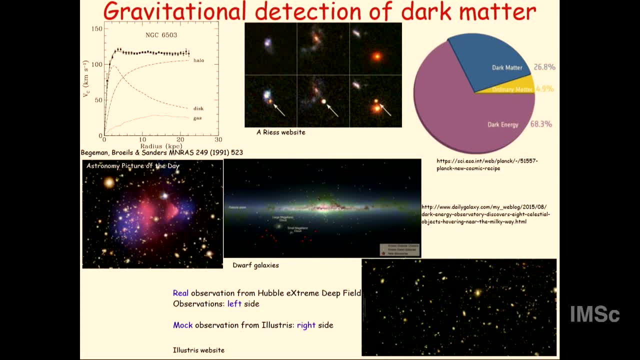 the universe, the cosmic microwave background and this you see, the evidence of dark matter. This is the evidence of dark matter at gigaparsec length scales, 10 power, 9 parsec length scales And finally, I mean all of this is observations, right Suppose. 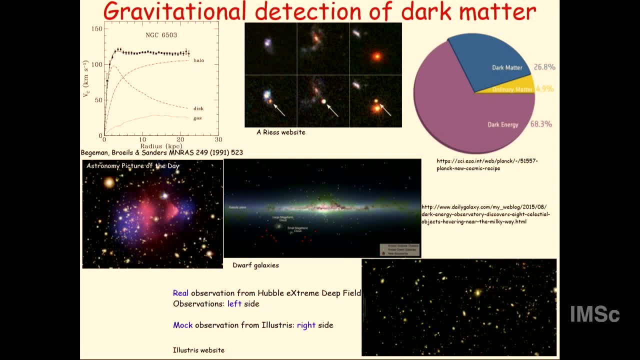 you're a theorist, right, And you say: well, wait a minute, I want to theoretically find if there is dark matter or not. You can actually even do that. You can try to simulate the whole universe. There are simulations which you can run on a laptop- standard laptop. You download it and you can. 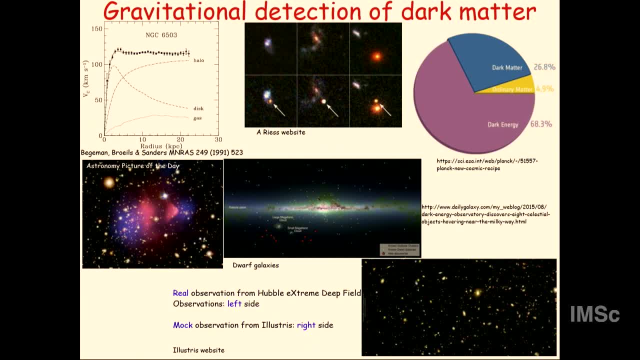 run it, And you can only match the observations of the universe if you have something like dark matter, right, Something like a pressureless fluid. In simulations you think of dark matter as a pressureless fluid. So this is a more fancy simulation which you cannot run in your 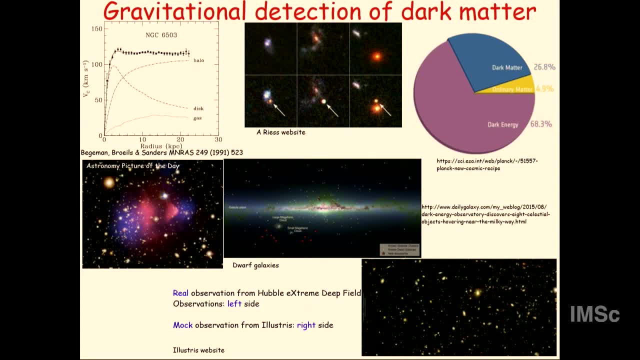 laptop, all right, This is from the illustration collaboration. So in simulations there are many people. They make a collaboration, They run simulations in big collaborations. So the left side is a real observation, all right in this picture. Left side is a real observation from the Hubble. 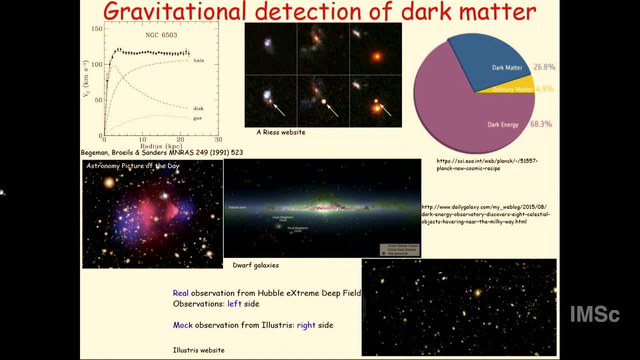 extreme deep field right. So from the Hubble telescope there's some observation. all right, The right side is a mock simulation, right? If I just give you this picture, right, you could say, well, okay, this is just part of a sky, right? You can obviously do this not. 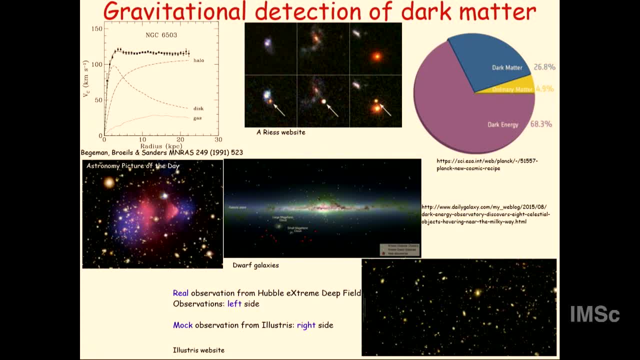 just pictures. You can do this. You can make this picture. You can do this. You can make this picture. You can measure many properties statistically. How many galaxies are there per unit mass? How many? what are the colors of the galaxy? That means, what is the luminosity? 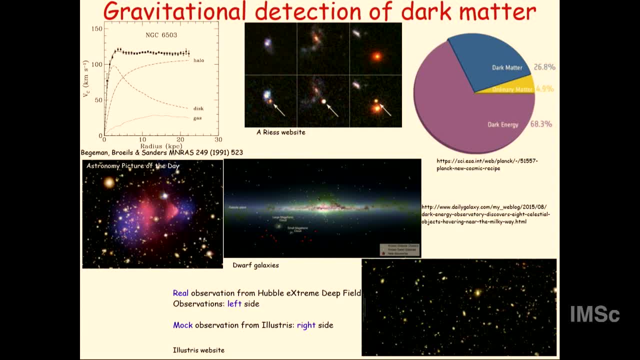 of the galaxies And various things. How many black holes are there in the big black holes are there in the universe? You can do measure all of these things and they do match extremely well. So this is a proof that you need dark matter which acts as a pressureless fluid. 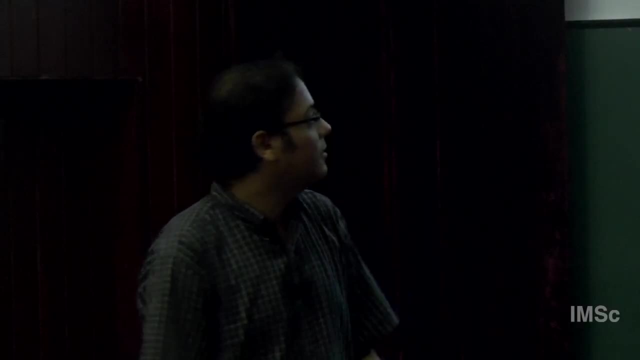 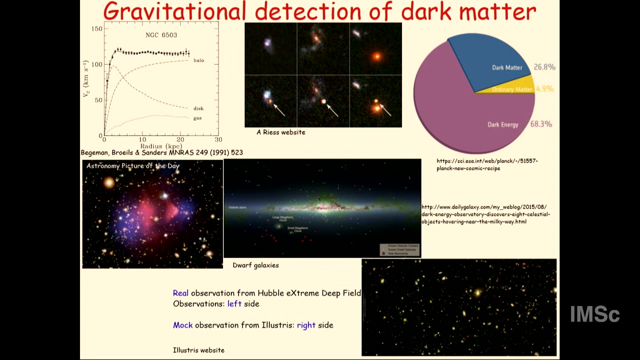 in the universe in order to reproduce the observations. all right, Now let me go to the next slide. Yes, yes, yeah, sure, Yeah, no, I'll answer it. Good, I'll give. tell a point about it. Good, just wait, I'll tell a point slightly after. 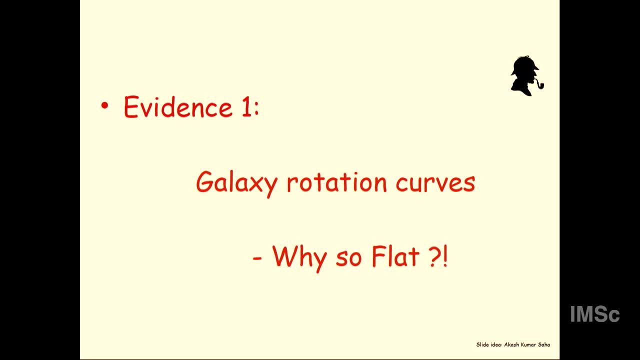 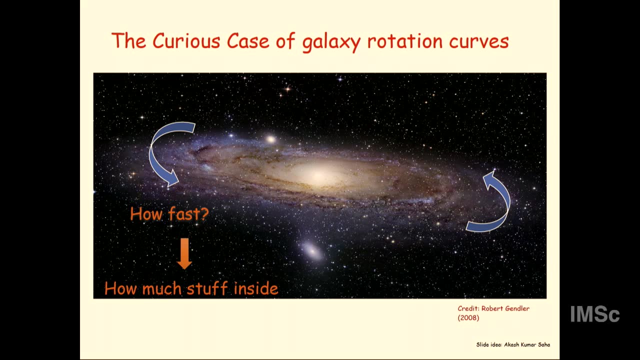 this thing, Not this next slide, but in a few few slides. So let me talk about the first evidence, galaxy rotation curve, in some detail. all right, So this is again an artist side view of a galaxy. all right, So you can see, this is the bulge, this is galactic center. 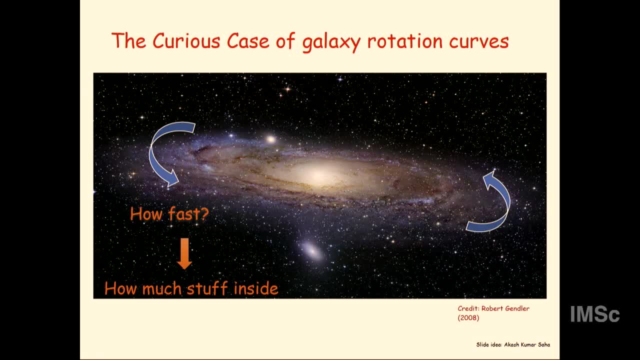 this is the bulge. this is the spiral arms. all right, So if you go out of the Milky Way, take a picture. it'll look like this: How fast it rotates depends on how much stuff it is inside. pure Newton's law, all right. 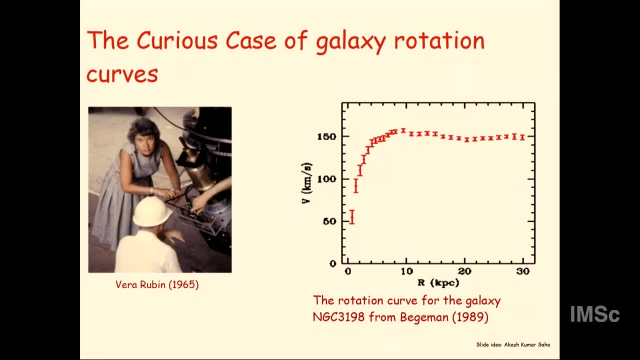 And then I'll come to the question later. I'll come to that. So this is actually. we should first credit, give credit to Vera Rubin, who actually did all of these pioneering measurements, and there's a beautiful story behind it. I mean, why was she looking here in the sky? 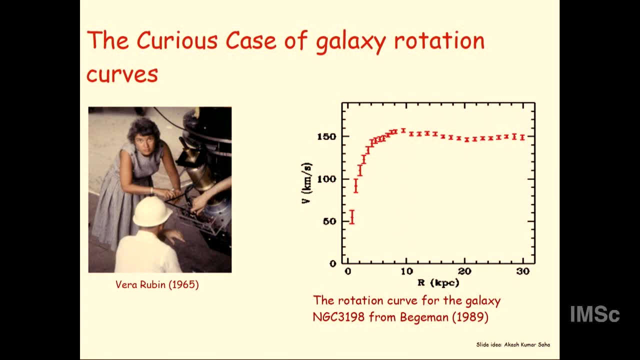 right, Because at that point when she was doing it, all the interest, interesting stuff in the galaxy was near galactic center, right? You see? this is again velocity radius in kiloparsec. Every galactic center is somewhere here. 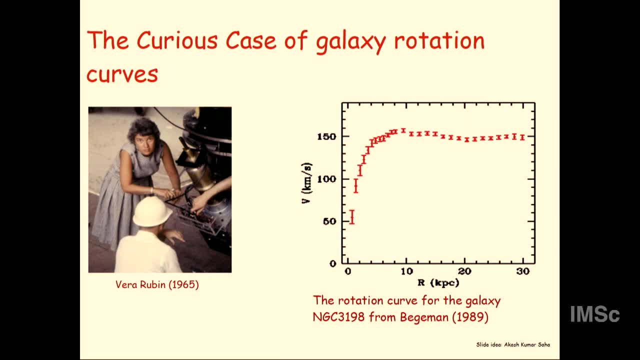 She was looking here. Why? Well, the story goes that she was a young astronomer and nobody gave her time in the telescope to look here. They said, oh okay, you look here, there's nothing interesting, you just have a look, that's it. And she had a look and after some 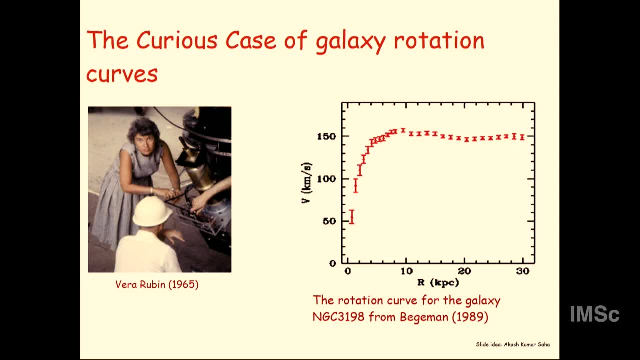 painstaking effort, she actually found more than what is there in the galaxy. here She found more interesting stuff. This is a very beautiful story of Vera Rubin how she actually discovered dark matter from basically grand projections. Her telescope times were rejected, that's why she looked here. right? This is actually the story. 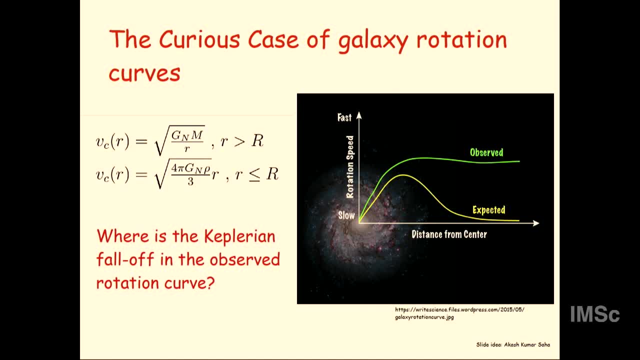 Subtitles by the Amaraorg community. Okay, good, So let's do this So you can plot this again: distance from the center, rotation speed, This is say the picture of some galaxy. If you take, I mean you can do. 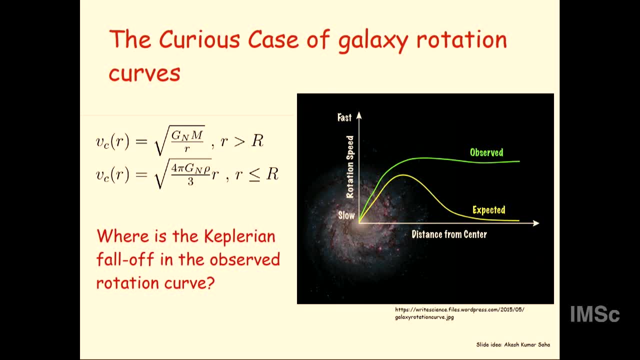 this standard Newtonian mechanics. alright, If you are outside the mass, you have this formula: this should fall off, and if you're inside it, it should be sort of stable, alright. So if you just follow the mass, as if the mass is following the light, then your curve. 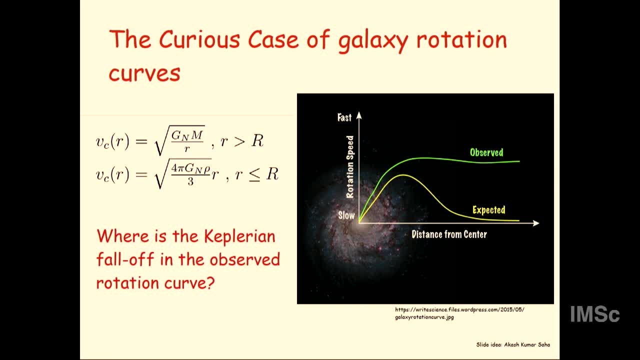 will be like this. This is expected, alright, But what we see is this: observed alright, And there's no light here. You can say wait, wait, wait. Why don't we use better telescopes? We have been doing this for last five decades and we know even from other observations that 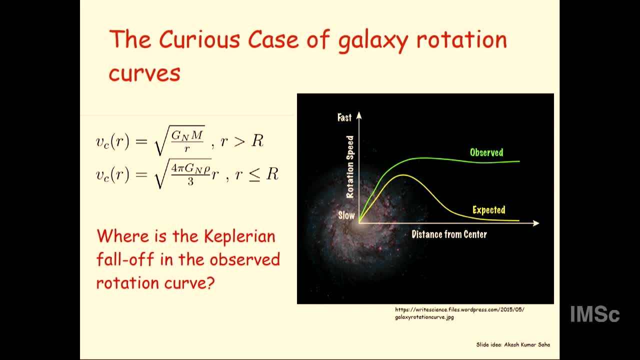 it's not that there are faint stars here. There is literally something new. alright, Faint stars cannot do it, okay, So this is some explanation of it, and then you can do this thing in fancy. GR language Subtitles by the Amaraorg community. 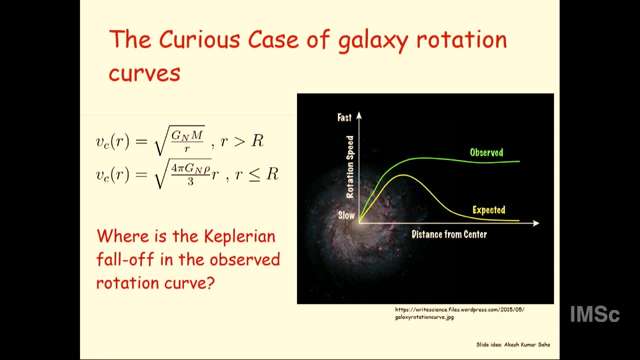 It actually don't require GR, but you can still do it. It still has the same thing. You cannot explain this observation with this thing. There's no way to explain it, alright, Good, So this is a very simple example of galaxy rotation curves. People have done this. 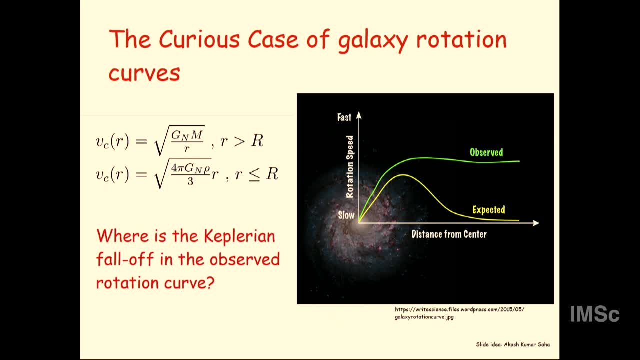 for various galaxies. by the way, I just gave examples of one or two. There are people who do this for their whole life, alright, They take various galaxies and try to figure this out, this rotation curve. These are very difficult measurements and they find it for every single. 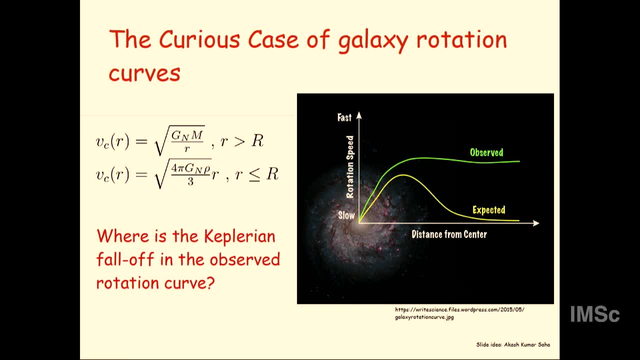 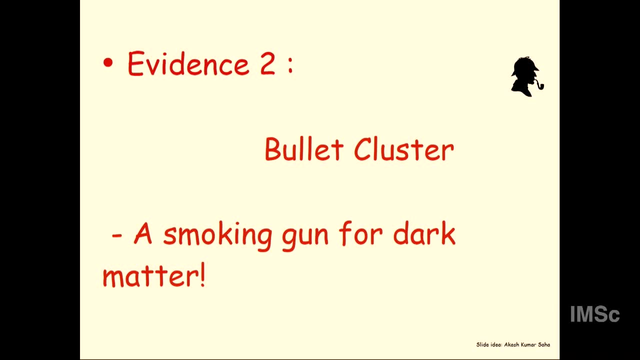 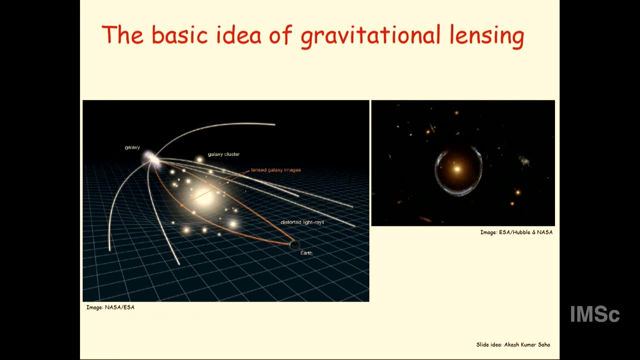 galaxy, Every galaxy requires dark matter, alright, Okay, good, Let me talk about the evidence in the second thing. This is bullet cluster, alright. So before this, we need to talk about something called gravitational lensing. This is one slide on gravitational. 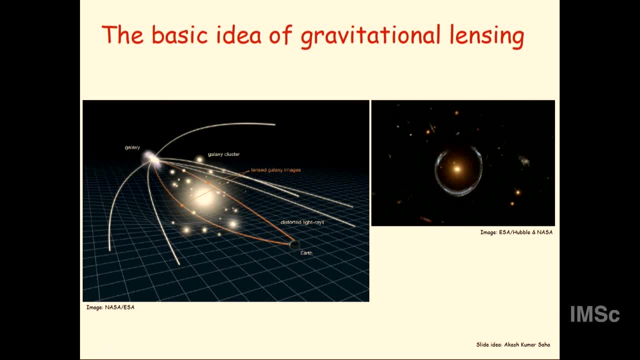 lensing. What does it show? So you must have heard that gravity bends space and light follows that bent space. alright, This is in very simple terms. This is gravitational lensing. So the story is as follows: This is the observer Earth, This is some distant galaxy and suppose 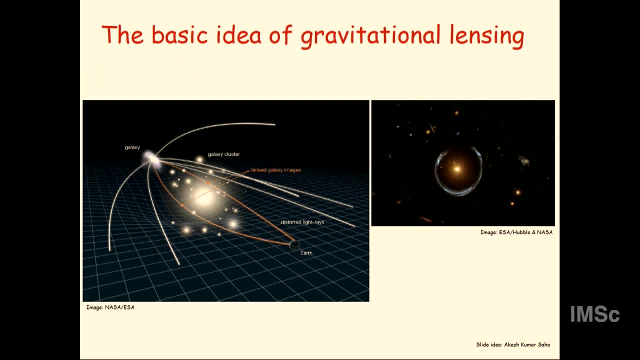 there is something in front of you which you cannot observe, or which you can observe alright. Because of the gravity of this object, the light from this galaxy will get bent. They will not come straight towards us, They will come bent towards us. This is called galaxy. 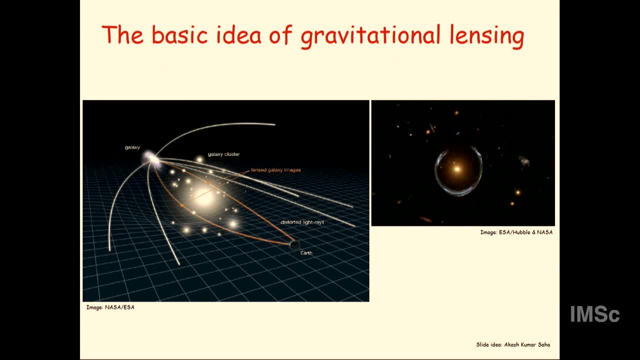 lensing alright. So the light is lensed. These photons should not come towards us because they are going away, and then you lens it towards the Earth. That's lensing, alright. This is again routinely observed by astronomers and cosmologists. 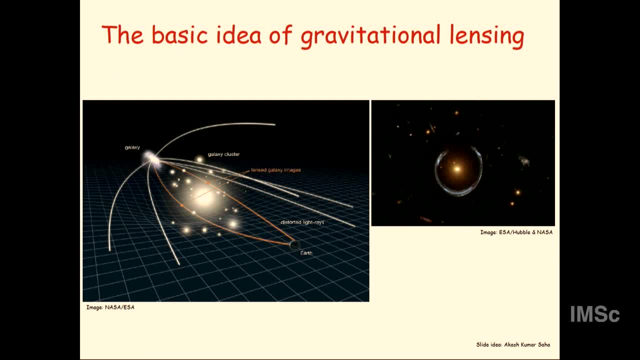 Alright, This is a real picture, right Where basically a galaxy is lensed and you see this thing. Basically, this is picture of all the galaxies that's actually formed. alright, So basically, again, just think of this as optics sort of. I mean you, this light goes. 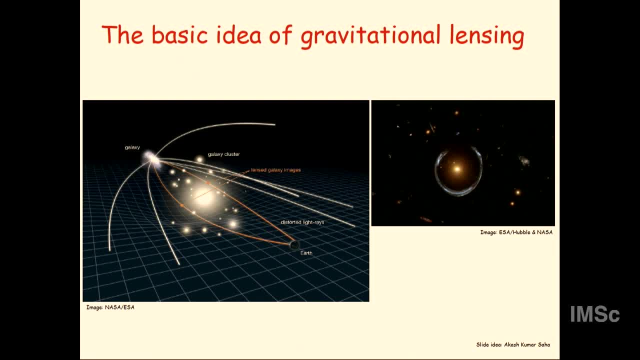 away. So this picture will be here, This light. you just go There is a picture here and like: this will happen, alright, And this tells you that there is definitely some mass, even if it's invisible in front of it. okay, And this is actually done in many, many galaxies. 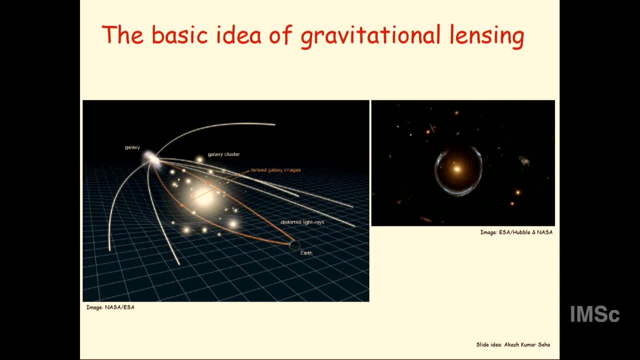 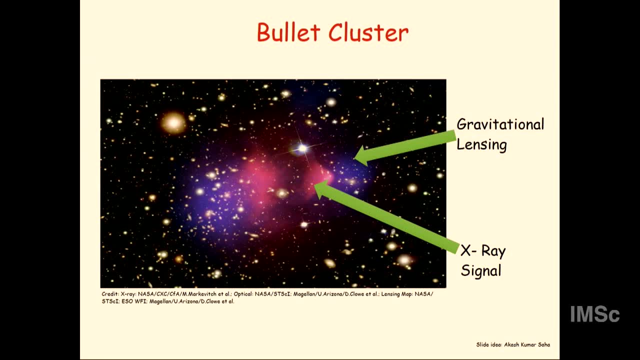 galaxy clusters And we again see that we need dark matter. alright, So what is it done? How is it done for bullet cluster? So, as I said, a cluster is 1,000 galaxies bound together roughly of the order of 1,000 galaxies. So what do galaxies have? So, galaxies have stars, Stars. 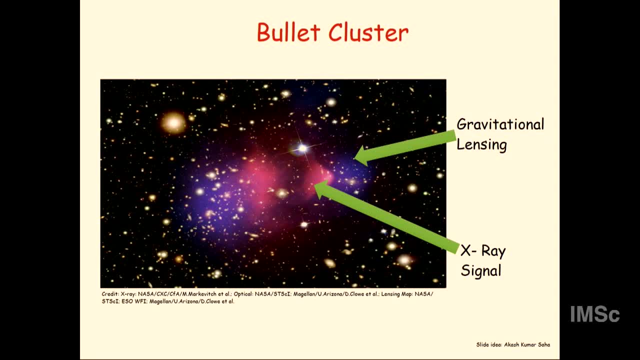 will not collide among themselves. Why? Because stars have too much distance between them. Stars will just go through them. That's it. It has gas. Gas means diffuse whatever material in the galaxy That will collide because of electromagnetic interactions. alright, So. 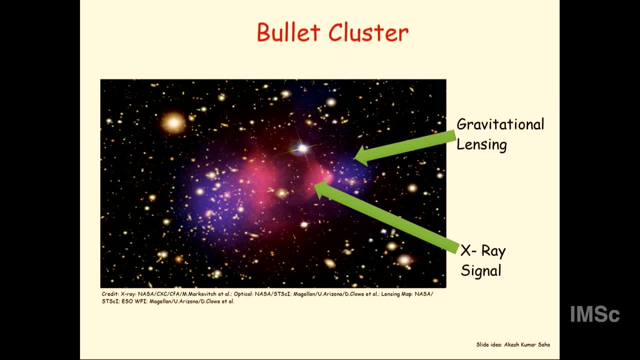 in this picture. what is shown in these pink things is basically gas which have collided- alright, And it's giving out some X-ray emission- alright. There's this bullet-like structure- That's why it's called a bullet cluster- And they're giving this X-ray-like emission, alright. 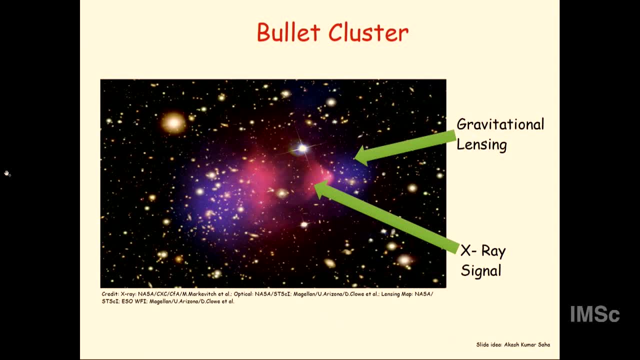 From this emission. you can figure out what is the mass of the gas. here You can figure this out, alright, And you can also do something else If galaxies have, or if galaxies have some mass of the gas. here you can figure this out, alright, And you can also do something. 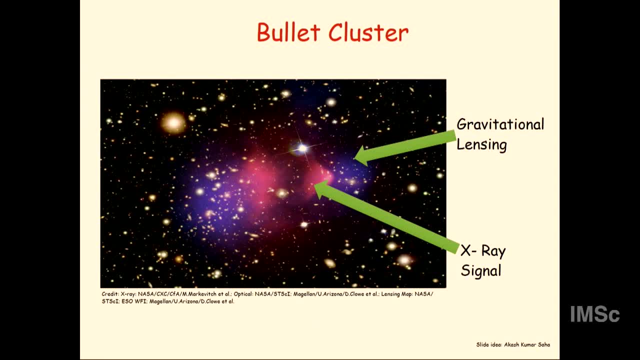 else. So you can see that these bullet clusters have dark matter. Dark matter will just pass straight through. They will not interact with matter And you can try to lens the material in these regions. Remember these things have actually have had sort of friction. They 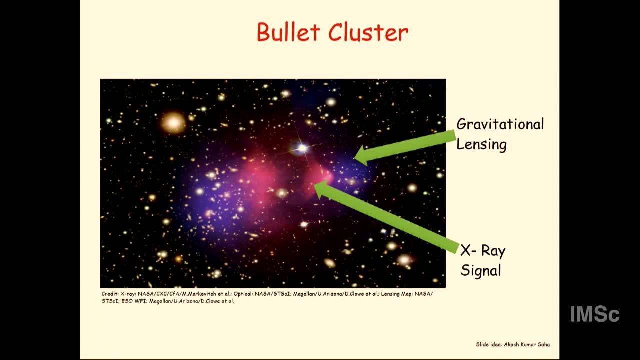 have stopped, whereas dark matter has just gone through. alright, You can lens the background galaxies, right? So these galaxies that you see are actually behind this bullet cluster, You can lens them and you can find that they have to be lensed. alright, Because, again, 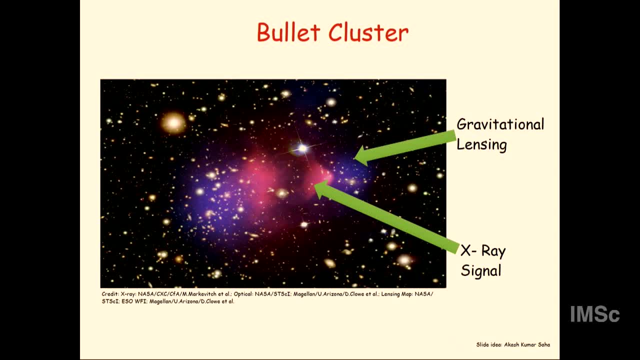 you can do galaxy shapes. Lensing changes the shapes. alright, There are various techniques to do it. You can find that the mass in this blue region is actually five times the mass in this pink region. That tells you that there is dark matter in galaxy clusters. alright, There's no other way you 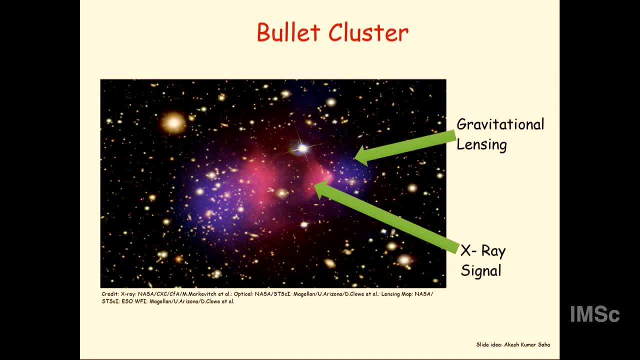 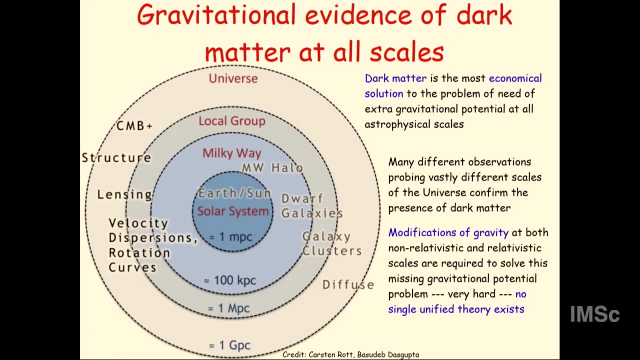 can reproduce this signal. alright, Is this clear? Okay, let's come to the part of the question that's actually not mentioned. So what I've been trying to tell you and convince you is that if you make gravitational and cosmological observations at all scales of the universe beyond, say, one kilo parsec, that is again. 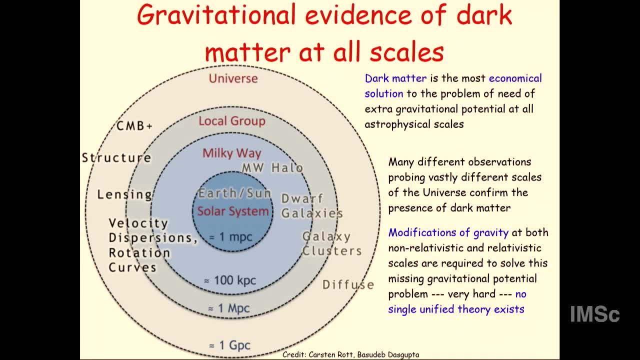 thousand light years, you need dark matter. In other words, if you do not include this extra non-interacting matter, you will not fit the observations. The observations need something right. So this is various scales, So you can do the largest scales, scales: 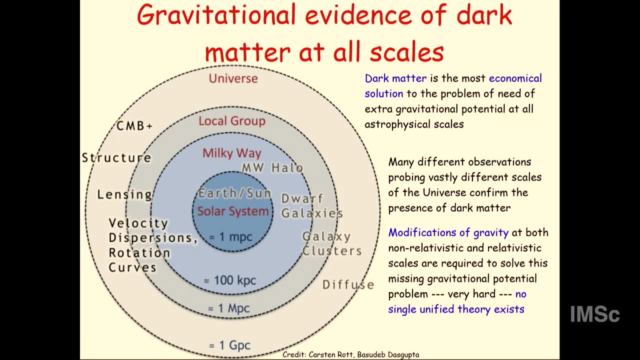 of CMB structure, formation, lensing and this rotation curves and various different things. alright, And then let's come to the question. All of this I said, well, it assumes GR, it assumes Newton's gravity and things like that. And you can ask: wait a minute, why are you assuming? 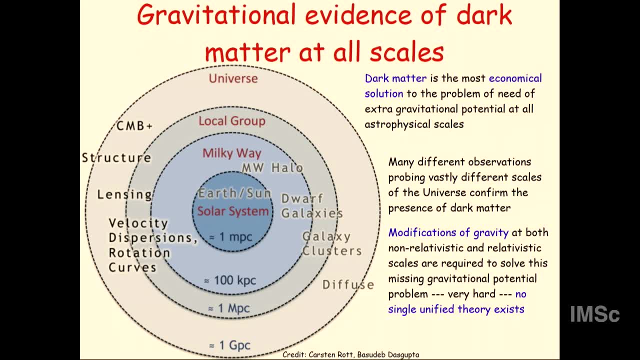 Newton's constant, Newton's laws of gravity and GR. Why can't you modify gravity? So that's a good path to take, except that none of the modifications of gravity have been able to reproduce these observations at all scales. I mean, most of them actually can. 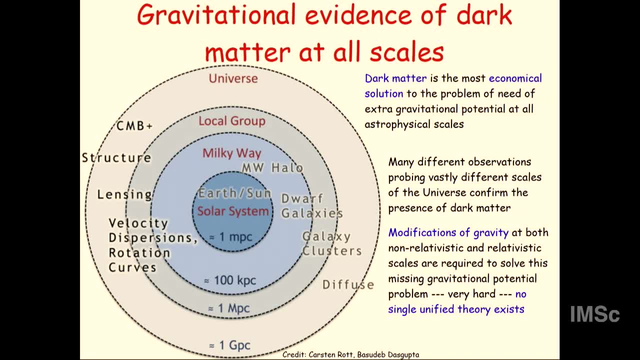 do it very well at the galactic scales, Beyond them, they just do not work. So the way I take it, I look at it this way, So the way I think of this, is that if you make observations, there are problems in these. 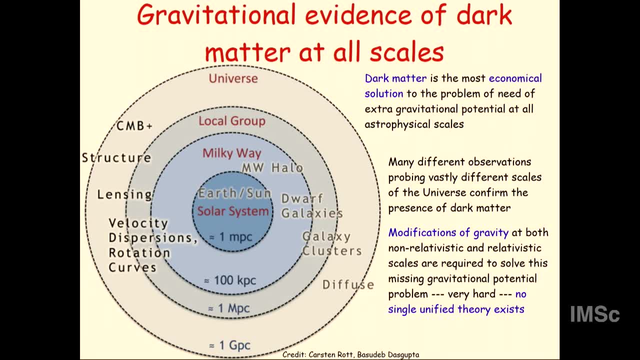 observations. We cannot explain it. In order to explain it, dark matter is the most economical solution. You put dark matter. problems from all scales, from galactic scales to extra galactic scales, will get solved. One solution will solve everything. If you do modified. 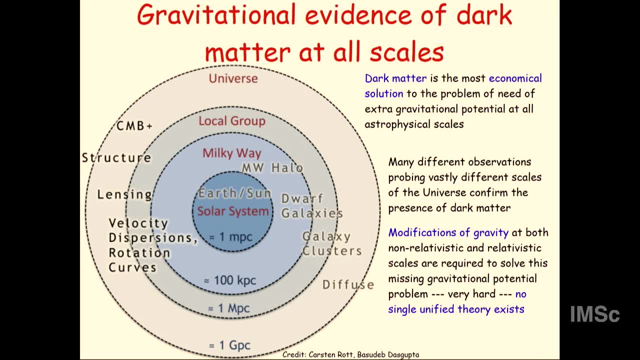 gravity. it may work, But currently we have not been able to show that it has worked, So it will require. I mean, there is no single, unified modified gravity theory which will solve all these problems. So the way I think of this is: there are. 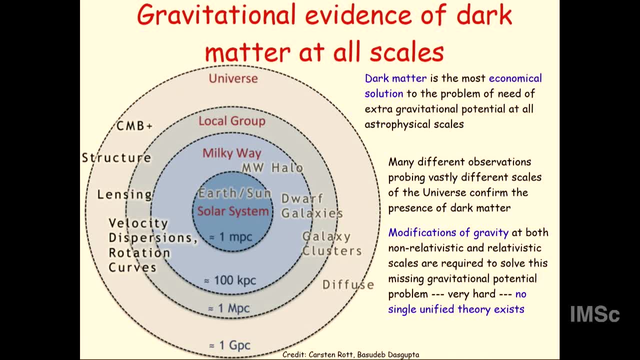 again, as I said, it is an economical solution to it. Maybe nature is even more complicated, Maybe part of it is modified gravity, part of it is dark matter and things like that. But again, that we can only find by doing these observations and trying to answer these. 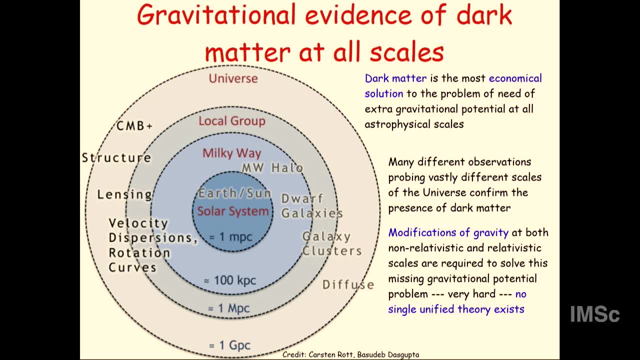 questions. Does that answer the question? Yes, Okay, Thanks. There is still doubt about whether modified theory cannot explain. I think at the CMB scales they literally cannot explain. This is, I think, almost everybody agrees. Okay, They explain that they effectively introduce a particle sort of. So this is almost everybody. 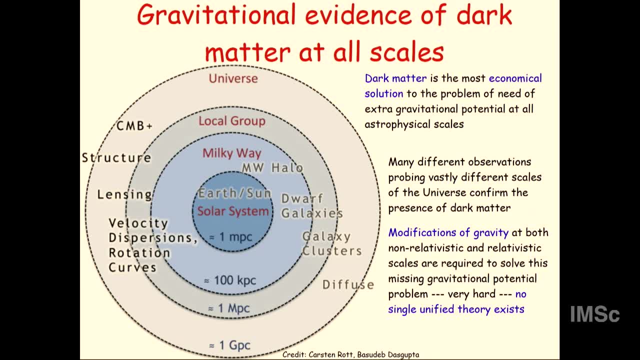 agrees with, Like all these tables, gravity and all these things. this I think everybody will agree, Put it this way. But I do agree at galactic scales, MOND. so this is one of the modified Newtonian dynamics. modified gravity works extremely well, Actually, we. 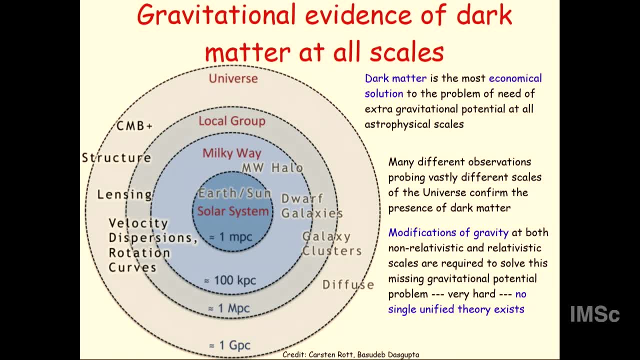 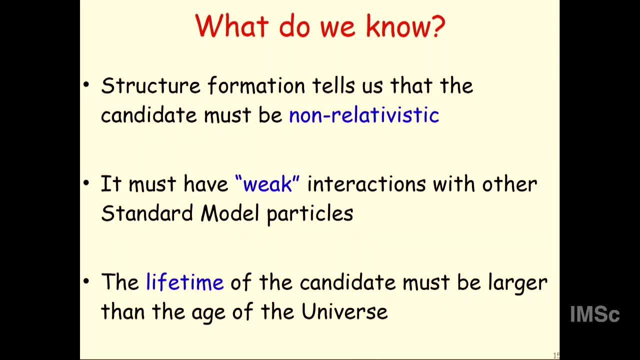 do not know why it works so well. That is also a puzzle, but I can talk later if you are interested. Okay, good, So what do we know? So, given all these observations that we have been doing, Yes, For the last few decades, 50 years- we know quite a few things about dark matter. 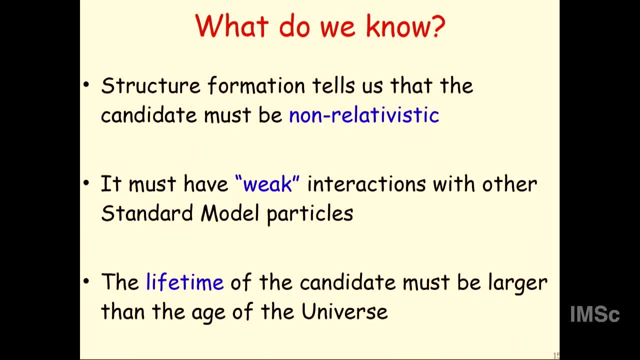 All right. The first thing we know is that the dark matter candidate has to be non-relativistic, All right, Otherwise structure formation will go crazy, and I will show you a picture how it will go crazy. The second thing we know: it must have weak interactions with. 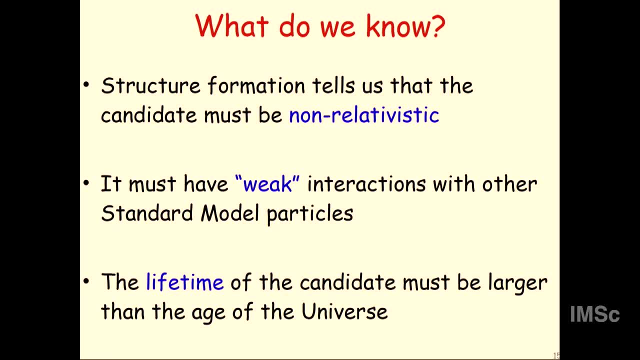 standard model particles Here. weak does not mean the four forces weak, that kind of weak, It can be that weak also- but it also means it cannot interact very strongly with known matter, Otherwise again, observations will go crazy, completely wrong. That is something. 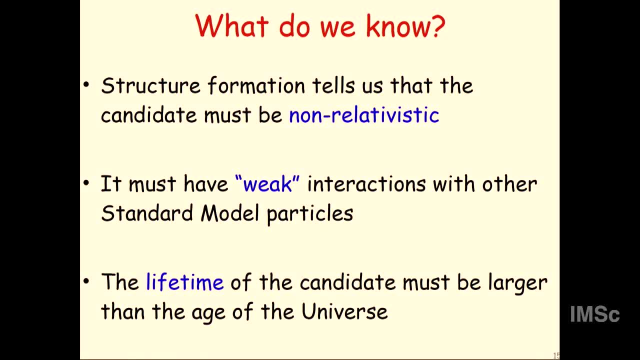 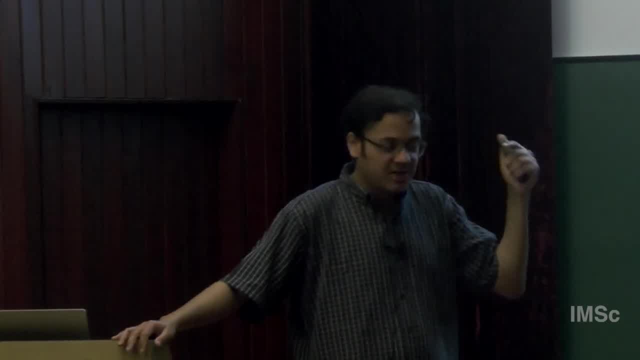 we know, And we also know that the lifetime of this dark matter candidate must be greater than the age of the universe. Why? Because we see dark matter very close to us. So that means whatever is dark matter must be existing till that time, this time. So these are the 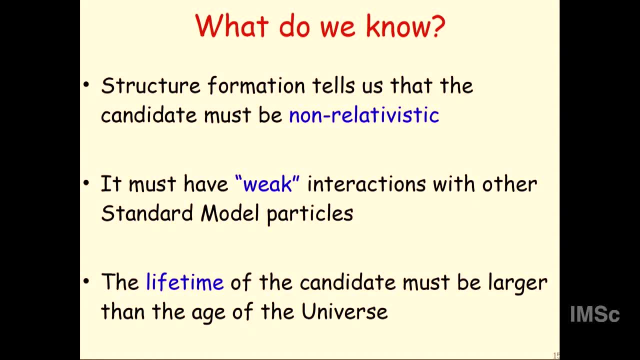 three things we know. All right, Note that all of these things are actually not equalities. We just know these are inequalities. Right? For example, we know that the lifetime of the candidate must be larger than the age of the universe. But what? What is it equal to? 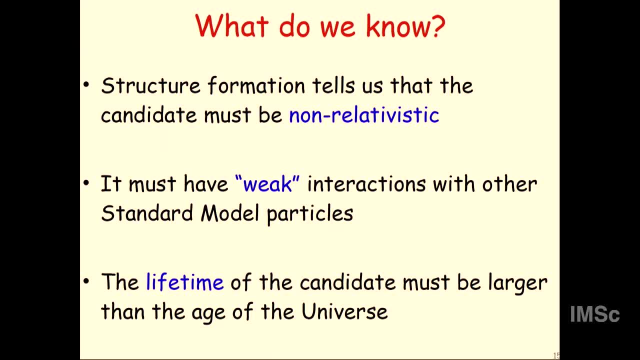 Yes, We do not know What is it equal to? We do not know, We just know it is a greater than some number, Right? No Ultralight dark matter can be a good dark matter candidate. I am not ruling it out. 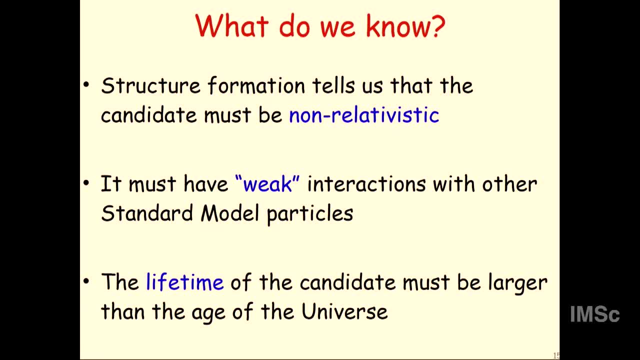 Good, So non-relativistic. if it is ultralight dark matter, it has to be. it has to form in a non-thermal way, such that its momentum distribution is actually non is momentum, such that its momentum distribution is non-thermal. For example, people talk of axions which can 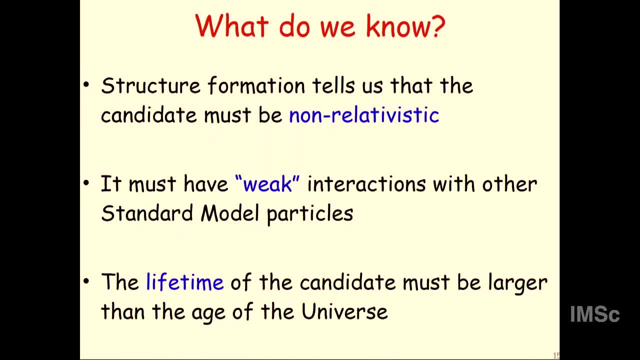 be as light as micro eV, That is a great dark matter candidate. Yes, Because it is not formed in a thermal way. All right, So I will tell you what is the mass range of dark matter. But ultralight particles can also be dark matter. There is. 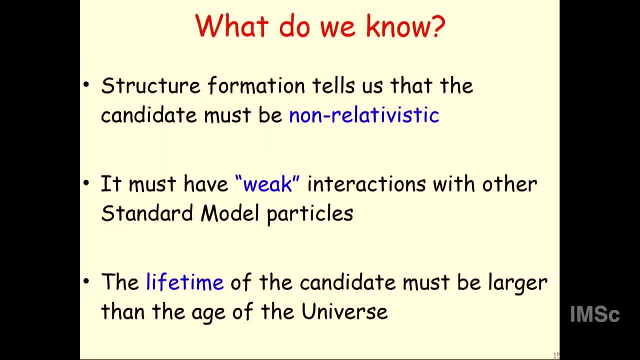 nothing wrong with it. So when you say non-relativistic, what do you mean by that? When I say non-relativistic, it means that currently it must be, for example, in the Milky Way. the velocity of dark matter is 10 power minus 3 C. Actually, in the solar circle. 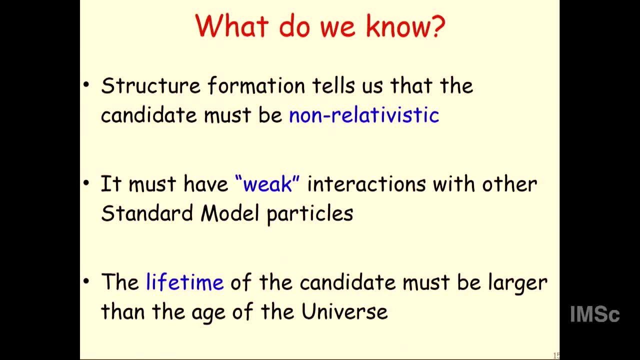 more precisely, The velocity of dark matter is 10 power minus 3 C. More precisely, it also means that dark matter which is beyond the Milky Way, in the universe as well. they are moving extremely, extremely slowly. So if you have very light particles, I mean 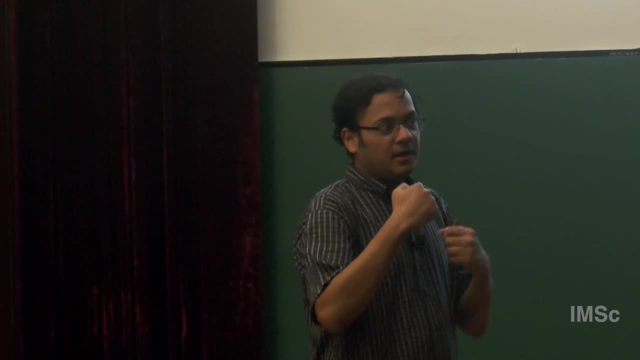 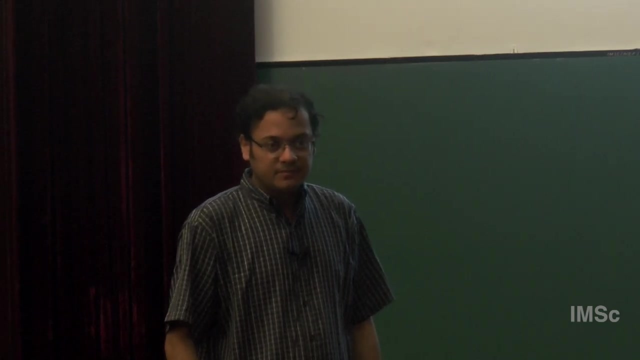 they do not talk to the. they do not talk to the universe, the temperature of the universe. They are never in thermal contact, technically, with the temperature of the universe. That is why they are non-relativistic. All right, For example, the way you are talking, the. 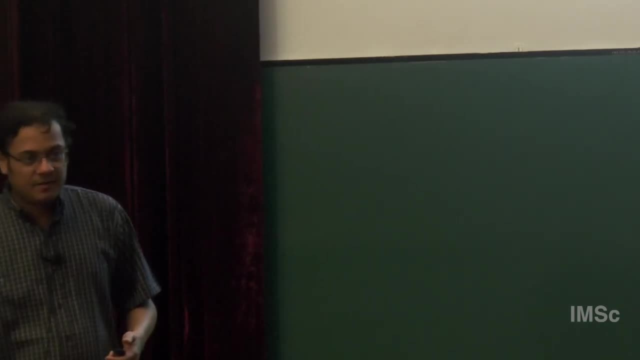 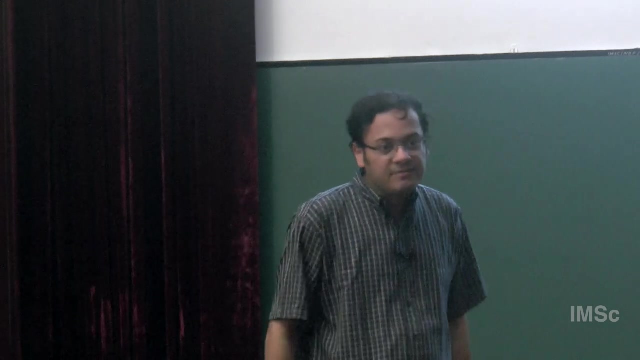 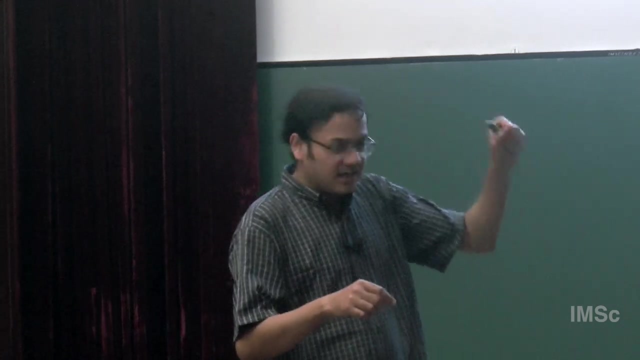 way you are asking the question is: we know the CME temperature, that is 3 Kelvin. We can convert that to an eV scale. That is 10 power minus 5 eV roughly. And if you take the dark matter particle as say 10 power minus 22 eV, then if there is a connection between 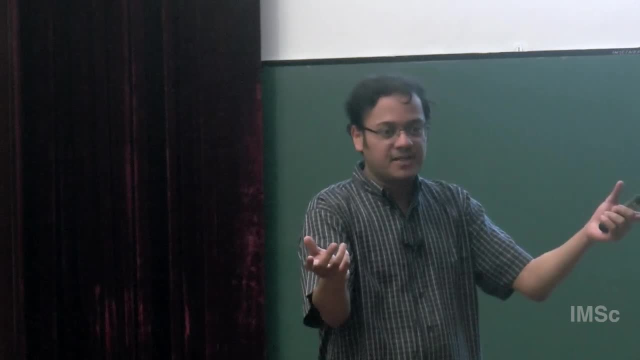 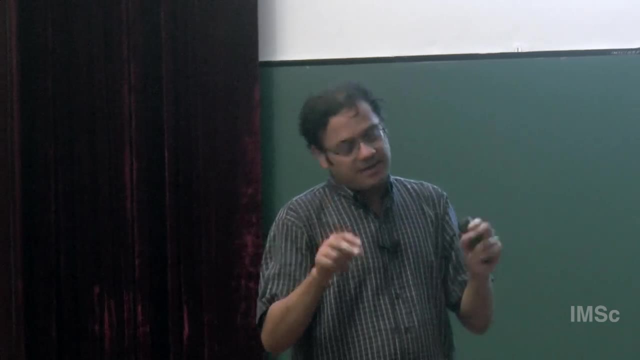 the CMB temperature and the dark matter candidate, then the obviously dark matter particle is moving at very high velocities. So that means if you take light particles it cannot have a connection with the temperature of the universe. If you take heavy enough particle, 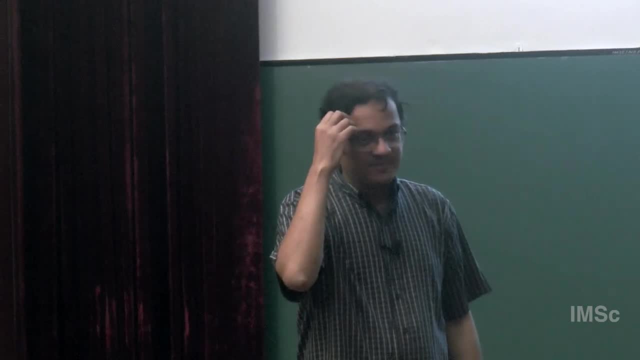 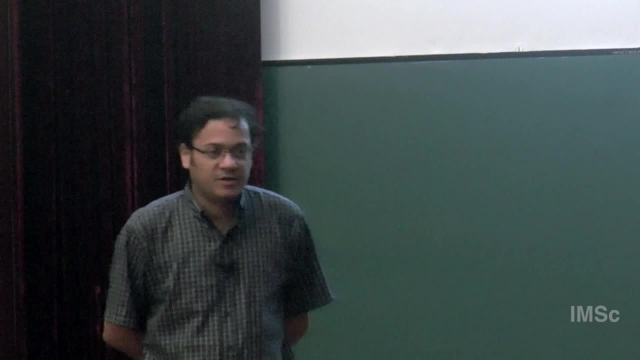 it can have a connection with the temperature of the universe. Does that answer the question? If it is a light particle, then they will form a condensate. They may form a condensate. I mean even there there is a when you are assuming they are forming a condensate. you 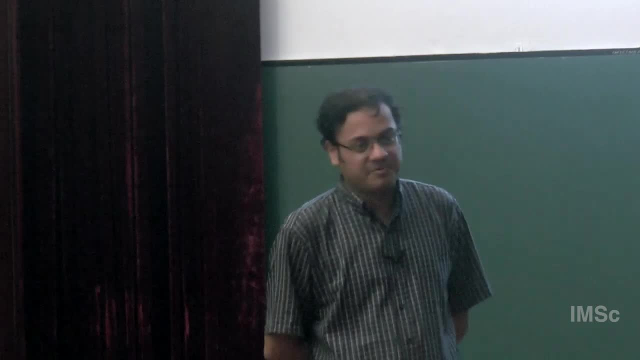 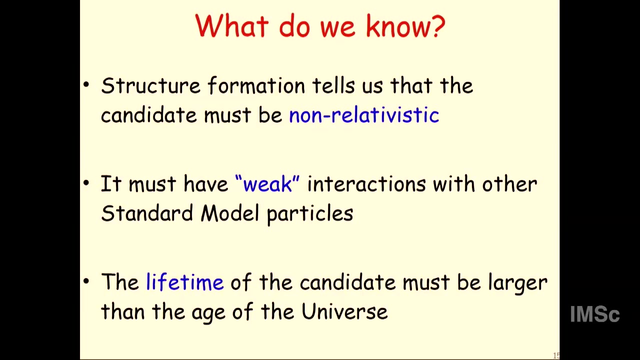 are assuming it is a boson. They can also be fermions, by the way. Then they will not form a condensate. So there are some caveats, All right, And I will be happy to talk more. Okay, Good, So what do we want to know? So the first question. as we were discussing, 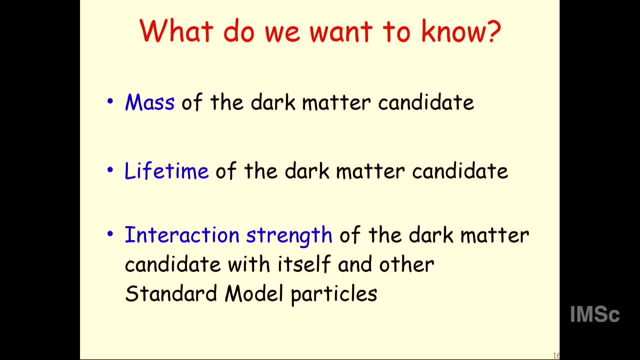 you could have guessed. what is the mass of the dark matter candidate? We do not know the answer. All right, You can ask a very simple question: What is the mass? We do not know the answer. What is the lifetime of the dark matter candidate? Again, as I said, we know its lifetime must. 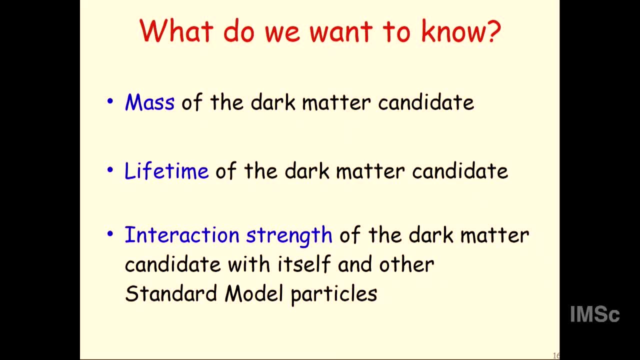 be greater than the age of the universe. What is the number? What is the number equal to? We do not know the answer. Okay, And thirdly, what is the interaction strength of the dark matter candidate with itself and with other stand-alone particles? How does it interact? 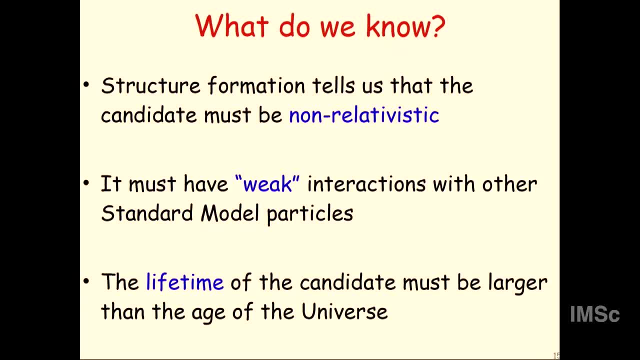 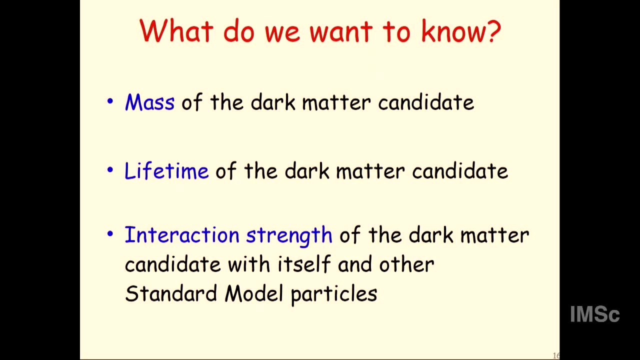 with other stand-alone particles. Remember, I said, it has weak interactions right within cores. That means its strength is smaller than some number. But what is exactly that number? We do not know the answer. Okay, So these are three of the major questions that we are trying to answer in dark metaphysics. 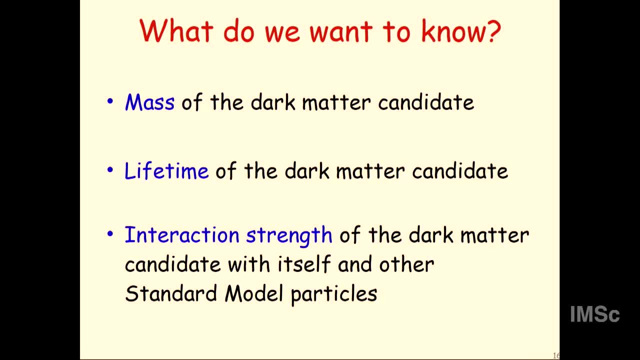 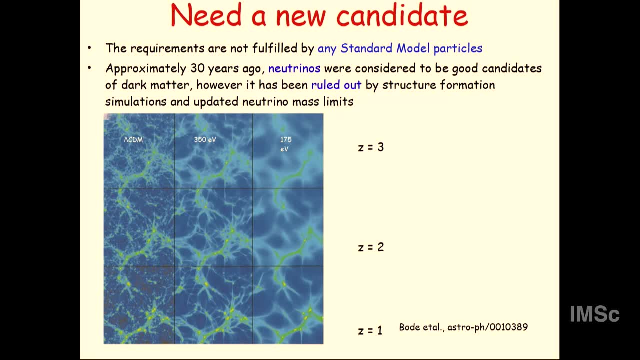 Okay, Good, So let us proceed. So now comes to one of these questions. So you can now say that, well, the fact that we require a candidate to be dark matter, why do not we look at the standard model of particle physics? right, That means all the particles that we 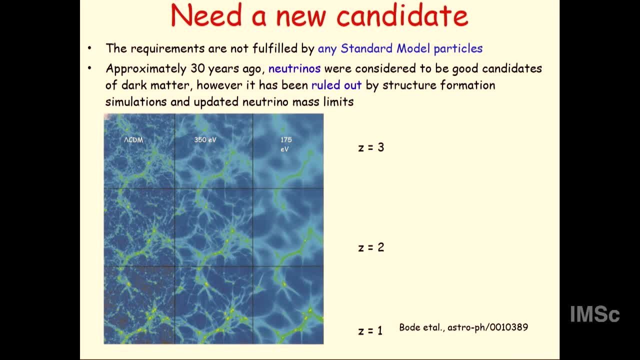 know of. Can any of one of those particles be dark matter? Turns out the answer is no, right. None of the particles that we know of can be dark matter, right? In fact, the particle which is, which could have been dark matter, is the neutrino, and that was already ruled. 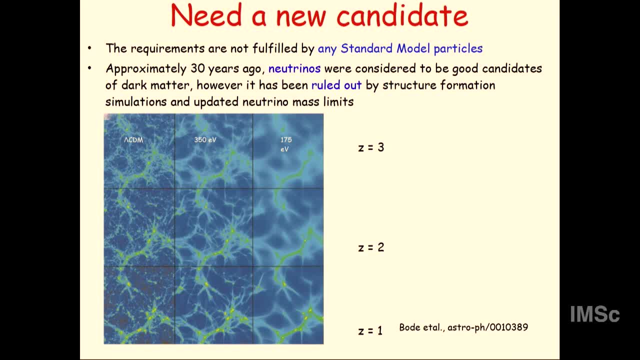 out two, three decades ago, right? So suppose this is actually a plot. Suppose you a simulation, actually. suppose you simulate the universe, assuming a dark matter candidate of much, much, much larger than the mass 175 eV. all right, You can show that it will actually. 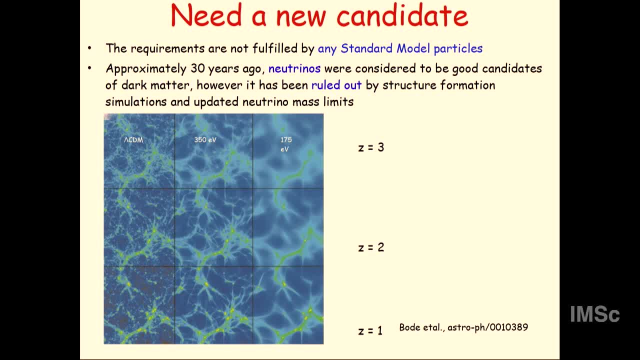 be relativistic, all right. And you simulate the universe at various redshifts, all right, Various times. So this is redshift 3,, redshift 2, redshift 1, all right, So these are various. 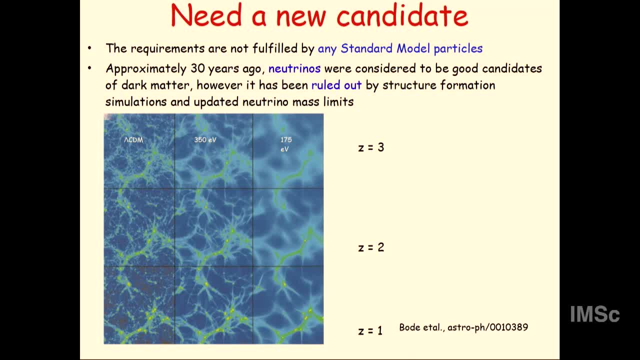 times. Redshift 0 is now, redshift 1 is roughly two or three giga years ago. right, And these are higher and higher, larger and larger times. all right, These are. this is these are early universe. Time is going up like this. all right, You get this observation, all right. 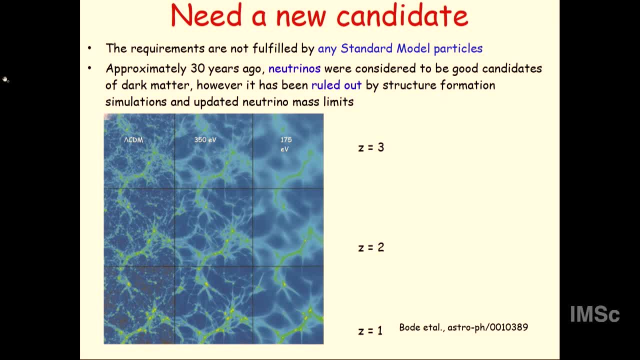 So if you take the dark matter part- suppose you take a heavier dark matter mass- all right, Candidate mass- and you make it non-relativistic- This will be relativistic. as I said, This will be relativistic If you make it non-relativistic. your structure formation happens like this: 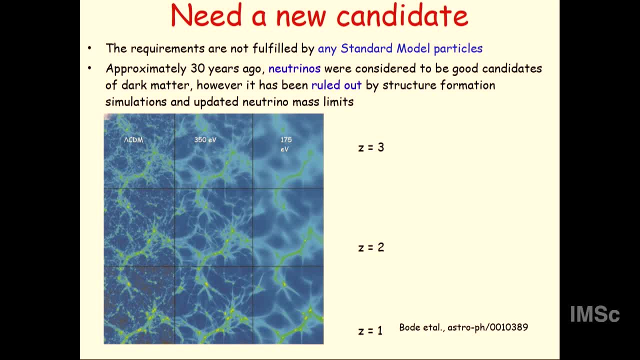 There is actually a reason. This is not. I mean. there is a physical understanding behind this simulation, and I can explain why it is, but let me just skip it. now Turns out, you can. you can take each of these slices and measure how the sky looks like. So what? 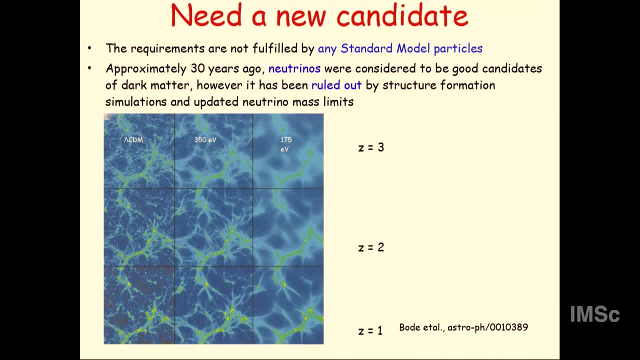 does this, this mean? This is all of these bright spots that you see in these pictures. these are centers of galaxies. all right, All of these are centers of galaxies. So, all of these bright yellow spots and all of these faint things that you see, these 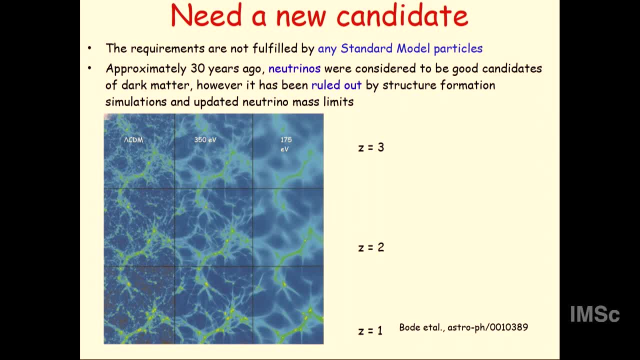 are filaments. That means matter connecting between two galaxies, and all of these dark spots are basically empty patches. So what does this mean? That means you are counting galaxies in a volume. That is what the picture is. all right, You just take observation volume. 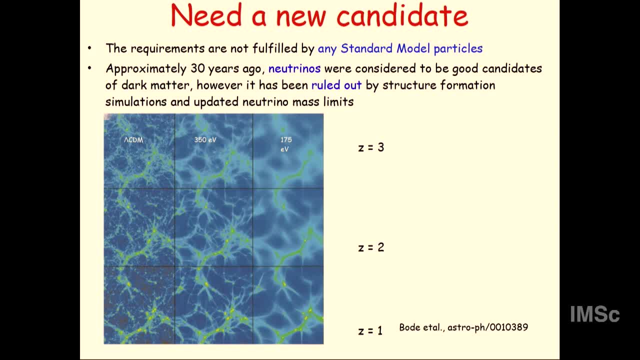 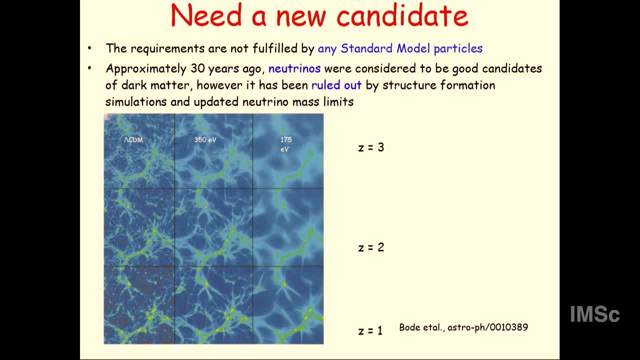 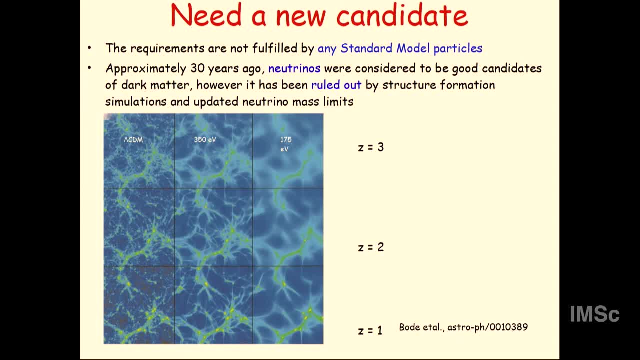 matches this picture. all right, If you make a large enough observation- large scale observation- the reality is actually like this. So this is like giga parsec length scales. If you observe the universe at giga parsec length scales- something like 109 parsec length scales- 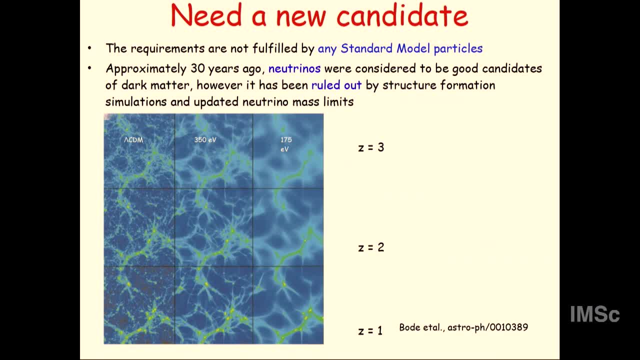 the universe looks like this. It does not look anything like this, all right, And this is pure gravity. all right, This simulation has pure gravity. nothing else Using this can show that neutrinos are ruled out as dark matter candidate. actually, you can. 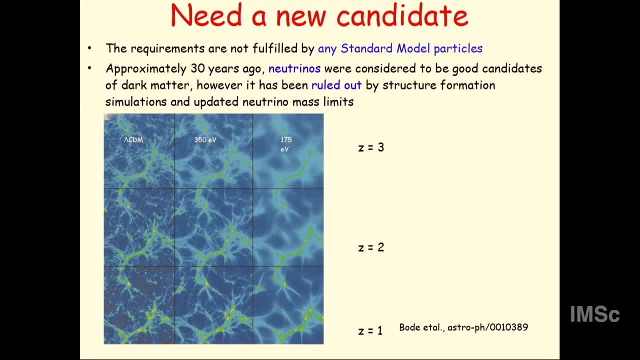 do even more right. these masses cannot be neutrino masses. more precisely, neutrinos must be much lighter. has to be much lighter orders of magnitude, at least two orders of magnitude lighter. right, these go even crazy. this, these simulations, all right. in other words, this is answering one of your questions. 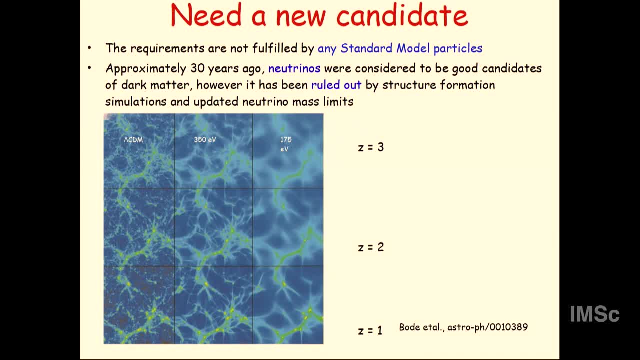 if dark matter is light, extremely light, then dark matter cannot be in thermal contact with the universe. right and just to give a scale in case people don't think of in terms of Evie, so this is once I have: Evie 1g. Evie, that means 10. 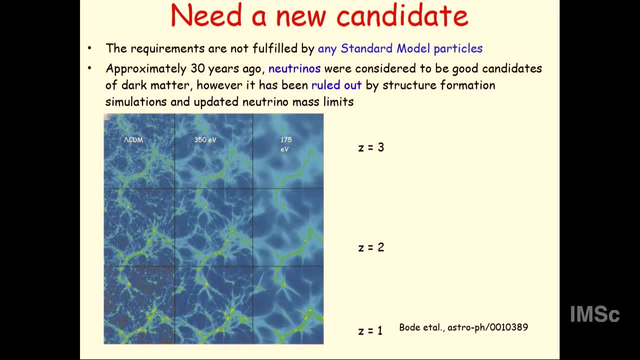 power 9, 10 power 9- Evie is the mass of the proton. so this is roughly 10 power, 7 times smaller than the mass of the proton. this particle, right, okay, so the universe looks like this. so this tells you the dark matter must cannot be. 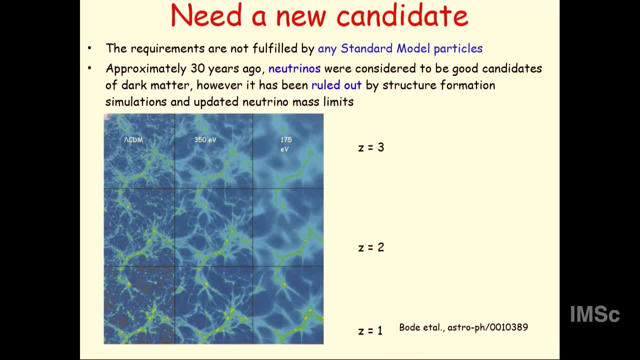 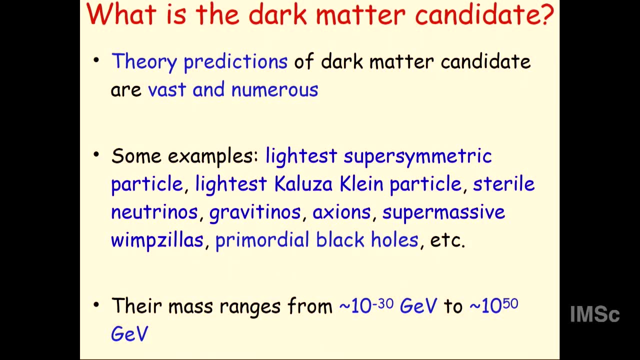 neutrinos. first of all, it cannot be in. it has to be non relativistic. this is one of the proofs that it has to be non relativistic, right? so these are the ones. the theory of dark matter, that could be dark matter, okay, okay, good, so what is again? so what then? what? 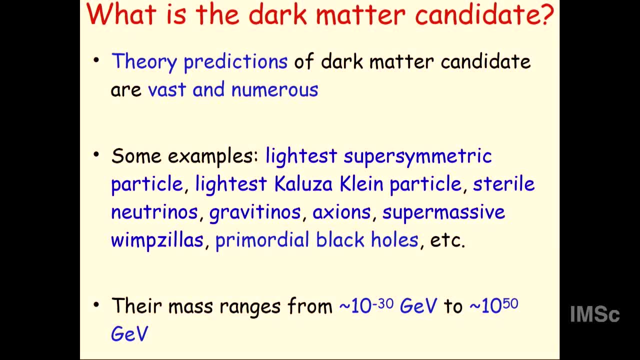 again, we don't answer the question. we just ruled out neutrinos, right? we didn't answer the question. what is that? the sac matter candidate? turns out that the theory predictions of what dark matter candidate can be are vast and numerous. there are many, many, many things, say. some of the famous models are the lightest. 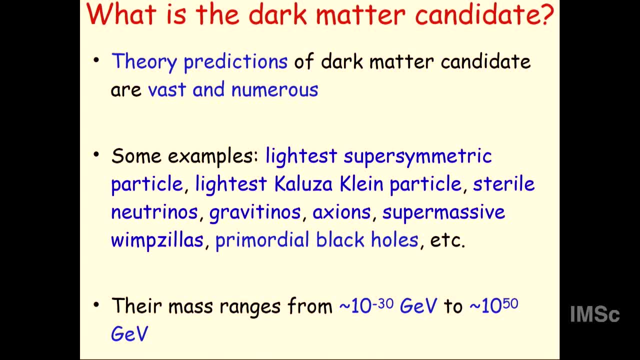 supersymmetric particle light as colors, the client particles try neutrinos. gravity knows axions are meaning just goes on and on. alright, the lightest a candidate can be is roughly 10 to the power minus 30 GeV. Again, 1 GeV is the mass of 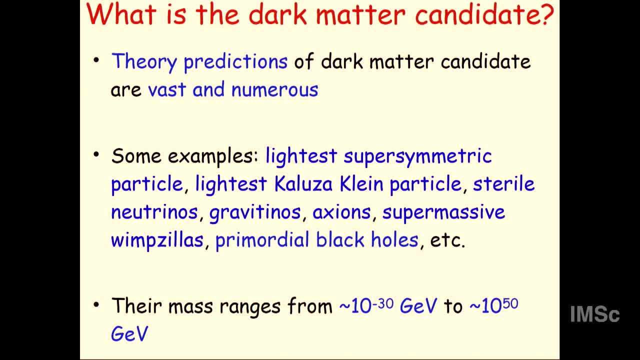 the proton. That means the dark matter candidate can be 30 orders of magnitude lighter than a proton. It is still allowed, Everything can be fine. A dark matter candidate can be 50 orders of magnitude heavier than the proton. Again, everything is fine, As long as you. 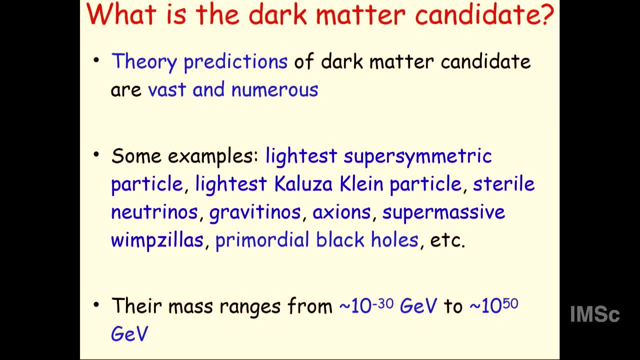 make up the things properly. So you see, there is 80 orders of magnitude where dark matter can be. Again, as was discussed, if the dark matter becomes very light, you have to make it non-thermal. That means it cannot come in thermal contact with the universe. 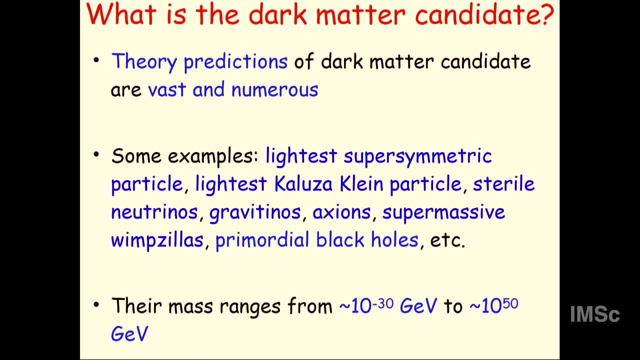 That means it cannot scatter with the universal particles, It cannot have the same temperature. If you have this, then this whole range is allowed. So the point is to search in this whole range and figure out what is the dark matter. candidate, Is this clear? Okay, good. 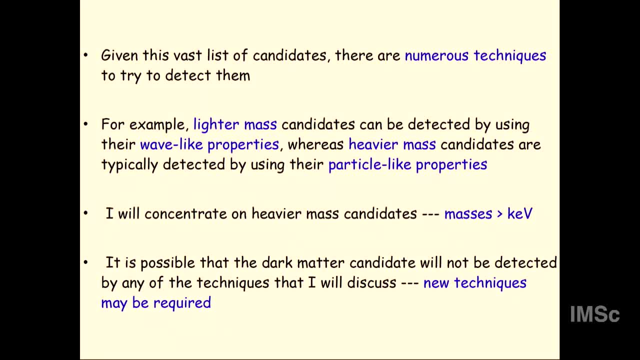 So obviously, now you see, there are 80 orders of magnitude, So there is no one technique that can be used to detect them. There are numerous techniques one employs, For example, lighter mass candidates can be detected by using wave-like properties. What does this? 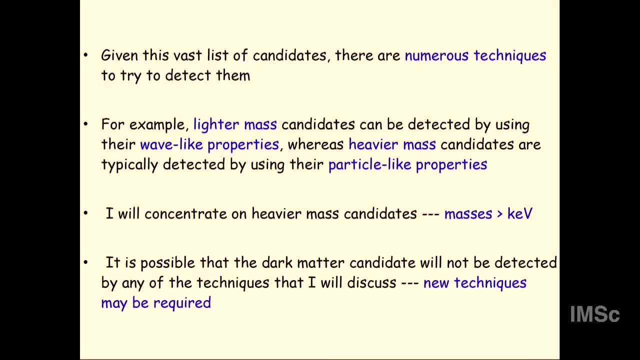 mean If the dark matter candidate is extremely light, then the phase space density is very high. If you take a given volume, the number of particles is very high Because, again, we know the dark matter density extremely well, as I said In this room, we know the 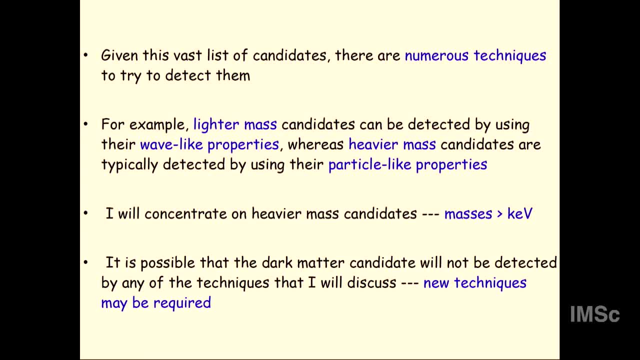 dark matter density within a factor of within 30% accuracy roughly. So we know the dark matter density extremely well. So if the dark matter particle is extremely light, there will be many dark matter particles in this room. Then we can treat it as a wave as 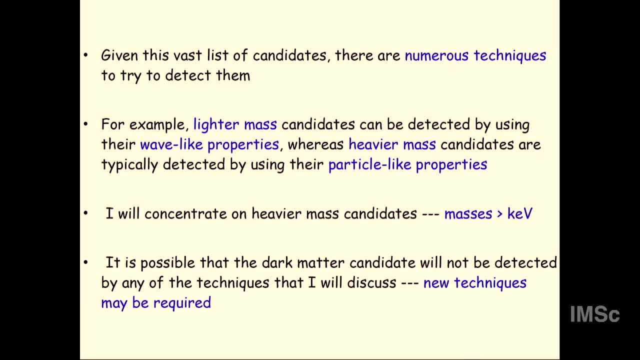 a fluid, Whereas if the dark matter particle is very heavy, then we can treat it as a single particle moving around. This thing can be quantified. If you are interested, please ask me. I will be happy to answer. In this talk I will be talking about heavy dark matter. 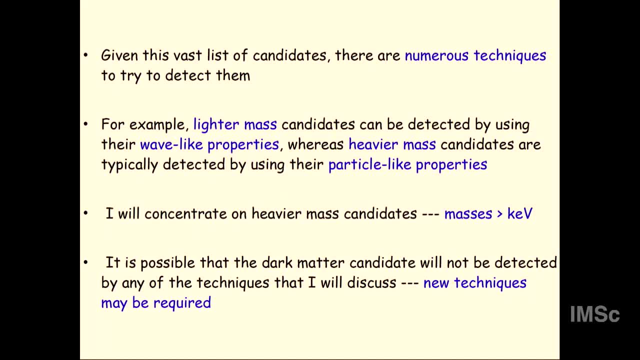 candidates. So let us talk about heavy dark matter candidates, which have a mass greater than kilo electron volt. Now, it is certainly possible that dark matter candidate will not be detected by any of the techniques that I will discuss. It is also possible that dark matter candidate 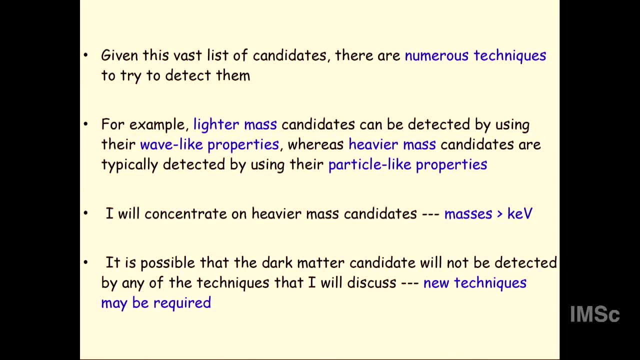 will not be discussed by any of the techniques that we have thought about. So we do. new techniques may be required, But it is also useful to fully utilize the current techniques, in addition to searching for new techniques to search for dark matter. 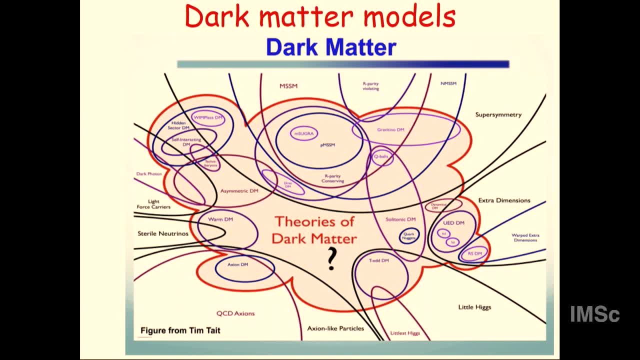 So I will show you two cartoons. So these two cartoons are very famous in the sense that how various theories of dark matter are incorporated into various other particle physics theories. So this is the famous super-symmetry Sort of the various models of super-symmetry. 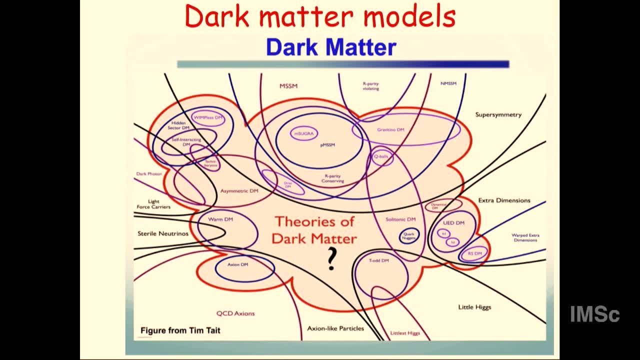 and almost all of them have dark matter candidate. That is one of the things which you try to solve. It is sort of like an external input, but you try to include that There is extra, that little eggs, QCD, axions and various other things. 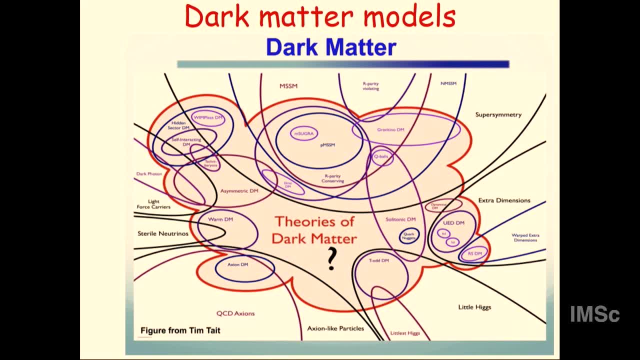 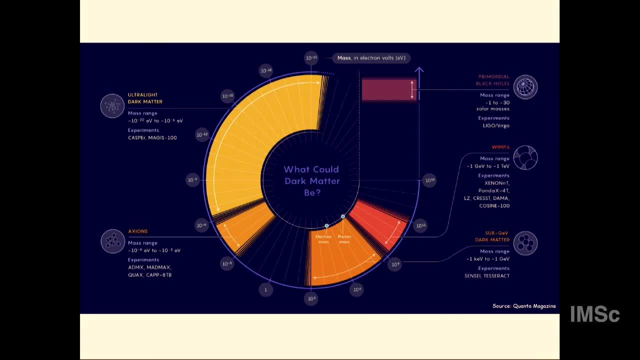 And there are people here in IMSE who work in many of these topics- Then this is also sort of a very nice cartoon recently released by the Quantum Magazine, which tells you the various candidates of dark matter. As I said, the lightest particle can be as light as 10 power minus 22 eV. 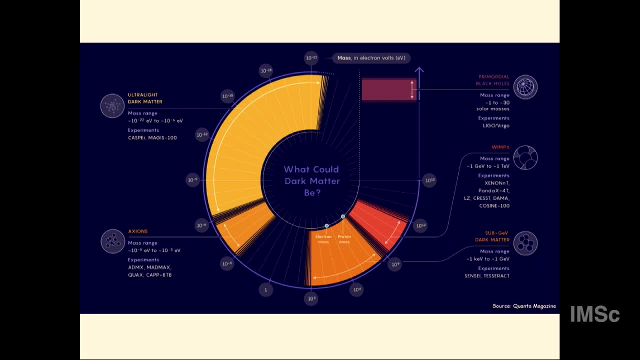 which is roughly 10 power minus 30 g eV. very roughly, And the heaviest particle can be roughly 30 solar mass, which is roughly 10 power, 50,, 51 g eV or even more than that. 30 solar mass is 10 power, 58 g eV. 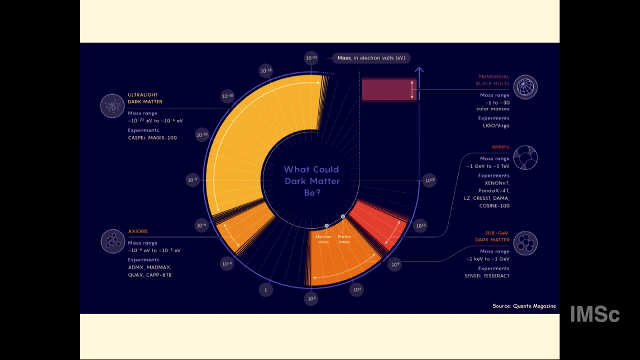 And there are various ways to detect it. So this thing- ultralight, dark matter and axions- these are detected as waves, as I told you, And these are names of various experiments: CASPER, MAGIS, ADMX, MADMAX, various experiments. Yes. The reason is as follows. Let me tell you the reason Why. Now you can ask: wait, why is this stopping at 10 power minus 22?? Why not? The reason is as follows: We know the size of dwarf galaxies. 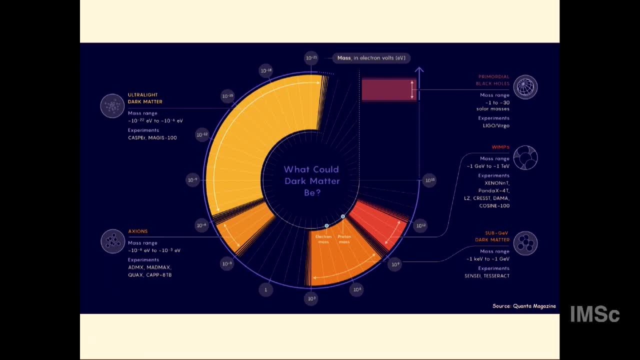 dwarf galaxies are satellite galaxies. They have a size of roughly 1 kilo per sec. We know dark matter is inside those galaxies because we see observationally. we see rotation curves and we see them Now at this length scale, since dark matter is localized inside that galaxy. 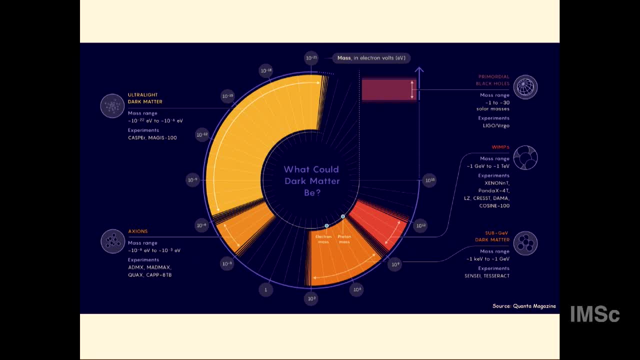 the de Broglie wavelength of the dark matter must have a size less than the size of the galaxy. all right, De Broglie wavelength is 1 over mv. right, We know the velocity of dark matter candidates. That has to be. we are moving the galaxy. 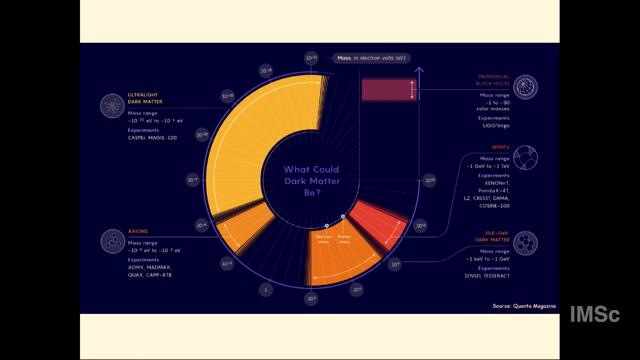 That gives you a limit of m. From that we get this number: 10 power minus 22 eV. all right, Although technically I mean there are caveats in the sense that when I said all this story, I assume there's only one dark matter candidate. You could have asked who told you that there's one dark matter candidate. There are many two. Then you can wiggle around these things, But in the most minimal scenario this is the smallest mass dark matter candidate can have and be the only dark matter candidate in the universe. 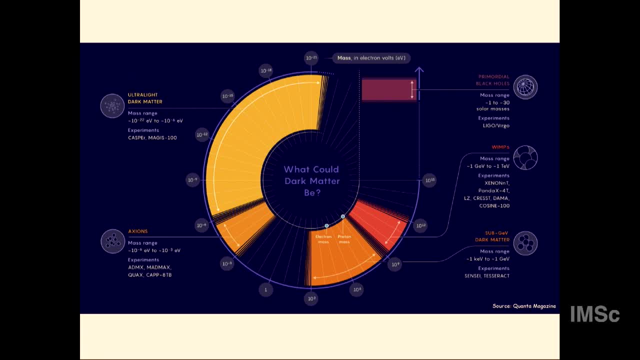 All right. So that means if there's one kind of particle which makes up the whole of dark matter, it must be greater than 10 power minus 22 eV. all right, This is a very robust argument. De Broglie wavelength is smaller than the size of the galaxy. 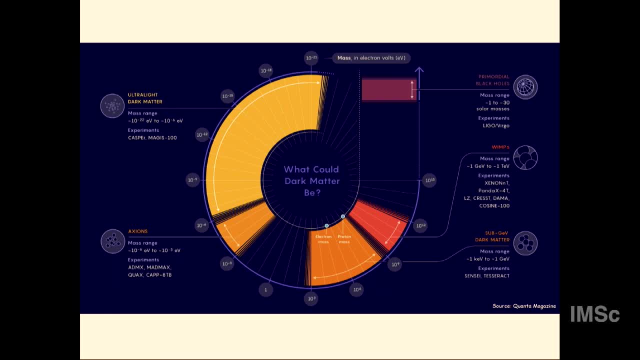 because the dark matter is localized inside it. right, Simple thing. It will give you the answer immediately. Okay, good. And then you can ask: what is the why this, why you stop at 30? so-and-so Okay good. And then you can ask: what is the why this, why you stop at 30, so-and-so. 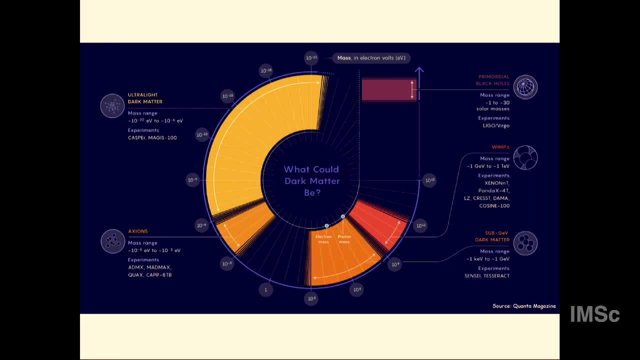 Okay, good. And then you can ask: what is the why you stop at 30? so-and-so Okay, good. And then you can ask: what is the why you stop at 30? so-and-so? Well, the smallest galaxies that we know of are 10 power, 7 solar mass. 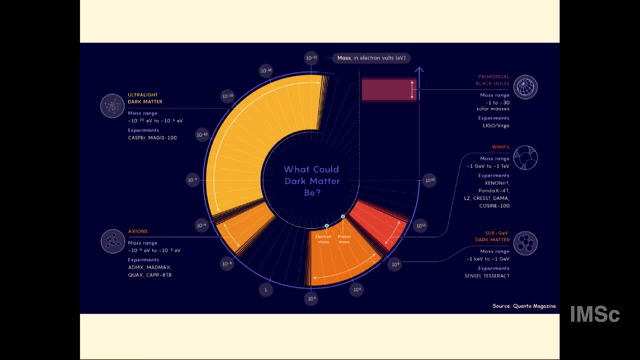 So that means that that's the maximum size dark matter can have. Again, if there's one candidate which makes up the full dark matter density, right, But turns out that if you go much beyond this number there are other problems with lensing and other things. 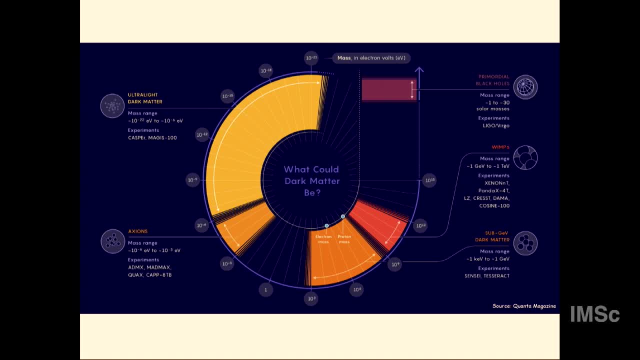 Again, I'll be happy to discuss, And so that's why we stop at roughly a few hundred solar masses. That basically sets the limit, all right, And then, as I said, anything in between can actually work. So note that the electron mass is somewhere here. 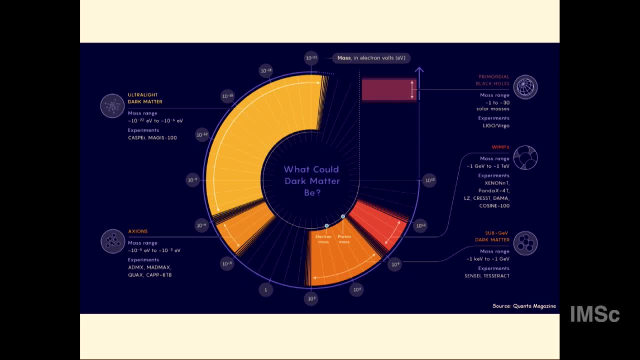 the proton mass is somewhere here. the neutron mass is somewhere here, right? So everything that we know is in this range. Everything else can be is a free game. Okay, good, So let's talk about the relic density, all right? 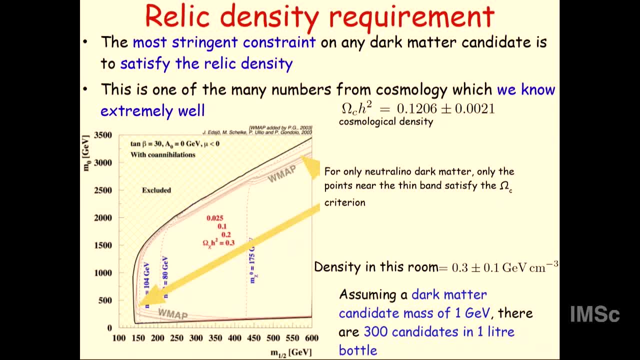 So the relic density means what? What is the density of dark matter in the universe? The energy density of dark matter in the universe? all right, This is a number we know extremely, extremely well. as I said, We know this number to 1% accuracy. 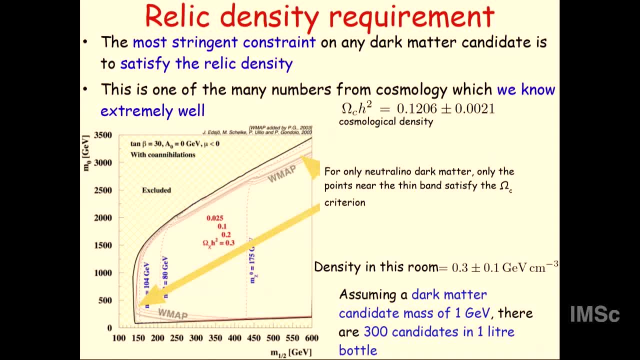 From the recent cosmic microwave background data, we know this number. This is the thing I mean. it's a fancy way to write it. right, Forget this thing, but this is a fancy way to write it. but the answer is 0.12 plus minus 0.0021, all right. 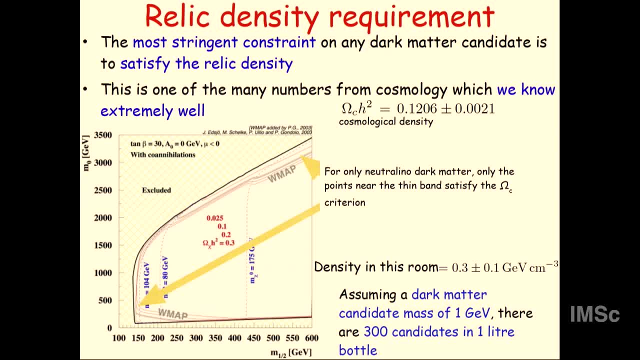 In dimensionless units. you just normalize the density. all right, I'll tell you. what does it mean? So this is the cosmological density. That means if you measure the dark matter density of the whole universe, you get this number in some normalized units. 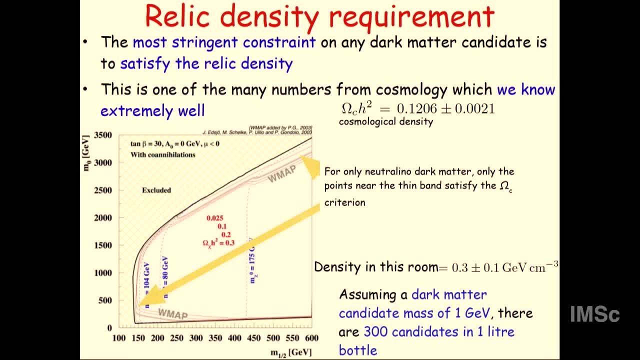 This is basically the roughly two 1% accuracy that I was telling you about, So this number is known extremely well. In fact, this number is known so well that, if you postulate any model which can reproduce the dark matter density- 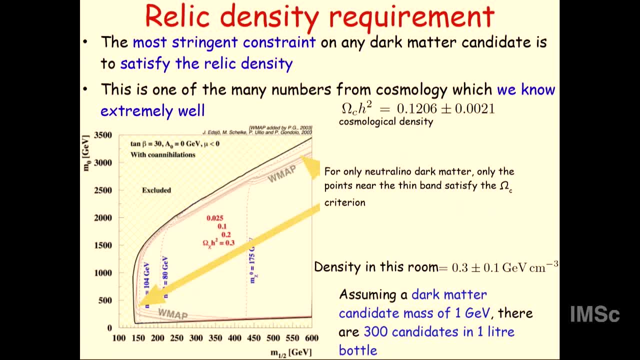 getting this number correct is extremely difficult. all right, Now let me show you an old plot. I have purposely chosen an old plot, just to show. even in 2003, this was extremely difficult, right? And in 2003, the error bar was not 1%. 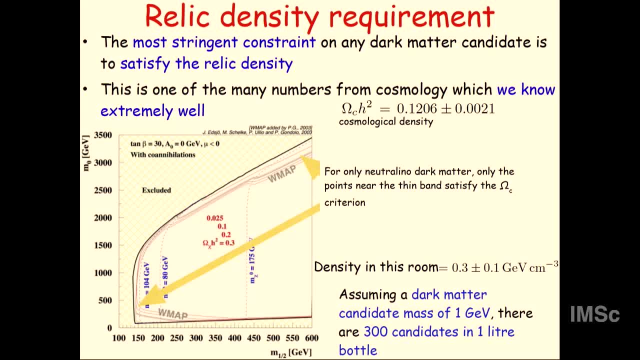 It was slightly more than that. So what is being plotted? So this is some supersymmetric parameter space. all right, So some parameter, some parameter on the x-axis in some particle mass, some mass in the x-axis and some mass in the y-axis. 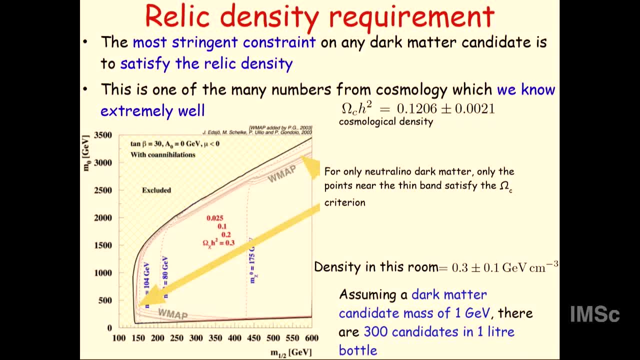 You don't need to go into the details. all right, Anything that you see shaded is ruled out. all right, Anything in this whole region is ruled out. I'll come to that. Let me just finish this and then come to it, okay. 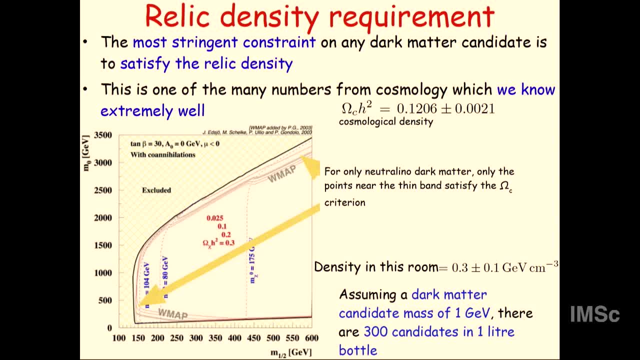 And because this is actually this thing, all right. So, if so, this. as I said, this comes from the Planck satellite. The previous iteration of the Planck satellite was WMAP satellite, If you wanted. this is what happened. 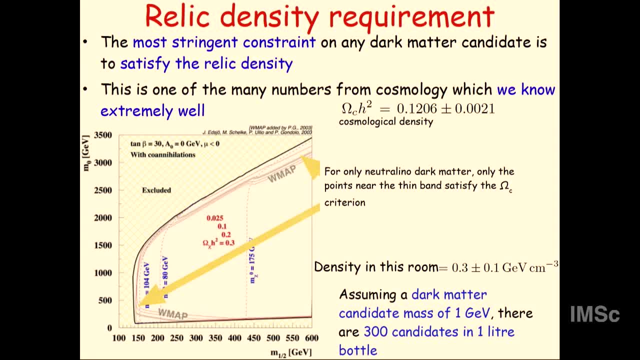 So, if you want, you can see that this model, this supersymmetric model, reproduces the occurring dark matter density. only this thin regions that you see are allowed. This thin regions are allowed, all right. Everything else is ruled out. If you want, 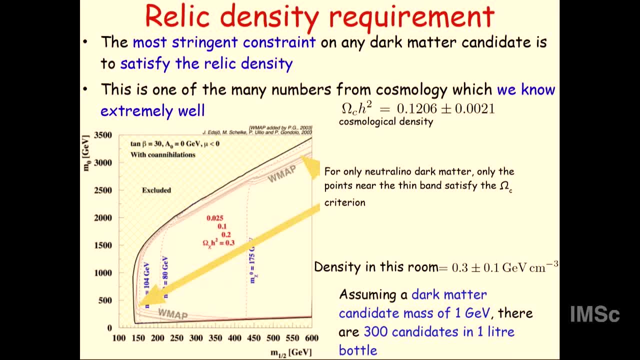 if you want that requirement that my new physics model will have a dark matter density, then only this thin region is allowed. As I said, from laboratory observations this region was ruled out. this excluid region, that means laboratory observations, not from cosmology or astrophysical observation, from laboratory observations. 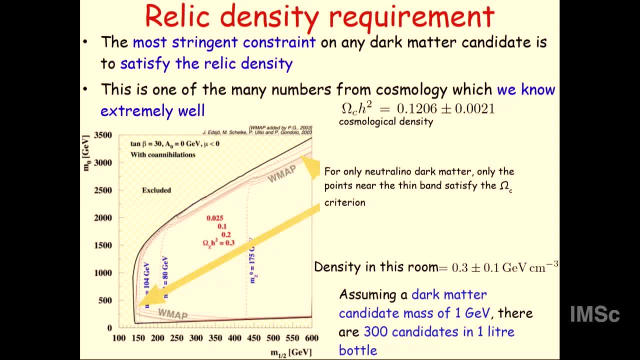 all of this white region was allowed, once you put in the fact that you need dark matter, only this thin, thin lines. you see, i mean only this thin line is allowed. it's a very rough way to explain this plot. all right, now let me come to the question. so this question was asked is this: 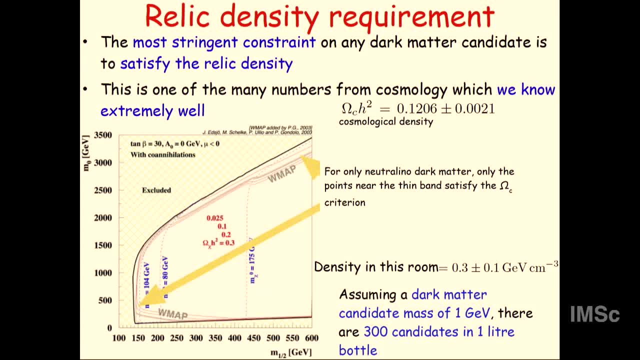 number uniform. so, as i said, this number- i mean i've written it in a dimensionless way- is the dark matter density of the whole universe. but actually the dark matter density in the whole universe is not the same. for example, the dark matter density in this room is roughly five. 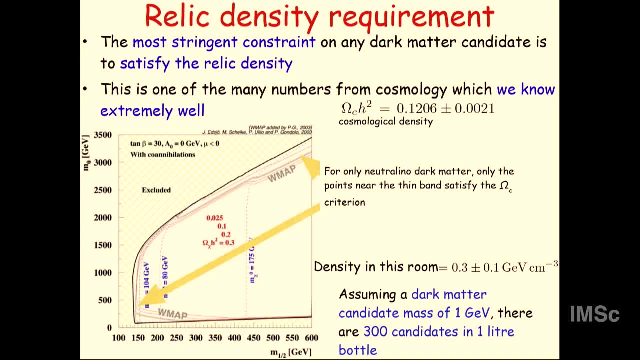 watt of magnitude higher than this number. all right, uh, for example, the density in this room is 0.3 gev per cubic centimeter. right, it's a fancy way to say this. basically, it means that if you have a dark matter candidate with a mass of one gev. 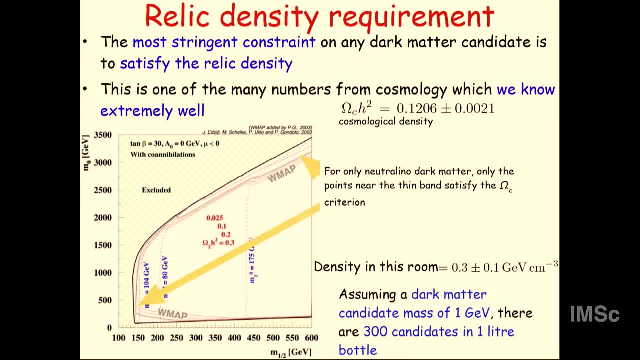 then in a one liter water bottle that you have, there are 300 dark matter candidates inside that right. so you see, this is this, this number and this number differ by four to four orders of magnitude. all right, that is simply because in inside, if you go inside a galaxy, the galaxy is a. 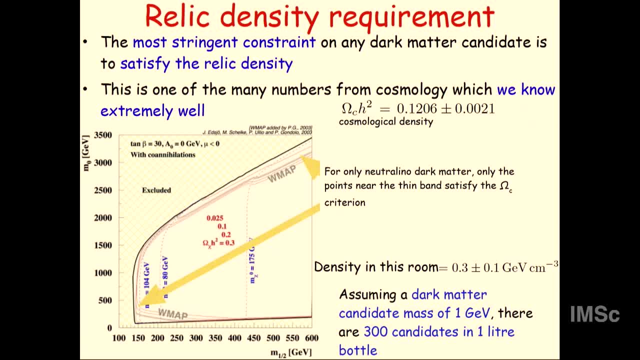 non-uniform thing. the potential, well deep, depends. and then there's there's a clumping of dark matter. more precisely, i mean more technical terms, clumping of dark matter. so, if you remember, most of the universe is actually empty. so for most of the universe this number is true, but the moment 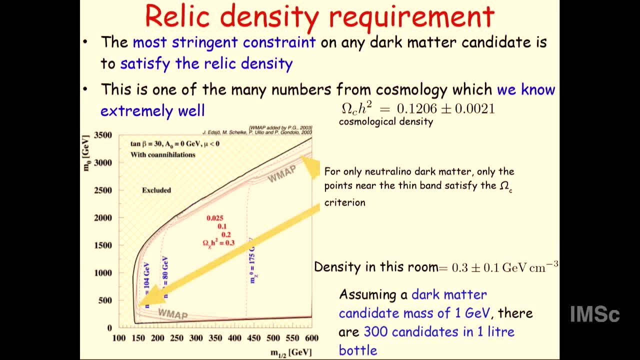 you hit a galaxy, your dark matter density increases. and i'll tell you, i'll show you a plot very soon which shows you how the dark matter density inside a galaxy changes with the distance. correct, yes, yes, correct, yeah, i'll show you that. okay, good, good, we don't know that answer. i'll show you a plot. there's huge uncertainty. 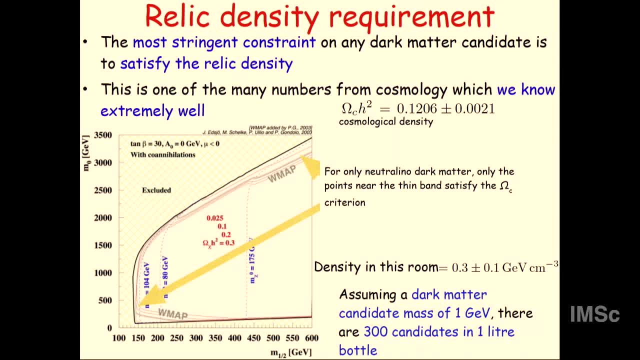 okay, since you have, since this question was asked. so remember i told you this number is known from cosmological observation. that means looking at the cosmic microwave background. how do you know this number? you can ask, wait a minute. this number is known to one person accuracy. the whole universe is known to one person accuracy. and suddenly you say that. 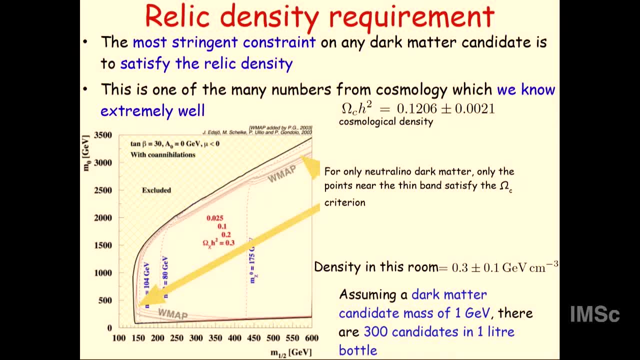 the solar system is known to 30 accuracy. how is that possible? so this number is measured in a different way. this number is measured by basically looking at stars near the sun. how are they moving right? so you look at stars moving. so basically, this is the galactic plane. the sun is in the 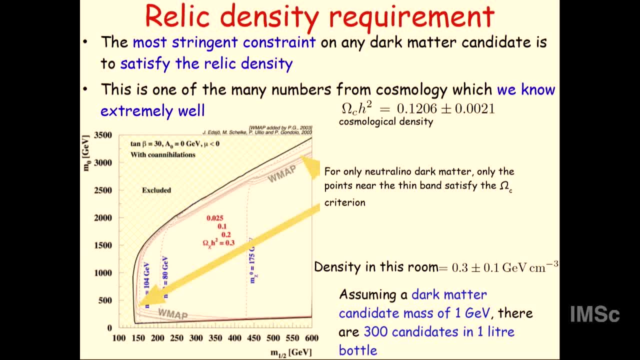 galactic plane. and then there are stars which are moving like this. there are many stars moving like this. okay, from the motion of the stars you can get this number. and why is it so uncertain? why is there uncertain to 30? simply because we don't know the baryonic density very well. 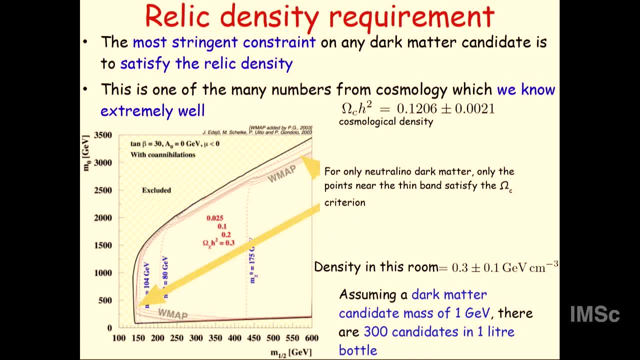 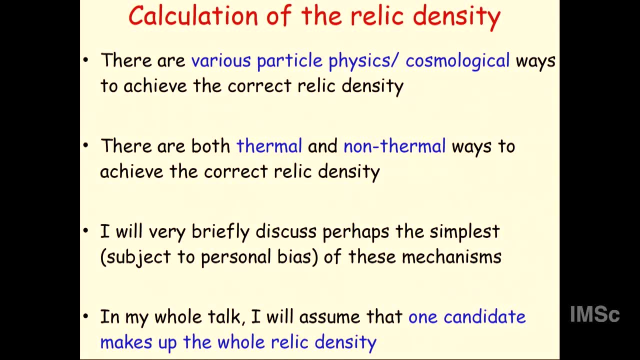 right. and then there are other reasons again i can discuss in detail. all right, okay, good, so i don't know how much time i have. so so, as i said, the various particle physics and cosmological ways to derive the correct relic density, all right, they're more, both thermal, 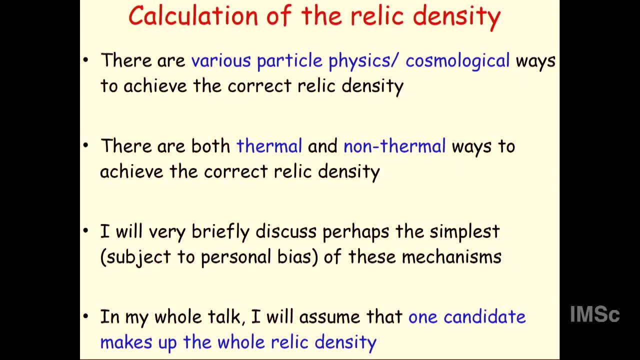 to achieve the correct ray density. What does this mean? Thermal means that the dark matter particle has scattered with the matter in the universe. Non-thermal means the dark matter particle has not scattered with the matter in the universe. That is what it means, right? 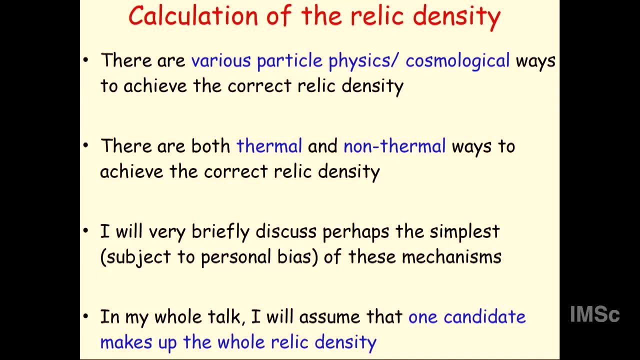 That means this again. in other words, thermal means it shares the same temperature as the universe temperature. Non-thermal means it does not share the same temperature as the universe temperature. all right, I will discuss one of these mechanisms, And in this whole, 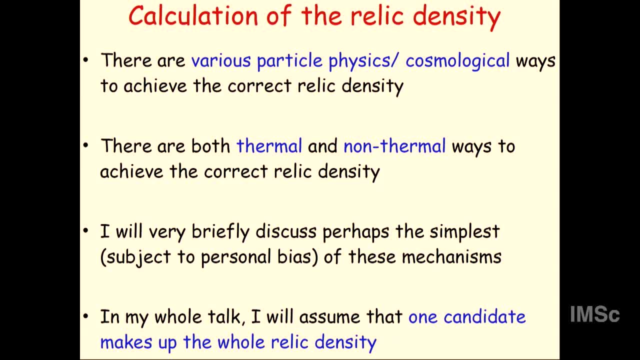 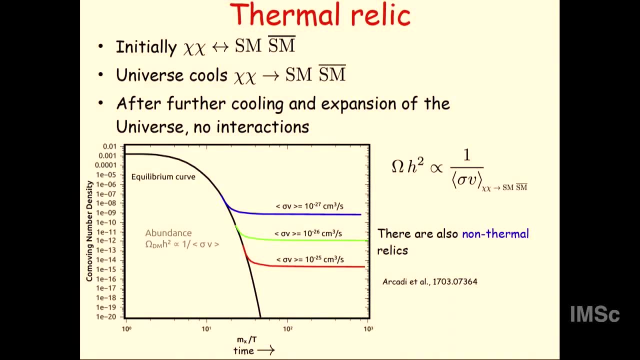 talk. I will assume there is only one candidate which makes up the whole dark matter density. all right, This is an assumption. but this is an assumption which can only be tested by doing experiments, observations and theory. okay, So this is one way to get the correct. 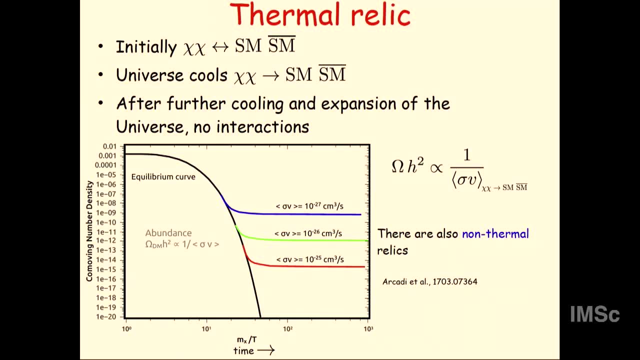 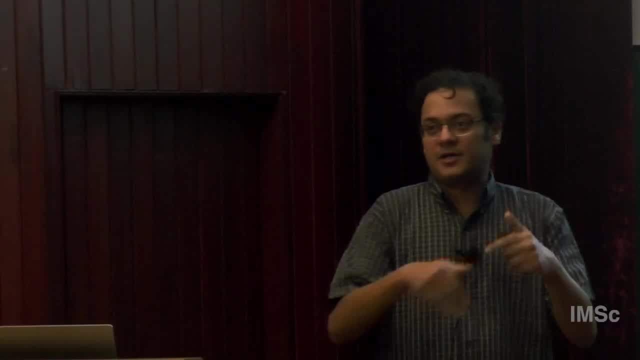 dark matter density. And the story just follows. Initially dark matter particles, and this is called the thermal relic. That means here the dark matter is produced by collisions with standard model particles. right, There are other ways. as I said, there are other. 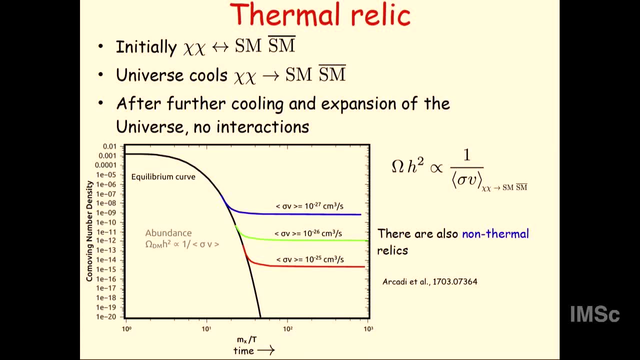 ways. there are also non-thermal relics. all right, I will not discuss that, Okay, well, how is dark matter produced Here? the story is that at the very early universe, when the universe is extremely dense, dark matter candidates- I denote this by chi- and standard model particles will collide. 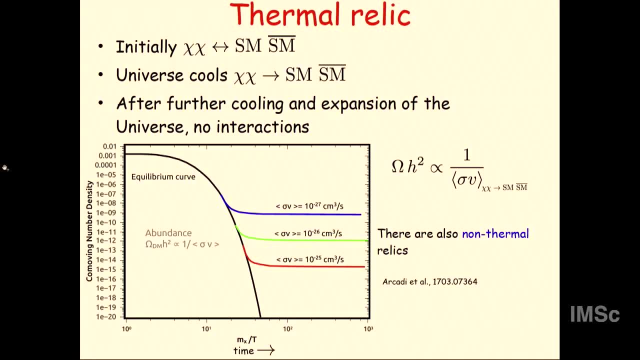 among themselves and interconvert. all right, As the universe cools. I assume that the dark matter candidate is heavier than some standard model candidates. all right, Standard model means all particles that we know of. So, because of kinematics, since the universe has cool, 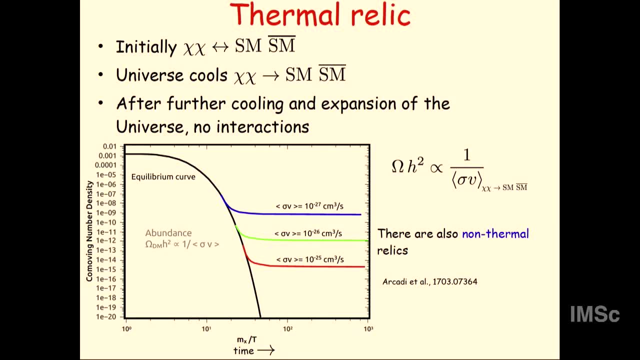 has temperatures decreased. this interaction will not go both ways. This interaction will only go one way. all right, One way to look at this. let us assume that the dark matter candidate mass is 100 GeV- all right, And the electron mass is 0.5 MeV- right, Unless. 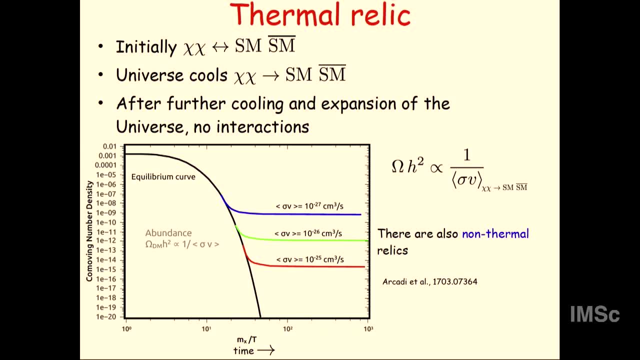 the background temperature is: unless the electron has enough energy you will not produce 100 GeV particles. Two electrons colliding will not produce 100 GeV particles. that is just energy conservation. You have to accelerate the electrons to 100 GeV of energy to produce. 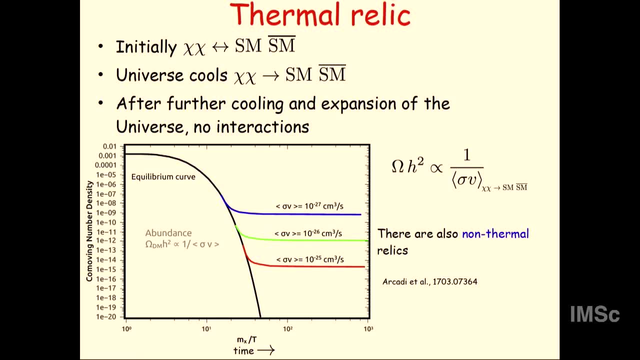 them right. But once the universe cools, that means once the temperature of the universe goes less than 100 GeV, the electrons, the electrons are thermal electron. that means electrons talk to the universe, talk to the factors. So the electrons are thermal, the 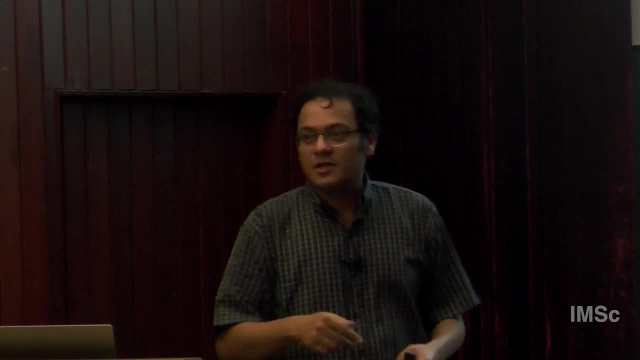 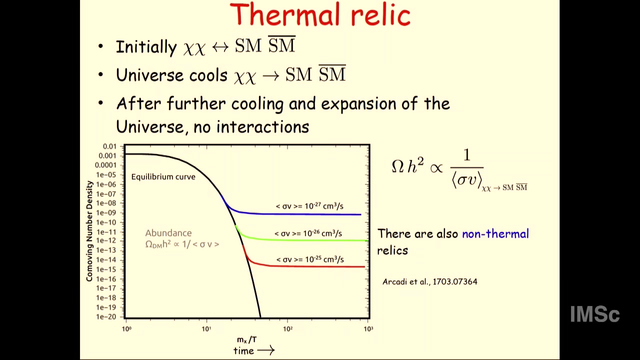 talk to the photons of the universe. They follow the temperature of the universe. Once the temperature of the universe goes less than 100 Gb, roughly again there is a factor of few here and there, but let us forget that Two electrons colliding will not produce dark matter. 100 Gb dark matter. 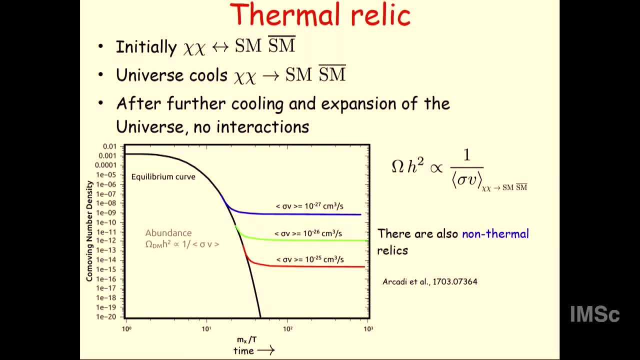 particles, Energy conservation will not allow that, But two dark matter particles with 100 Gb. they can collide to produce electrons. Again, energy conservation allows that. So this happens. Now something funny happens. and this happens because the universe is expanding. See, in this process there are two dark matter particles which are coming close to each other. 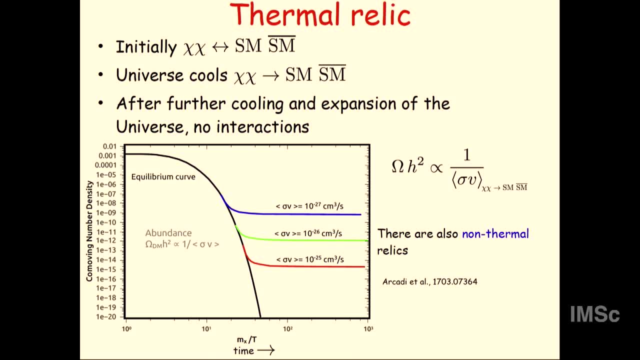 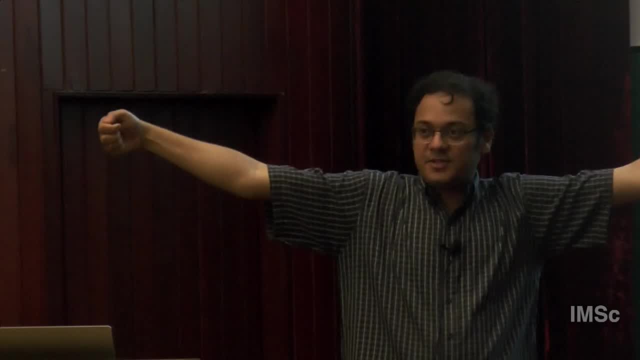 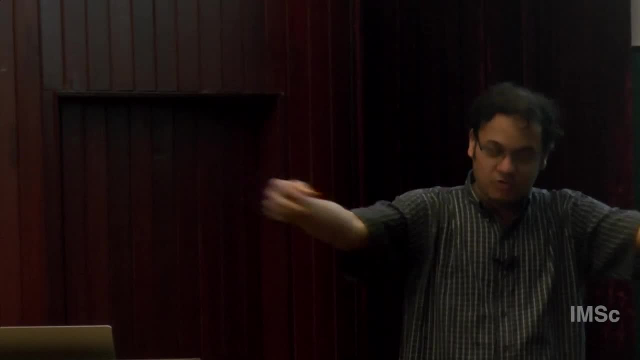 and colliding and producing some strand wall particles. But the universe is expanding. That means two particles are trying to come close to each other. The space between them are increasing. So you take a sort of some elastic sheet, take two balls, let the two 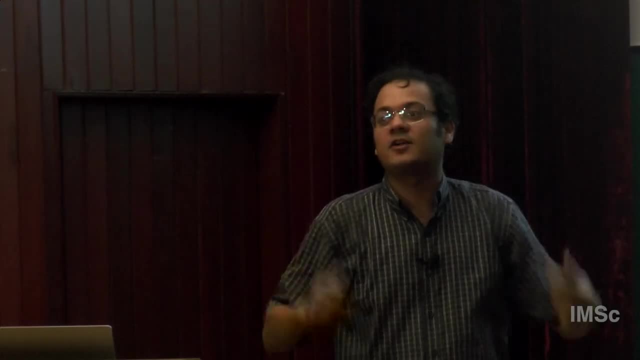 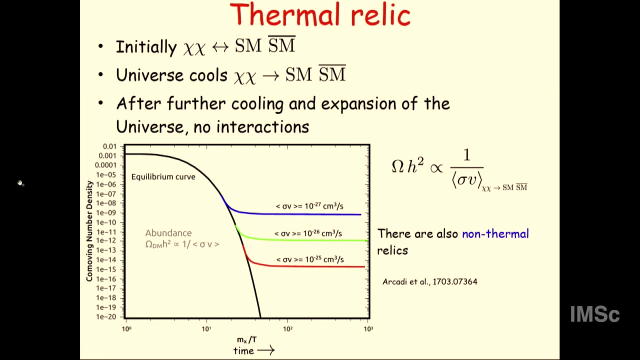 balls come together. If you pull the elastic sheet fast enough, the balls will not come close to each other. This is exactly what happens At some point. they they are two rates. Mathematically, there are two rates. One is the rate of this interaction, The other is 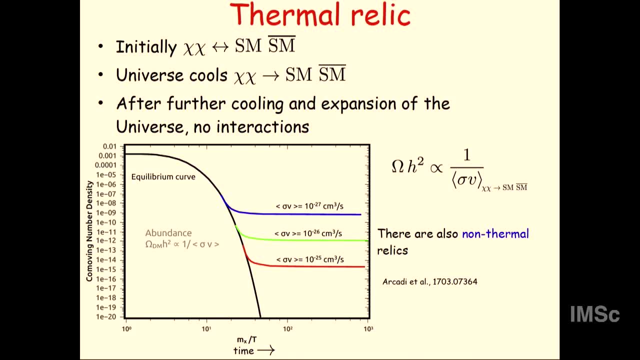 the rate of expansion of the universe. Once the rate of expansion of the universe exceeds this rate, this interaction also stops. That means dark matter particles will not come close to each other to interact. So you can do whole thing mathematically. This can be done in a very sophisticated way. 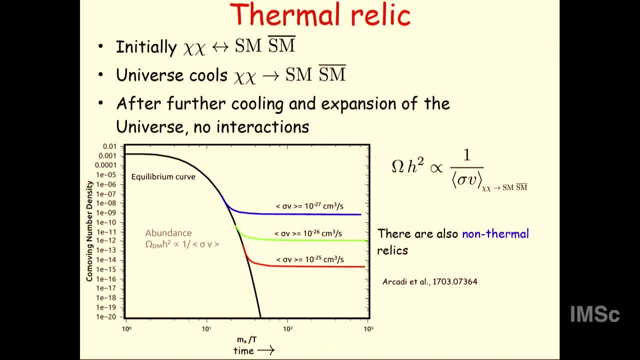 What you get is as follows: What is plotted in this thing is the time. So this is early time of the universe, This is late time of the universe And this is the abundance. So this is the equilibrium curve. That means if you are always having this interaction, then you are following this. The number density of dark matter will follow this curve. 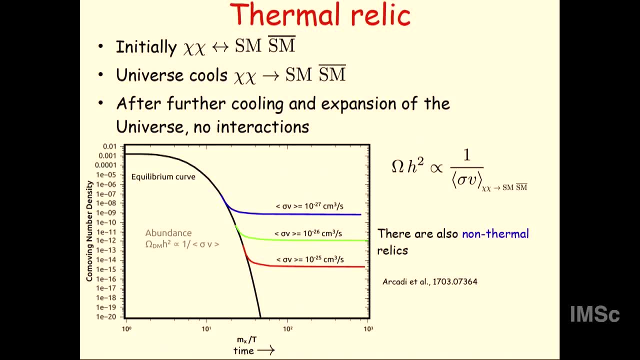 All right Now, depending on, remember, depending on this interaction, this cross section of two dark matter particles producing strand-mold particles, depending on this number, where does this interaction stops? depends on that. As I said, remember, there is a competition between two rates. One is the rate of this. 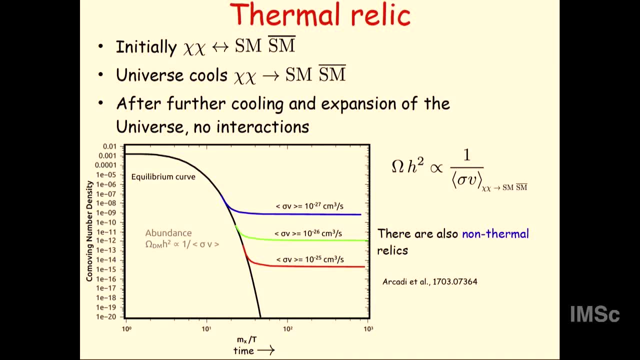 interaction that two dark matter particles producing strand-mold particles and the expansion of the universe. Once the expansion of the universe dominates, this interaction effectively stops And the number density technically is called freeze out. That means it stops. The number density is known. 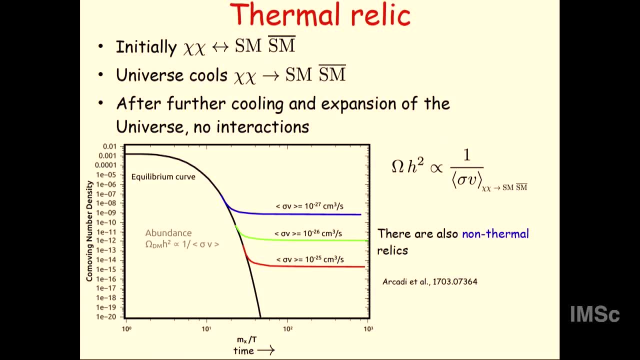 All right, So that is how you can reproduce the correct dark matter relic density. All right, This is, as I said, this is one way to do it. There are various ways to do it And actually something funny here happens. The funny thing is as follows: As I said, you can do this calculation. sorry, 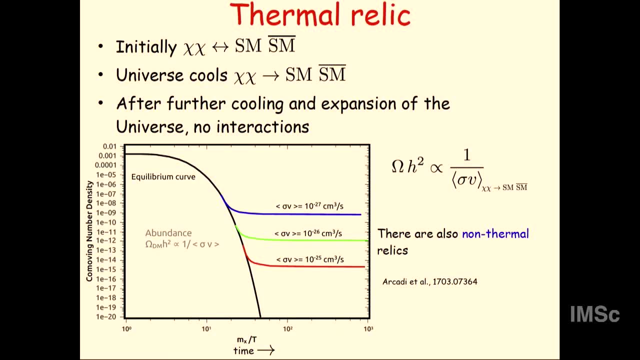 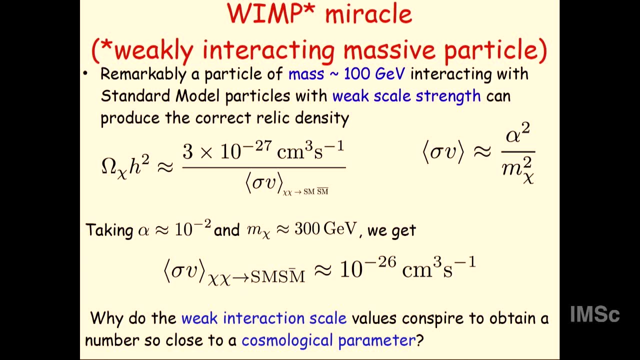 you can do this calculation in great detail. You will find that the dark matter particles are. density is inversely proportional to the this annihilation cross section. you can do this in more details and you get a number like this: all right, the the dark matter density in this. 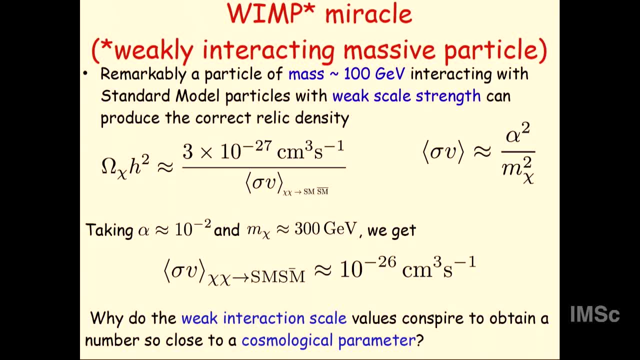 dimensionless units, is this number divided by the annihilation cross section of dark matter particles adding to standard particles. there's a v here, which is the velocity, relative velocity, and then you, you do this velocity average with these things all right. in very simple particle physics models this thing, this number, can be written as alpha square, where alpha is a coupling. 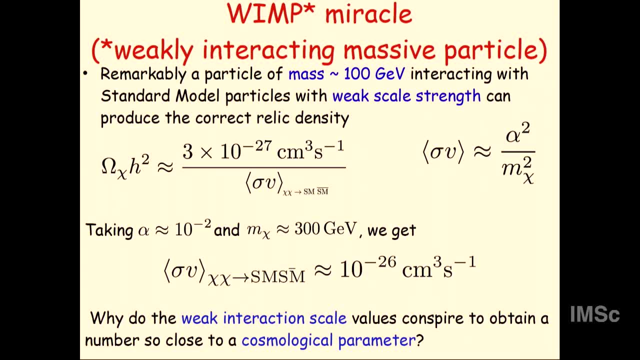 constant and the dark matter particle mass squared, m, chi squared. you put these numbers. take alpha is 10 to the power minus 2. that's sort of like the coupling constants that we know of. all right, you make the dark matter particle mass of 300 g. that's sort of like weak scale. 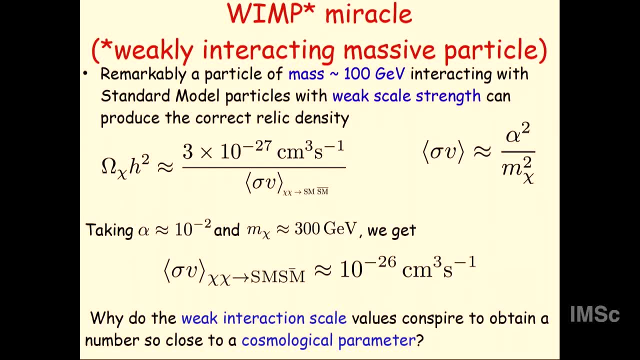 weak interaction scales, you get this cross section, which is 10 to the power minus 26 centimeter cube per second, which is astonishingly close to the number that you require. yeah, but you require this number to be 0.1, right? if you put this value in, you get 0.3, right, just just. 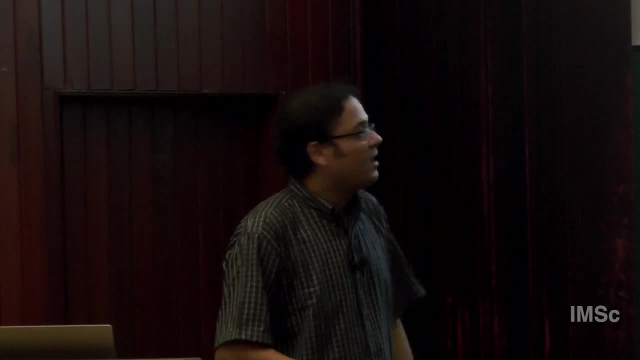 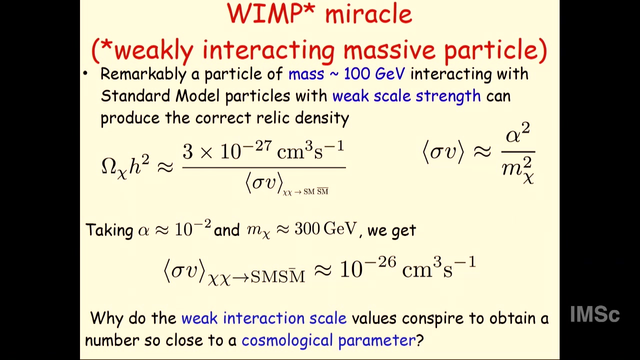 one back of the envelope calculation. you will suddenly get this number out and this is a profound mystery. these numbers, I told you, I gave you this example of these numbers. these numbers are sort of weak interaction scales. alright, weak interaction is beta decay. beta decay is weak interaction, right? 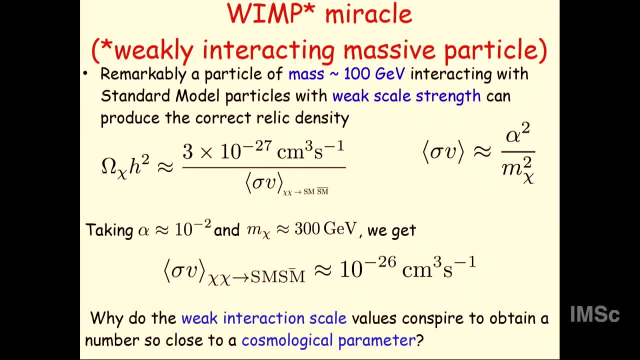 these numbers are weak interaction scale numbers. how come I use these numbers and suddenly I get a number which is in cosmology? weak interactions have nothing to do with cosmology, by the way. what is the knowledge of magnitude of part? so this is actually called the WIMP miracle. 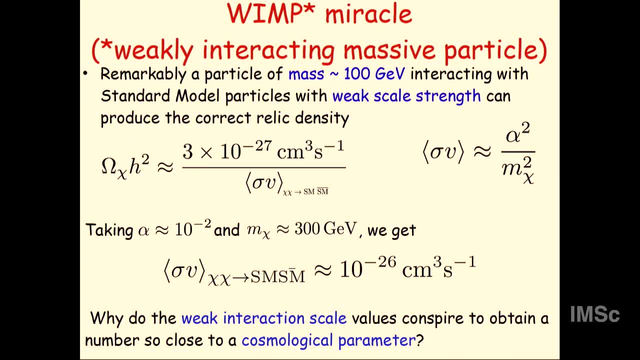 weakly interacting massive particle. how come we take numbers from particle physics? we write them in the proper units, right? I just write it in terms of units for this. you don't have to do any. any Feynman diagrams, nothing by dimensional analysis you will get this thing. this is how. 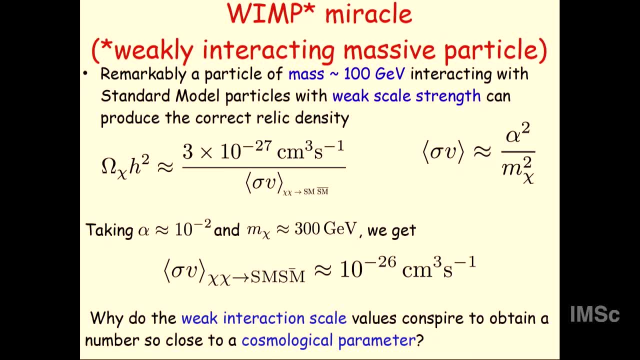 it will work. if you just take weak interaction numbers, do a dimensional analysis, you suddenly get the correct answer. this is absolutely an astonishing thing. the question is why we don't know the answer. alright, so this is one way, as I said, but there are also other ways to do it. 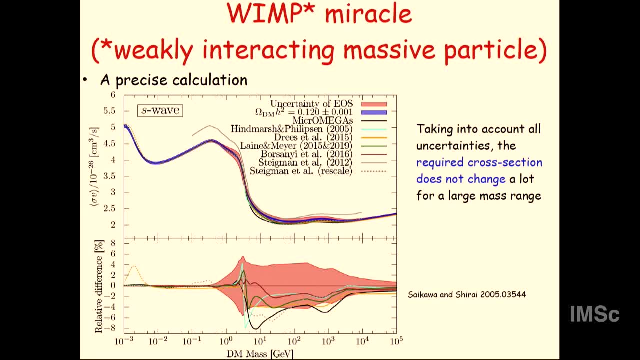 so this is again a more precise way to do the whole calculation right, and this is taken from this paper. what is plotted is the dark matter mass on the x axis and just look at this plot. and what is the sigma v required? alright, you can, to get the correct relic density. 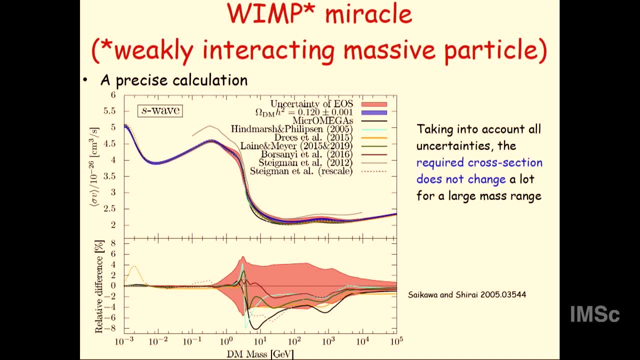 alright, you see, it is not. doesn't change much. depending on this, x axis changes by 8 orders of magnitude. alright, this sigma v. so whenever you are on this line, you reproduce the correct dark matter density. this changes from 5 to 2. factor of 2. 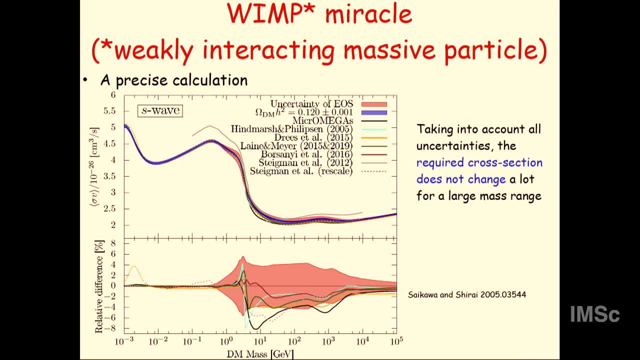 within 5 orders of- sorry, within 8 orders of magnitude. this cross section changes by a factor of 2, and yet you get the same answer. this is by doing the same calculation in a more precise way, right? this is the astonishing thing. why does this happen? 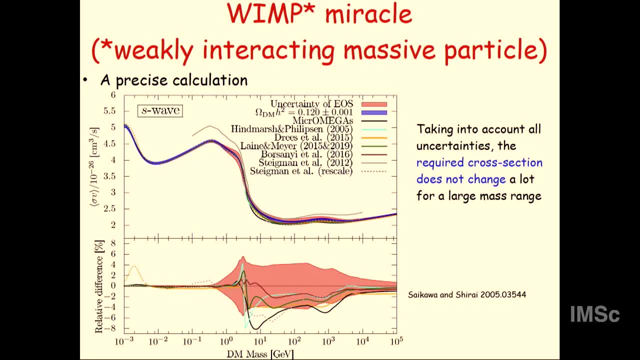 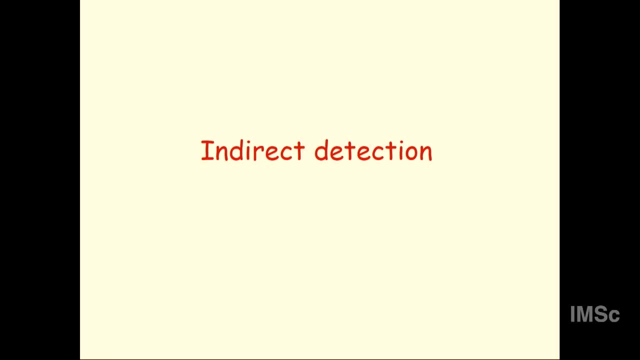 we don't know the answer, alright, and there is something which we try to find out, ok, good, so now that I have told you, remember, this is one way to find out dark matter, I mean, how do you detect it? again, there are various ways to find out dark matter. 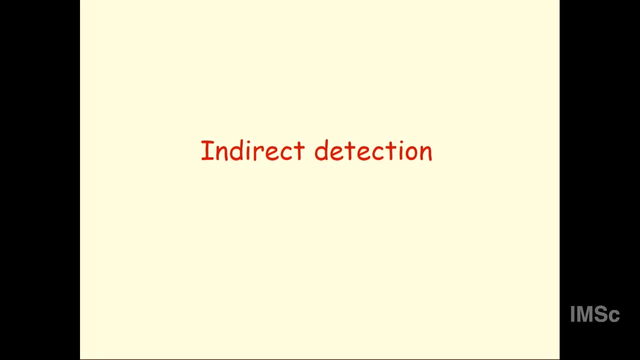 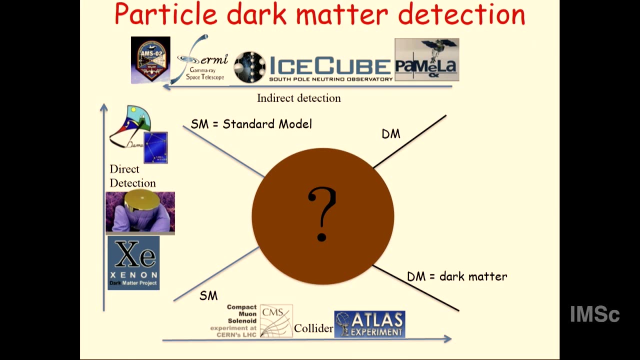 there are various ways to detect it. I will be talking about indirect detection. so what does indirect detection mean? indirect detection means as follows: suppose you draw this cartoon Feynman diagram. alright, sorry for which, correct, correct, and this is actually the sort of this slide is good. 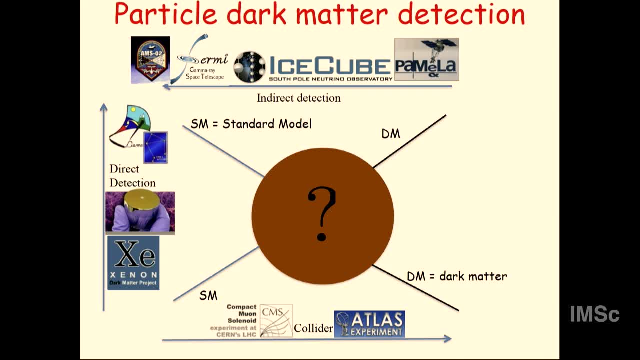 so this is a cartoon, Feynman diagram. alright, you don't need to know anything about Feynman diagrams to understand this cartoon. so there are two standard model particles in the asymptotic state- it can be initial state or final state- and there are two dark matter particles. 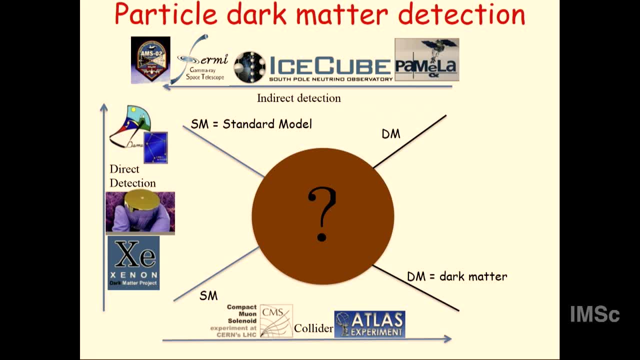 at the asymptotic state. it can be both initial state or final state, right, depending on which way you look at the picture, you can detect dark matter. so let's look at what LHC does. what does LHC do? LHC tries to collide two protons. 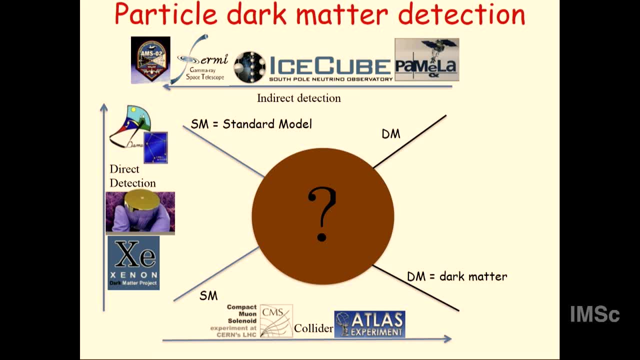 and produce dark matter. so LHC does that. the diagram goes this way: right, that means you collide two dark matter, two standard model particles, two protons and you produce two dark matter particles very roughly. alright, I mean, there are other signatures, but anyways, I can discuss in detail. 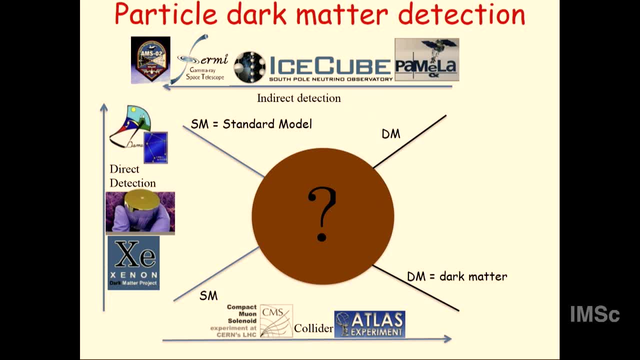 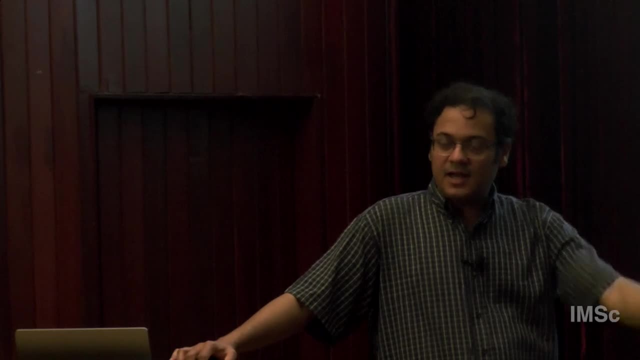 this is how LHC works. alright, all these LHC collaborations. this is called in collided production of dark matter. there is direct detection, which I will not talk about. what does this do? in this, what we do is we keep some low energy. we keep some detector in an 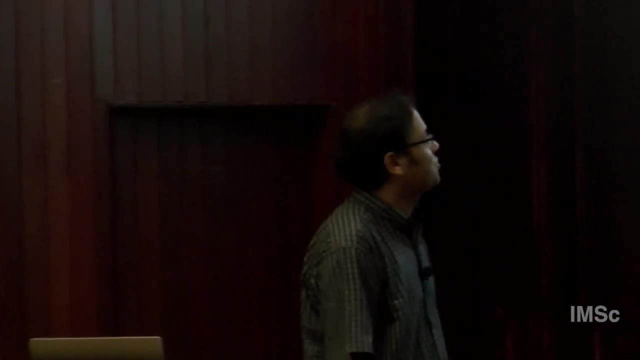 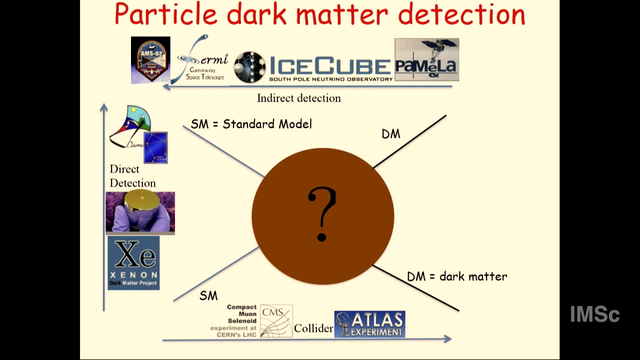 background: free environment. we try to make the background as low as possible. so that means this SM: some standard particle is there. we hope at some point a dark matter particle will come, will collide with the SM. so this SM will give you some signature and the dark matter will just go out invisibly. 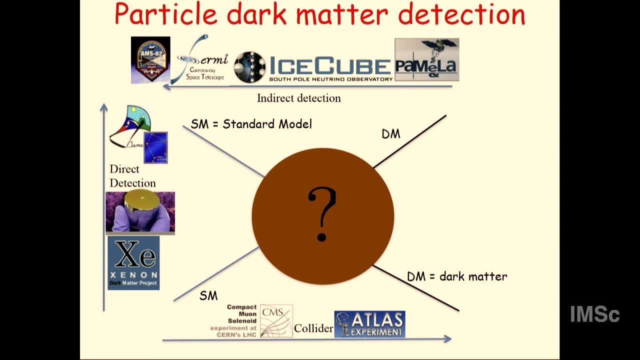 right, so there are various detectors, right? so this is something where condensed matter is extensively used to detect dark matter. alright, so you put in a dark matter. sorry, you put in a detector, various kinds of fancy detectors. you hope at some point a dark matter will come, will collide. 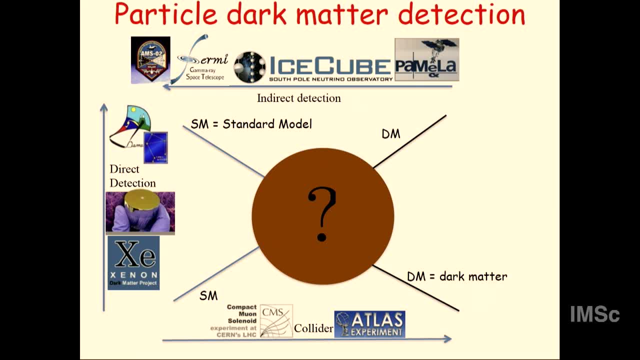 will hit the detector. you see some signature, ionization signature, phonon signature and various different things, superconducting signature and things like that. you see here, this is the final state and then the dark matter will go away invisibly. so the time goes this way, alright. 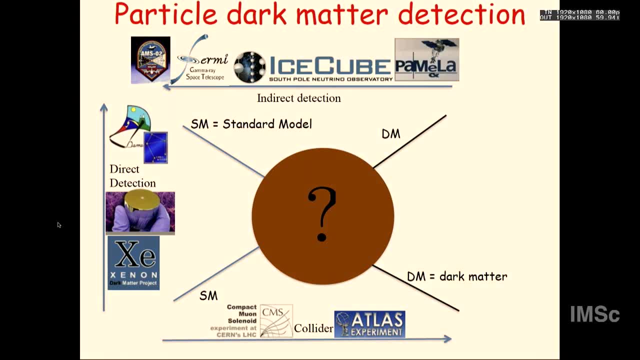 oops and finally, what I will be talking about is indirect detection. what does indirect detection means? remember, I have been telling you that there are lots of dark matter in the universe. it is possible that dark matter two dark matter particles, as I said, although remember, two dark matter particles. 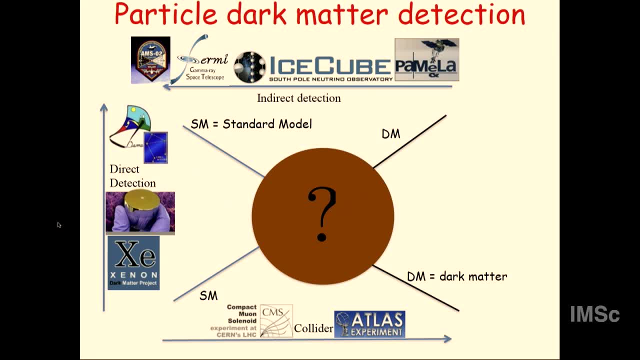 the collision has stopped. it does actually not stop entirely. there are some residual collisions happening, very, very few collisions. so that means two dark matter particles can collide and produce two strand wall particles. so this is the diagram going this way. alright, something else can also happen which is not given in this diagram. 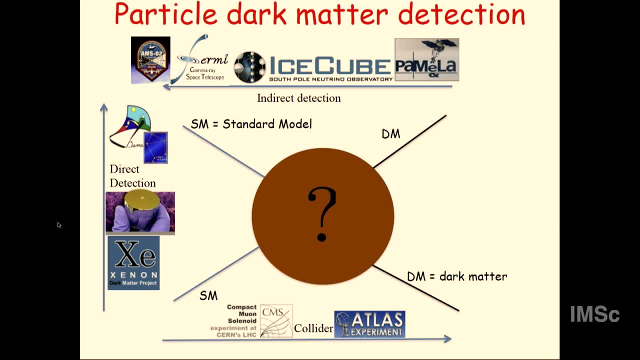 if the diagram, if the dark matter particle can decay, right, then there is one dark matter particle here and that will just decay to two strands of light. alright, two strand wall particles, and I will give you an example of that. alright, this is indirect detection. when this diagram 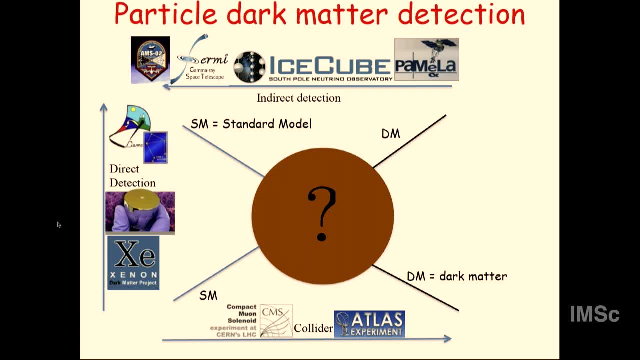 you look at this diagram. that is initial state: you have dark matter particles and final state: you have strand wall particles. that is indirect detection. collider is initial state. you have strand wall particles. final state: you have dark matter particles and direct detection is initial state. you have strand wall particle. 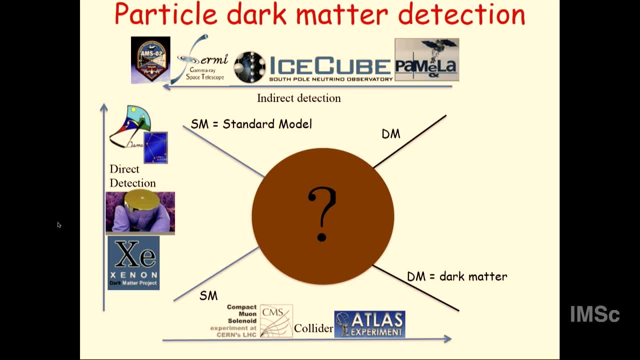 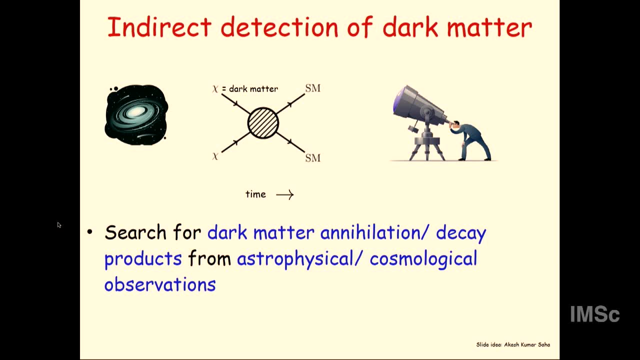 and dark matter particle. final state: you have strand wall particle and dark matter particle. that is how it works. I will give a brief description of this. alright, so what does indirect detection look like? so again, as I said, so what you do is you look at some astrophysical observation. 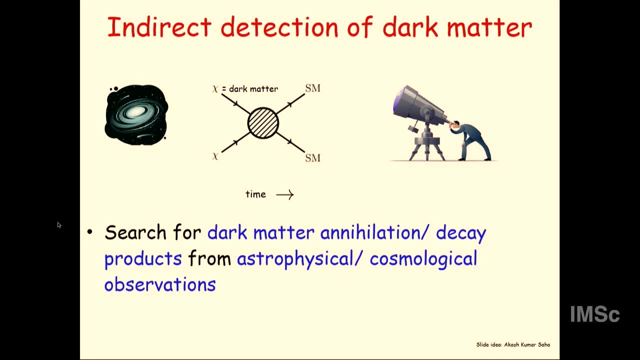 astrophysical or cosmological observation. you hope that two dark matter particles will collide, or a dark matter particle will decay to produce standard wall particles and you will observe that from the earth. that is what the hope is. alright, so you search for dark matter annihilation or decay products. 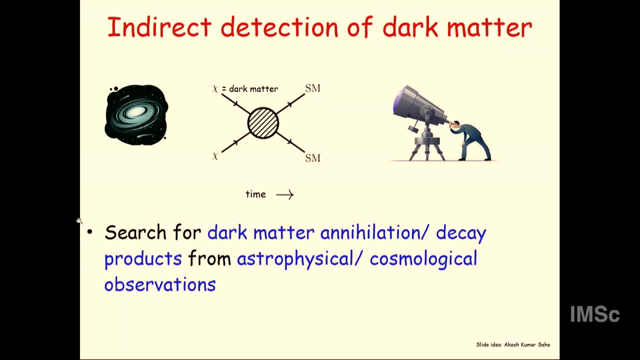 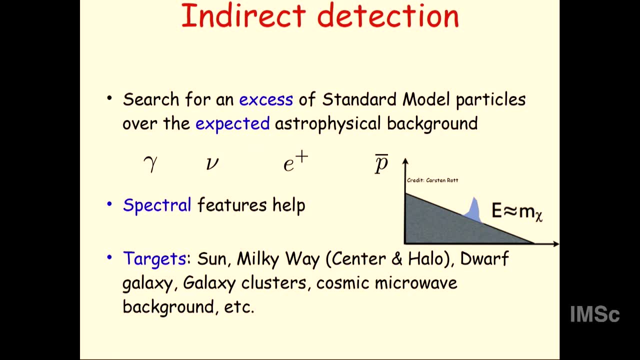 from various astrophysical and cosmological signatures, from cosmological observations. ok, so more precisely, what does that mean? that means you search for various dark matter particles, various strand wall particles over expected astrophysical backgrounds. alright, so we search for various particles: photons, neutrinos, positrons, antiprotons and various things. 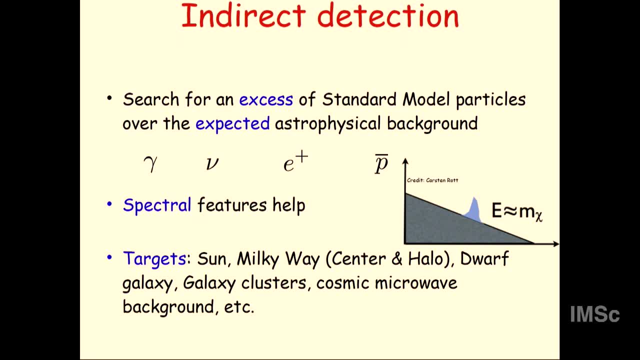 in cartoon way. what does this mean? what it means, is this cartoon alright? in the x-axis what is plotted is the energy, and y-axis is plotted is some particle flux. it can either be neutrinos or it can be photons. neutrinos, positrons, antiprotons. 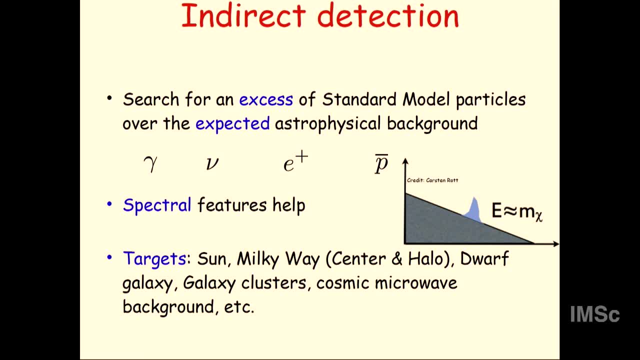 the astrophysical background will look like this, something like this: alright, and we hope that some point we will find excess of these particles due to dark matter annihilation or decay. this peak, and there are kinematic reasons why this peak- cannot be mimicked by astrophysics. 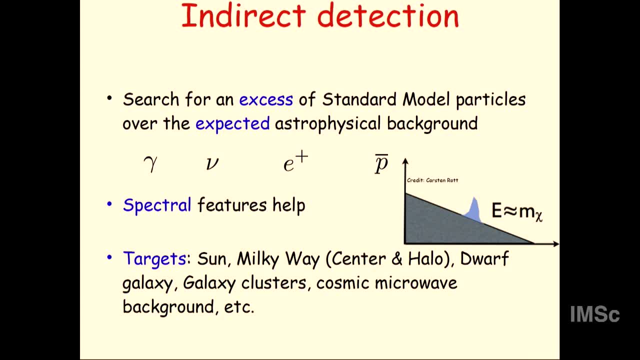 almost always. but again, and to do this we look at various objects. we look at the sun, the milky way, dwarf galaxies, galaxy clusters, cosmic microwave background, various different things. we just look at anything that we can observe, anything that you can observe, and try to find it. programming zweiten, and he can seeした. 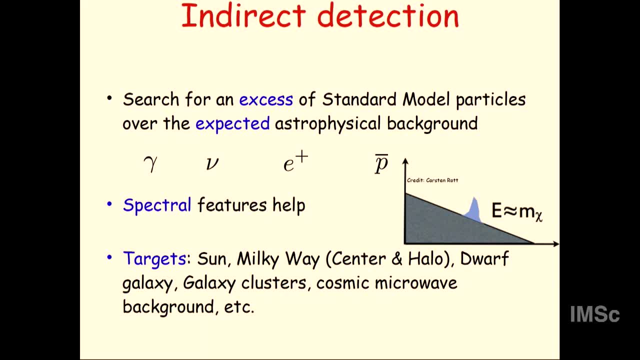 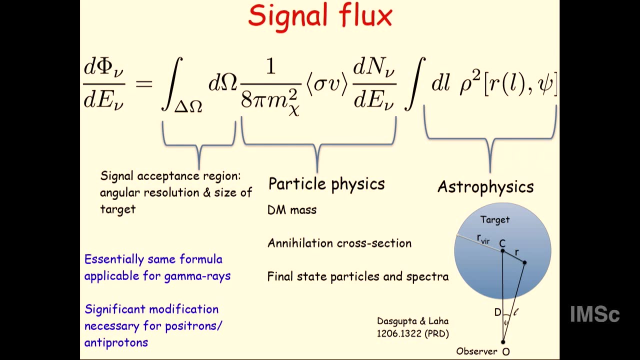 find the signature all right. and, as I said, I mean there is also some spectral features. spectral feature means this thing is called a spectral feature. the feature, the spectrum is different, the energy spectrum is different. all right, So how does this signal look like? This signal looks like: so this is actually for neutrinos. 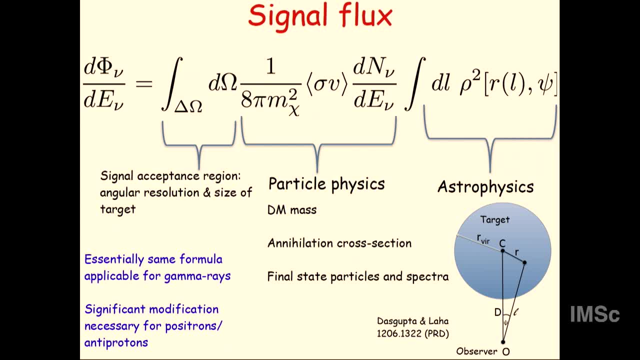 and I am plotting it. I am telling you the flux of neutrinos from dark matter annihilation, just because it is the simplest to do. it depends on how much sky you look at: d, omega, right. it depends on some particle physics inputs. what is the annihilation cross section? 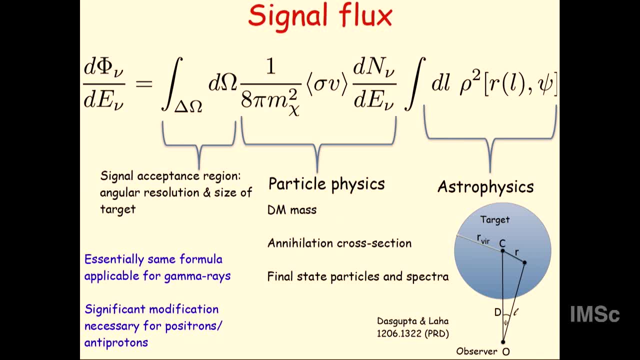 what is the dark matter, particle mass and what is the neutrinos spectrum from that interaction? and it depends on how much dark matter is there in your line of sight. all right, So bottom line there is. I mean you do not need to go into the details of the interaction. 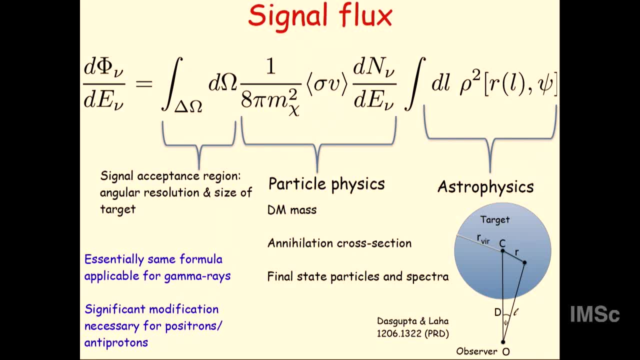 of this equation, what it depends on. it depends on particle physics, which tells you what is the dark matter, mass Right, What is the annihilation cross section and what is the final state- dark matter, what is the final state standard model particles, and it depends on astrophysics that what is the 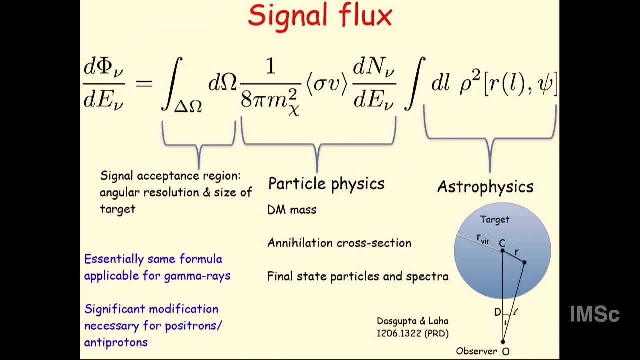 density of dark matter, as was asked in some object. all right, So you look at some object. all right, this is, this is your observer. you look at some object, you figure out this integral like this from here. all right, Essentially, the same formula is applicable for gamma rays. all right, there are important. 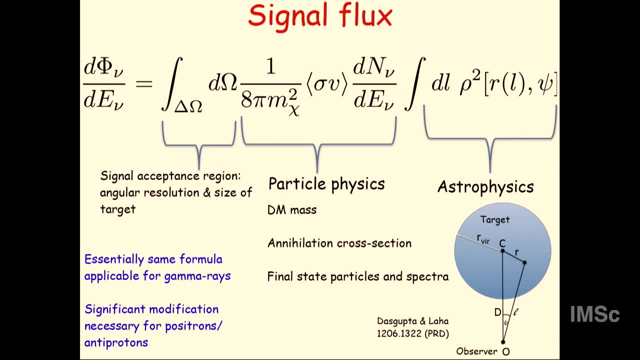 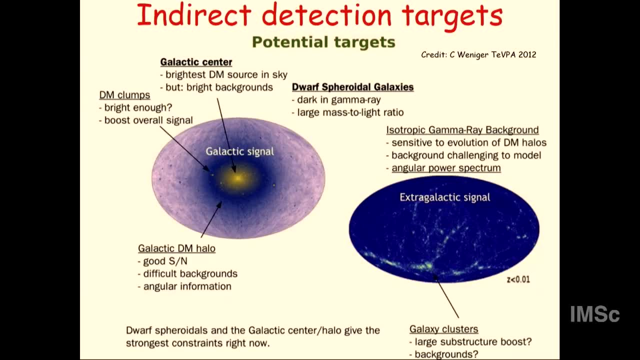 modifications again, which I cannot go into now, but I can tell you more if you are interested- and there are. There are also other modifications required for positrons and antiprotons. ok, So what do we look at? as I said, this is, this is a picture. we, as I said, we look at everything. 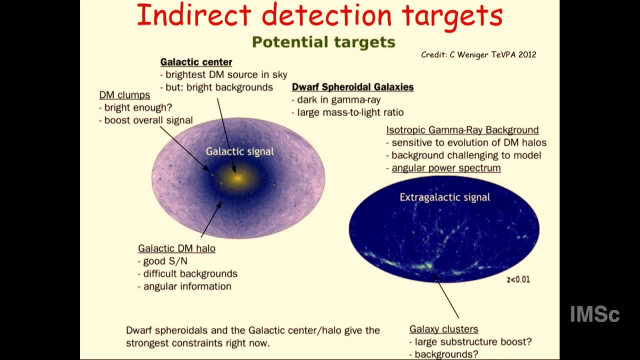 by the way we look at. so this is sort of like: this is the galactic center, this is how the galactic signal will look like. we look at extra galactic space. we look at dwarfs, galaxies, we we look at galaxy clusters. we look at everything right, we look at whatever we have. we look 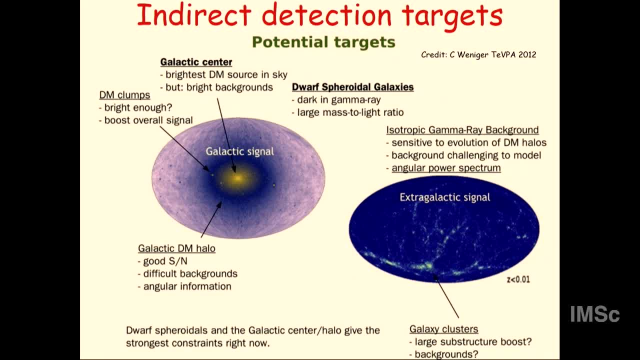 at it, and all of these have some advantage and disadvantage. all right. For example, let us let me talk about two different things: the galactic center and dwarf galaxies. So galactic center is the brightest dark matter source in the universe. sorry, in the sky, oh. 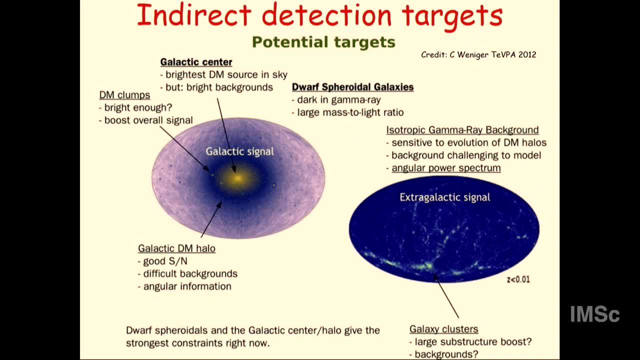 yeah, in the universe, what from what we observe? why? because it is very close, it is a flux argument: 1 over d squared. it is super close, it is very bright, but there are lots of things in the in the galactic center. it is very difficult to entangle, disentangle the signal from background. 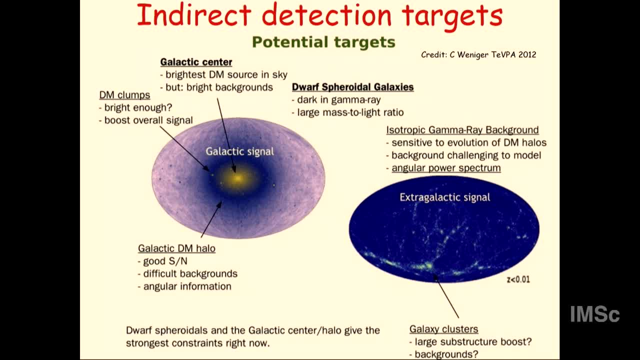 all right, So there is a pro, but there is a con For dwarf galaxies. Dwarf galaxies Are quite far away, all right, so their flux is low, but they do not have much astrophysical production, astrophysical backgrounds, so that is an advantage, right. 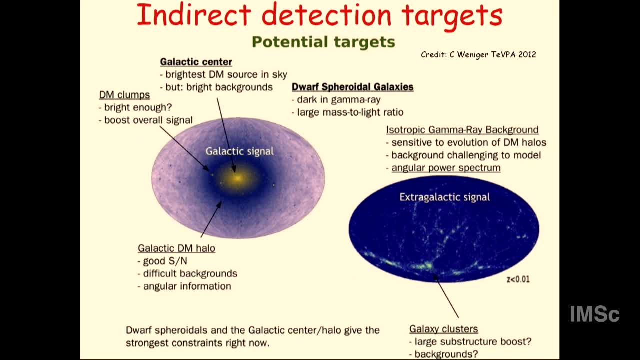 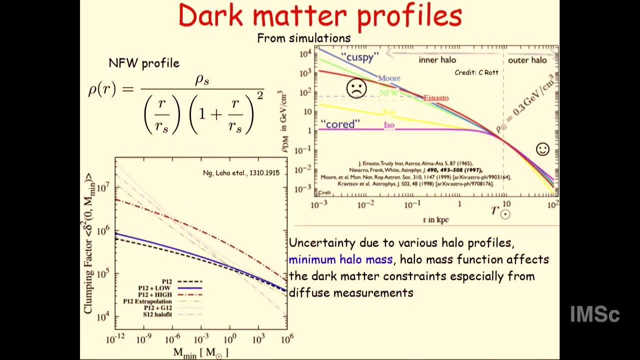 So this advantage and disadvantage is there in all of these things. I can go over all of this, but let me not go over. but if you are interested, please ask me. I will be happy to talk more about all of these things. all right, And this comes to the question that was asked: what is the dark matter? density in, say, a typical. 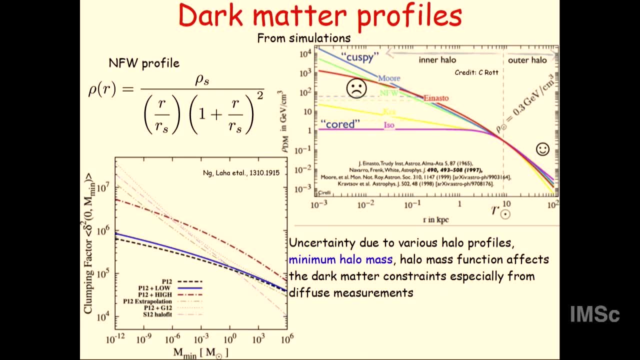 galaxy. This is what is plotted. This is the dark matter density in the milky way. all right, This r is the distance from the center of the milky way. all right, And this is the dark matter. density in GeV per cubic centimeter on the y-axis right. 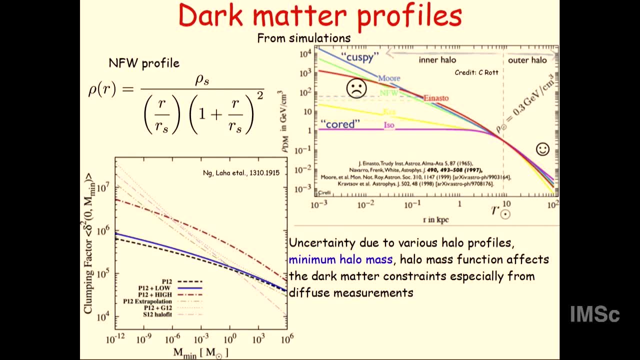 We are roughly at 8 kilo parsecs from the center of the galaxy. The sun is roughly 8 kilo parsecs from the center of the galaxy and there we know the density very well. as I said, we know it to 20- 30 percent accuracy. 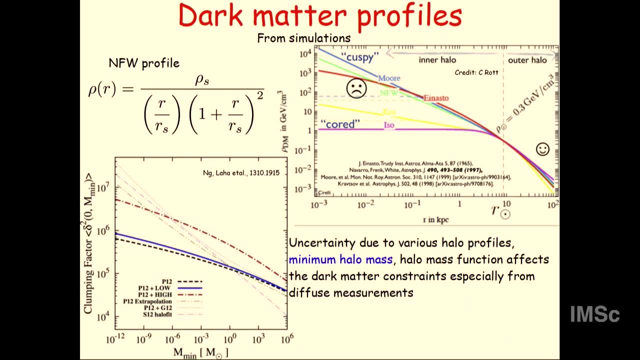 So so, so so. so all of this measurement should coincide here. But what is it At the center of the galaxy is something we do not know right. It's extremely unknown Why. Because at the center of the galaxies the mass budget, then the amount of mass, is dominated. 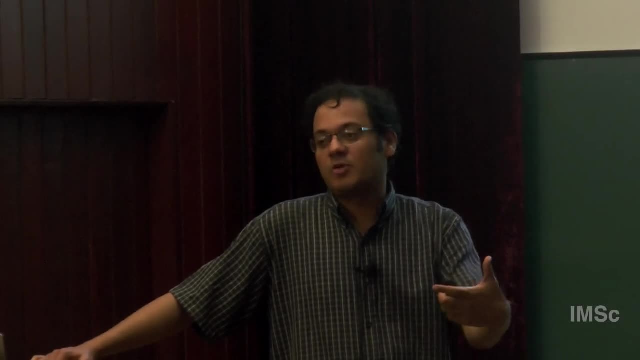 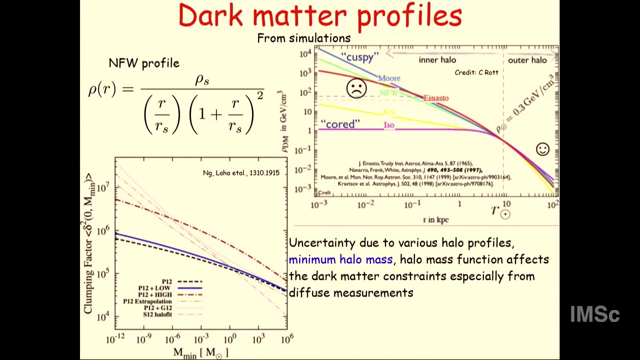 by baryons, that is is dominated by standard model particles, is not dominated by dark matter. Dark matter starts dominating only when you go, say, beyond one or two, one or two kilo parsec. That's why it used to. dark matter starts dominating. 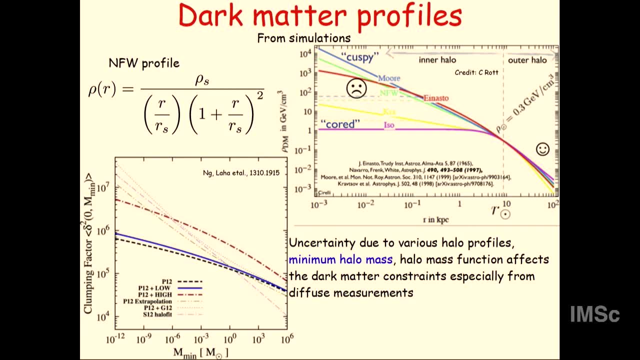 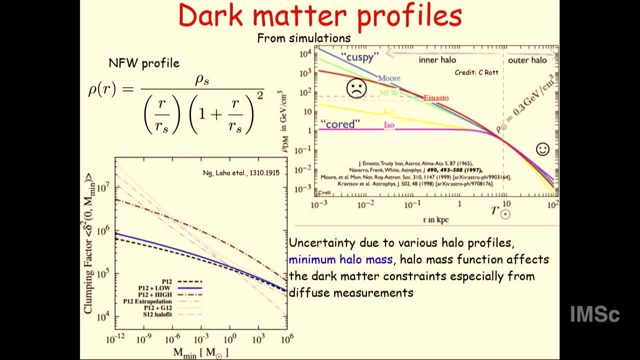 That's what this thing. That's why for the dark matter density is huge uncertainty. We have literally no idea. So the smallest distance from the galactic center where we have some measurement of the dark matter density is roughly one kilo parsec. 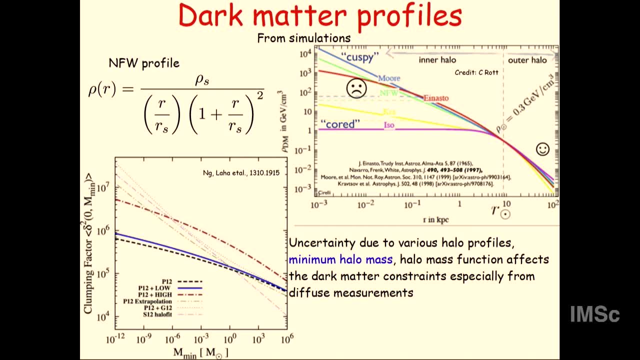 So say roughly here. Good, So dwarf galaxies have a size of roughly one kilo parsec. So again you have to rescale this figure. But this actually is sort of true in the sense that once you go near the center of the dwarf 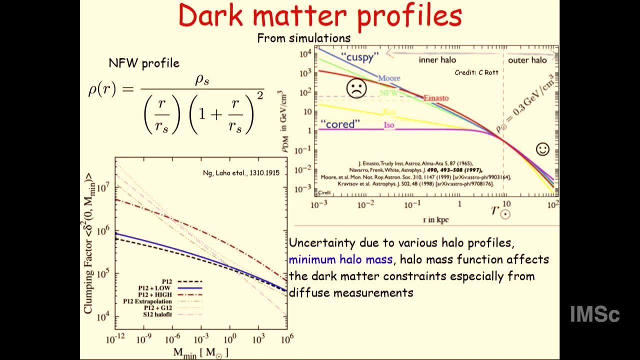 galaxies. their center means 0.1 kilo parsec roughly. There is huge uncertainty in the dark matter density Far away. this is well known. This is almost always true And this comes simply from very standard physics. Let me tell you, since the question was, let me tell you the physics. 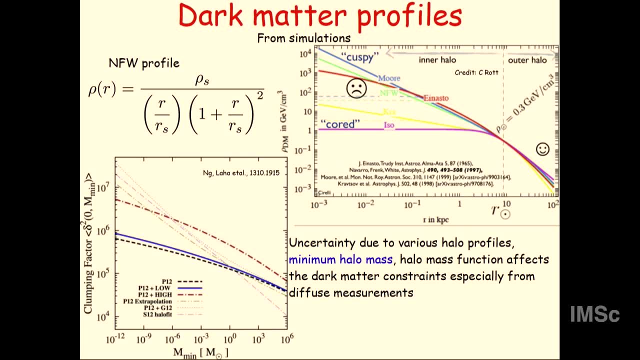 Anything that we know. like all standard world particles, we lose energy and we know, once it loses energy, it will just clump together. This is, remember this losing energy is going around and clumping. Dark matter does not lose energy, All right. Dark matter does not radiate. 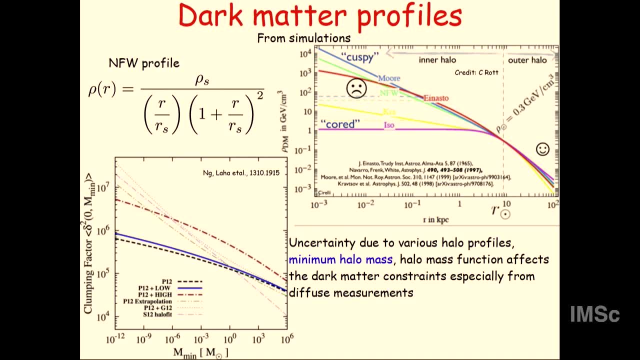 That means dark matter does not connect to photons directly, So dark matter cannot clump, So dark matter remains diffuse. That's what the argument is Right. I mean, that's a very simple way to understand it. You can do this thing. 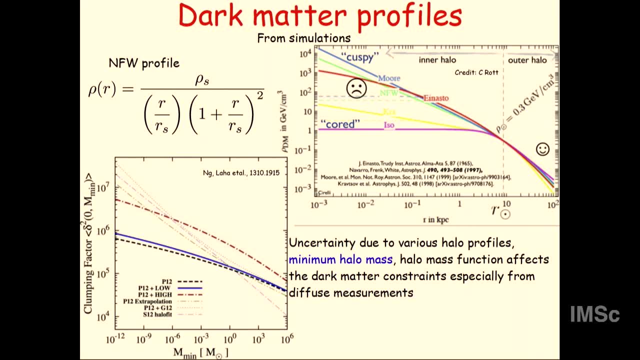 But all these simulations- remember, all of these things are coming from simulations. There is some data from here onwards, From roughly one kilo parsec onwards, there is some data. There is actually lots of data: One kilo parsec, So you can do all of these simulations. 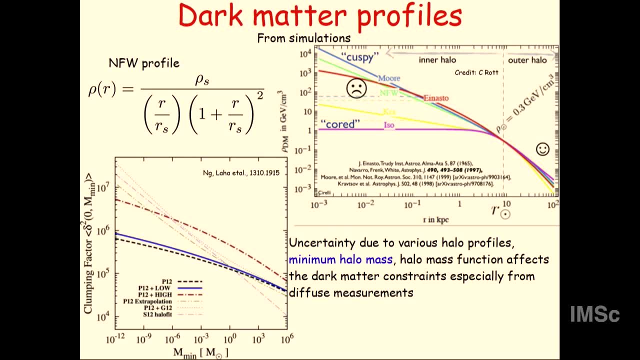 That's what the simulations are doing. I mean, you can do very fancy simulations, but the point is as follows: Everything that we know, like we can see, connects to photons, And then they lose energy and they clump, Whereas dark matter does not connect to direct, does not directly connect to photons. 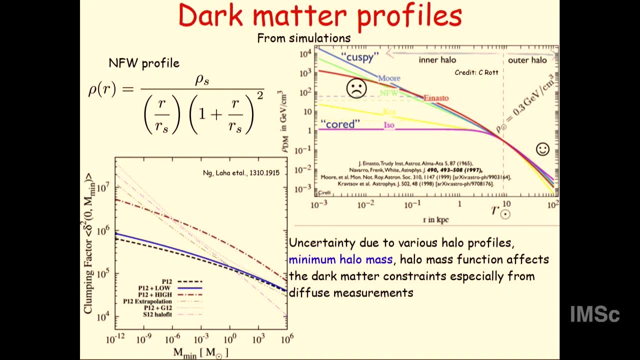 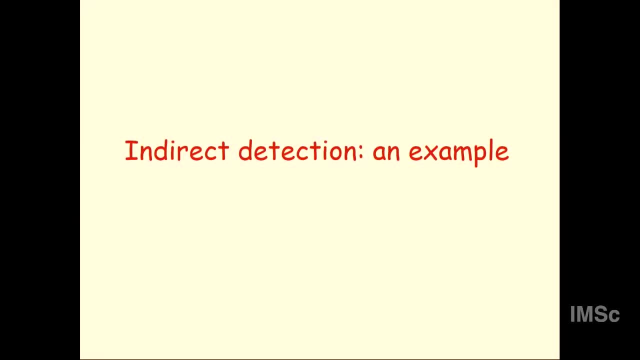 So that's why they cannot lose energy, They just remain diffuse. All right, So let me skip this plot. This is a bit more thing, But let me give you an example of indirect detection. All right, So there's probably five minutes left. 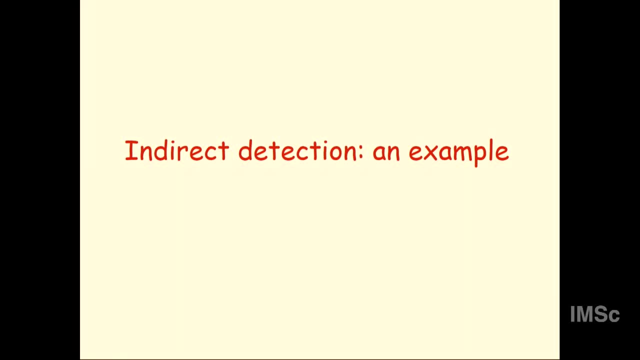 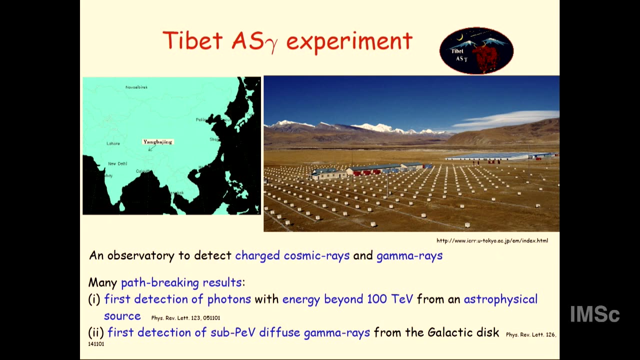 Right, Five minutes left, Yeah, So let me give you an example of one thing And I'll tell you something which is absolutely current. One month earlier, what has happened in dark matter, indirect detection- So let me now. I've been talking about dark matter, dark matter, dark matter. 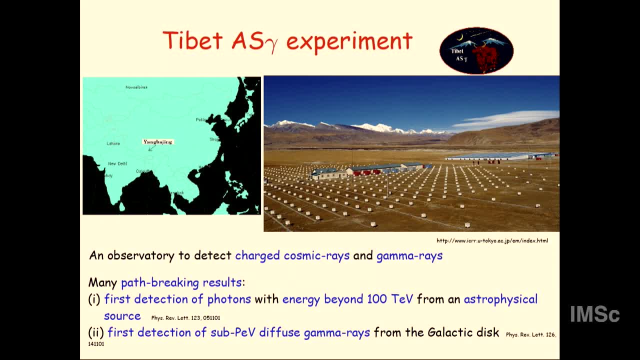 Let me talk about something completely different: Gamma ray astrophysics. How does the universe look in gamma rays, All right, And then tell you how it connects to dark matter? This is again a field by itself. It's like there are people who want to look at how the universe looks in gamma rays. 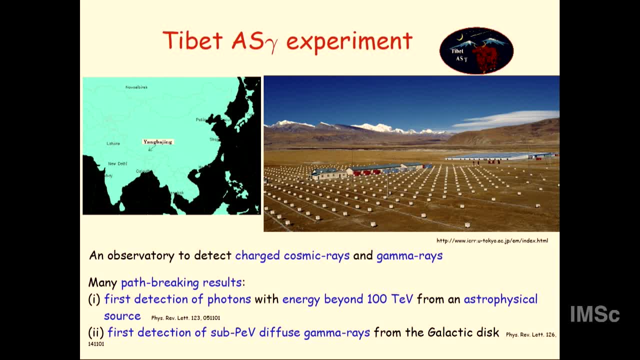 And we actually don't have much idea about it, by the way. All right, So one of the experiments that I'll be talking about- there are many experiments- is called the Tibet A-S gamma experiment. This is an experiment in Tibet Air shower. 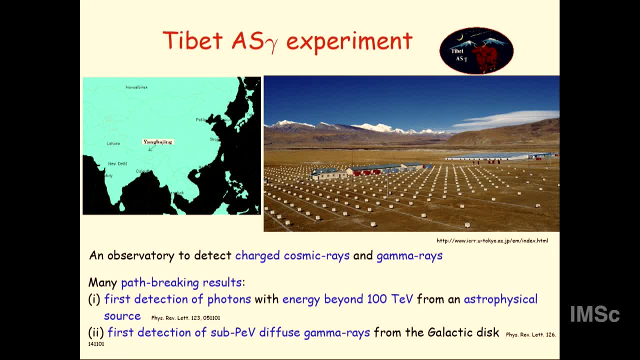 So A-S means air shower. Gamma is photons, Right. This is in this Yang-Bajing plateau. This is how the experiment looks like. This is an observatory to observe charged cosmic rays and gamma rays, Right, And I mean, ask me later how they do it and I can discuss how they do it. 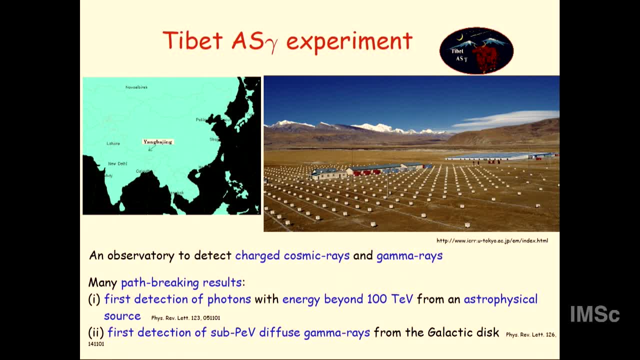 So Tibet A-S gamma has got some path breaking results over the last two, three years. So the first result that they got is that they detected. This is the first photons with energies beyond 100 TeV from an astrophysical source. All right, 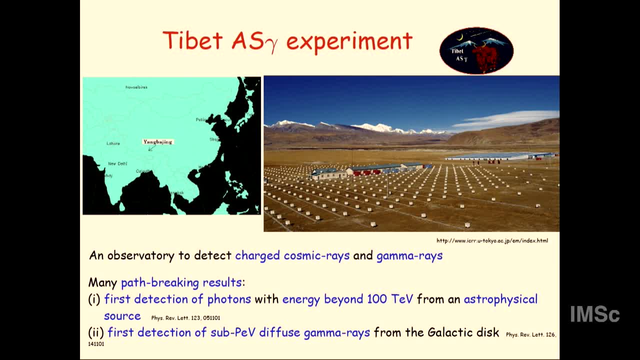 Just to give you a scale: One GeV is the mass of the proton. One TeV is 10 power 3 GeV. So this is five orders of magnitude more energetic than the proton. This was the first of the. This is the first observation. 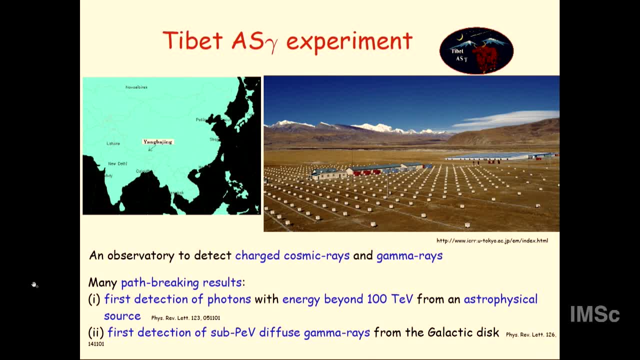 This is published here All right, From an astrophysical source. From some source, It actually discovered these photons We had never Before that. This is in 2019.. Before that, We did not know how the universe looked like in 100 TeV energies. 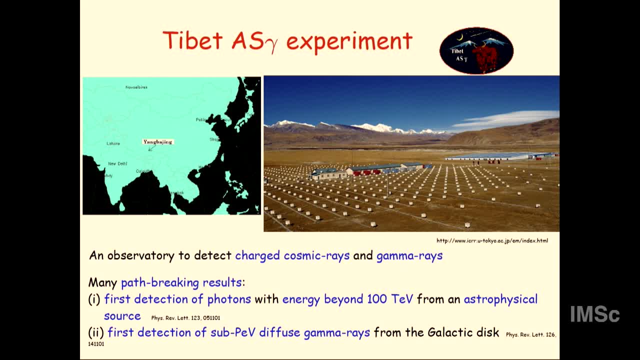 We had no idea, Zero idea- Right In 2021.. Last year They discovered sub-PV diffused gamma rays. I'll tell you what sub-PV means. PV is 10 power- 6 GeV. Right Peta electron volt is 10 power- 6 GeV. 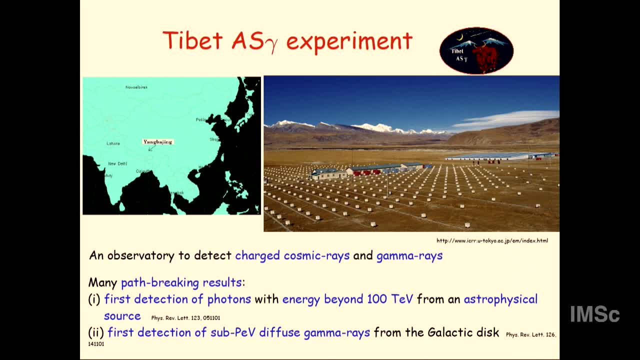 And sub. I'll tell you what is the energy range. I'll show you Right Sub-PV. Diffused gamma rays from the galactic disk. All right, And I'll tell you what is diffused gamma rays and what is galactic disk later. 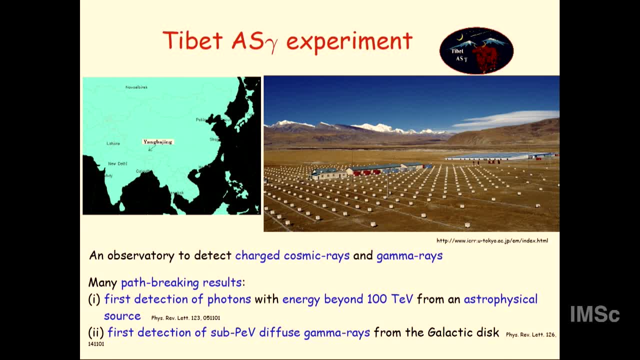 All right, This is also the first observation. All right, Remember, This is the first observation. All right, Remember, This is the observation from a single source. This is the observation. This diffused thing is not from a source. It's from parts of the galaxy which are not in an astrophysical source. 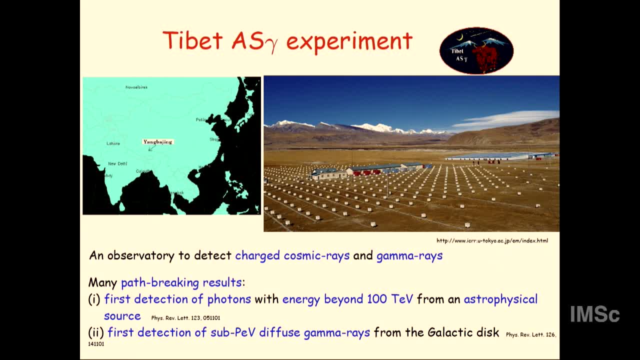 Okay, These are like two path breaking results. They have got it. All of this is completely gamma ray astrophysics Right, And I'll be happy to talk more about it And later connect it to dark matter. So let me talk about this. 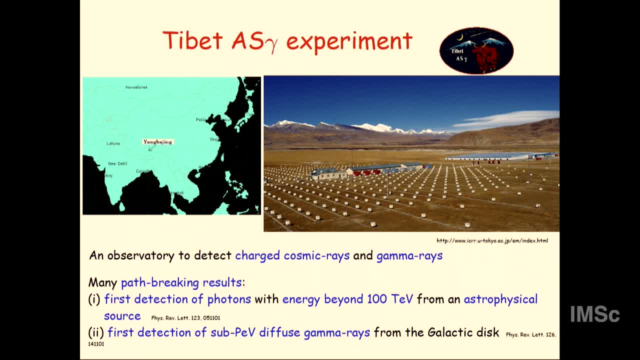 This first detection of sub-PV diffused gamma rays from the galactic disk. All right, So this is a cartoon impression of the galaxy, Right, If you look at this? This is the first time. This is the first time. 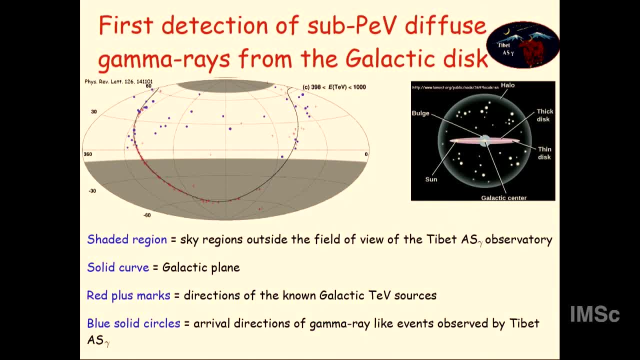 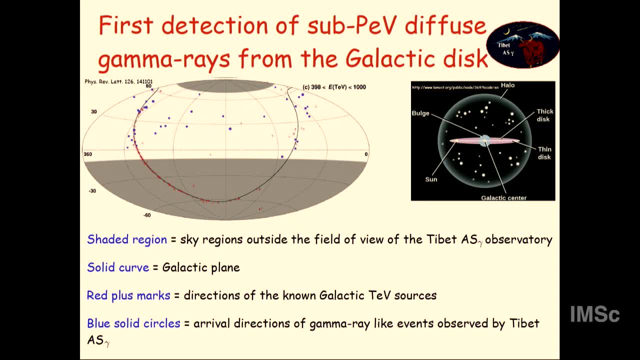 All right. So this is a cartoon impression of the galaxy. Right, If you go again far away from the galaxy, take a side run picture. This is the galactic center. This is the galactic bulge. This is the galactic disk. 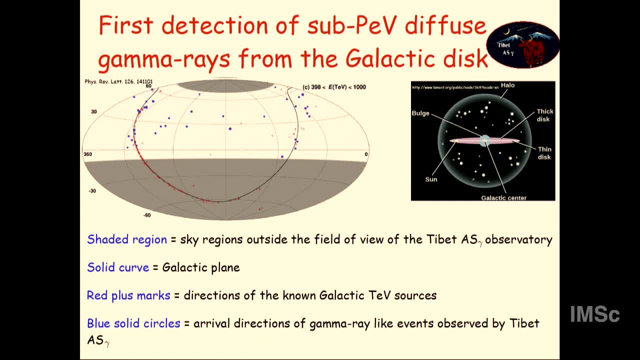 There is a thin disk and there is a thick disk, All right, And there is a halo, dark matter, halo around it. This disk and this bulge have lots of protons in them, All right, And the remaining thing is sort of galaxy, sort of empty. 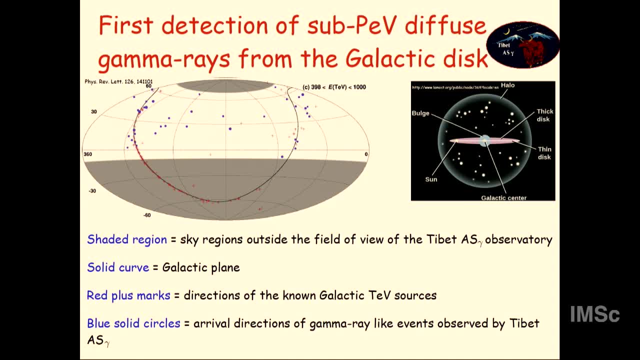 All right. So this is a map of photons from 398 TeV to 1000 TeV. right. 1 TeV is 1000 GeV. right. This is sub-TeV, It's just slightly less than a TeV. 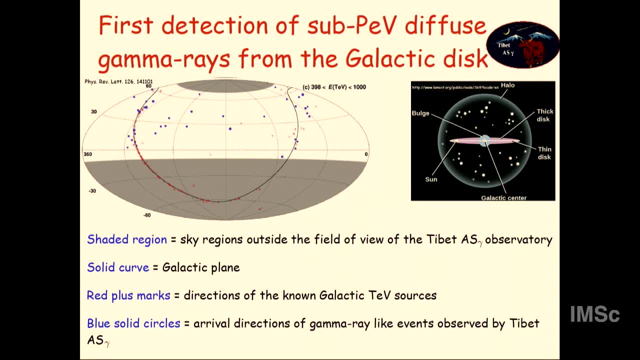 1000 TeV is 1 TeV. all right, So this is the galactic disk, This line that you see is the galactic disk, all right, This line, this thing, you plot it in fancy coordinates. It is basically this line, all right. 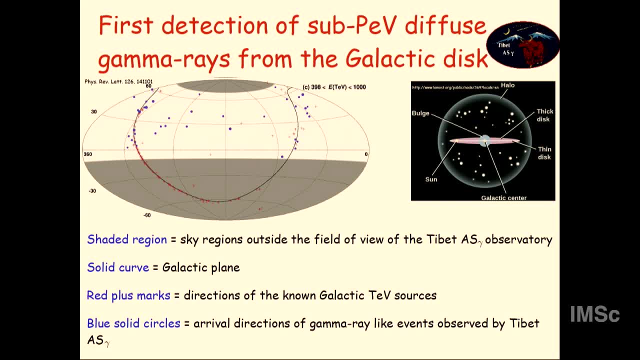 However, this is a map of what the universe galaxy looks like from the TeV to AS Gamma. all right, Anything that is shaded is something which TeV to AS Gamma cannot observe. all right, Because, say, for example, you are in Madras, Chennai. 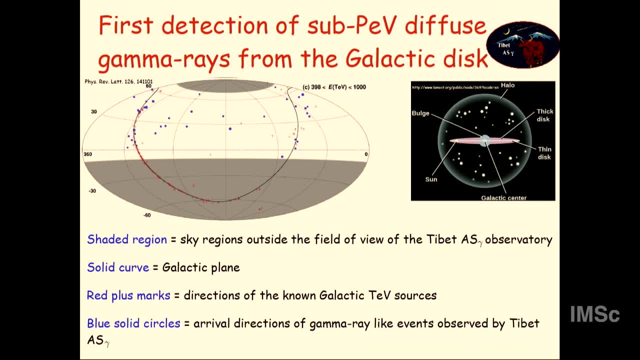 You try to observe the sky, You cannot observe the full galaxy or the full sky because at some point the Earth will stop you. The Earth will right. You cannot observe something like this, for example: You can do this for the whole year. 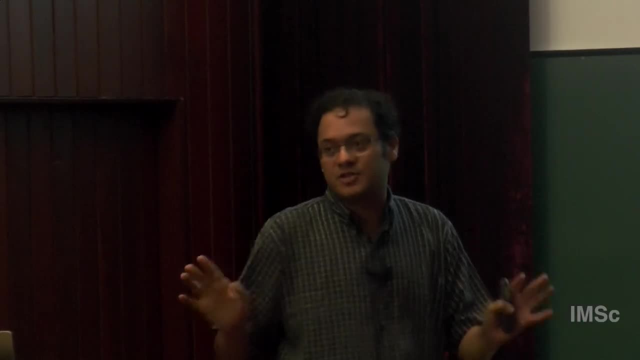 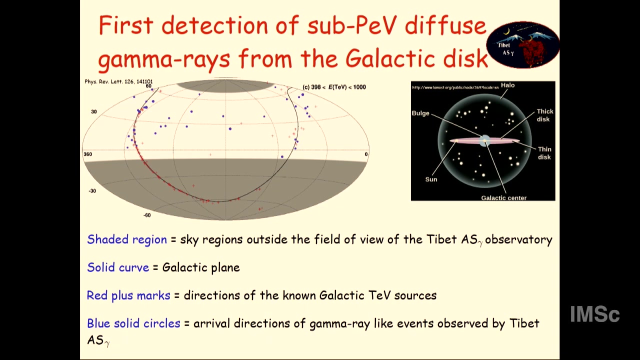 For many years you will not be able to observe some part of the sky from any location of the universe, Of the Earth, From Tibet. these are some locations you cannot observe, So they just grade it out, all right. So this plus mark that you see, this red plus marks, these are directions of known galactic TeV sources. 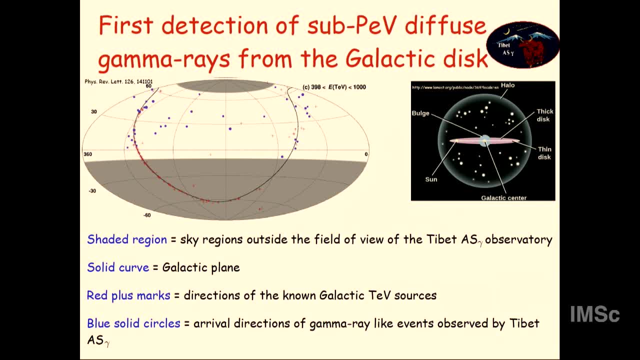 These are all measurements from other observations. right, There are many other telescopes. They have measured TeV sources coming from these plus marks. all right, You see, most of them follow the galactic disk. by the way, This is a. 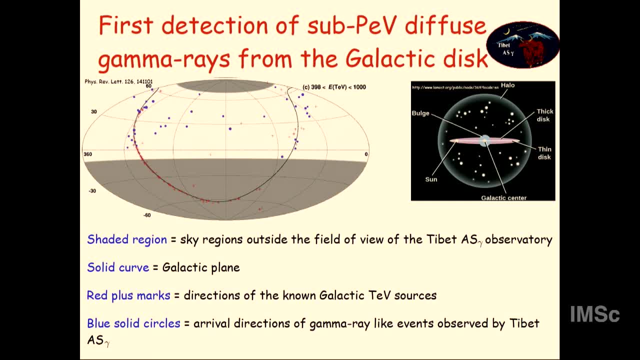 This is gamma rays, right, This is gamma rays. No, galactic sources, but not in TeV, or No, no, no, These are in gamma rays. Everything I am talking about is gamma ray. all right, These blue solid circles that you see are arrival directions of gamma ray-like events by the Tibet AES gamma. 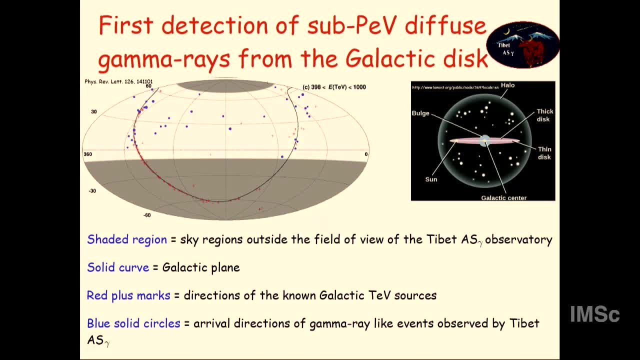 The astonishing thing is, you see, most of the blue circles follow this galactic disk, near this galactic disk, all right. And the other astonishing thing is, you see, you can do a statistical analysis. None of these blue circles coincide with this red crosses. 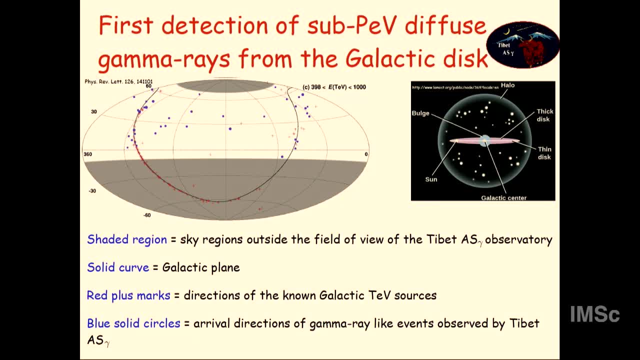 None of them cross it. So that means something is producing photons at these energies, but not producing photons at TeV energies. When I say TeV, it means 1 to 10 TeV. That's what TeV means. all right. 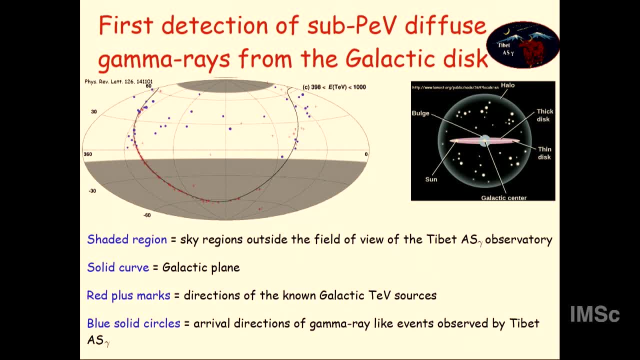 As I said, this is an astonishing discovery by Tibet AES gamma right. This is a discovery which gamma ray astrophysicists have been trying to do for the last 50 years, and they finally did it in 2021.. All right. 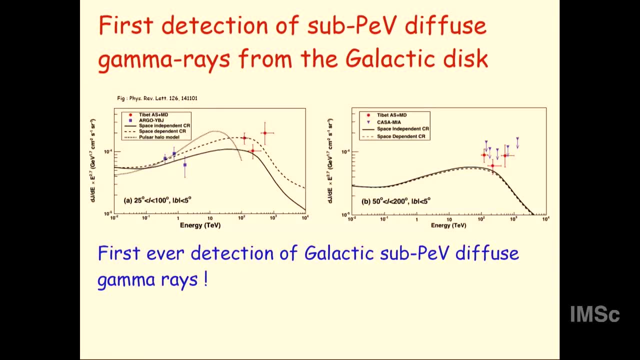 Good. So this is the spectrum. I'm almost near the end of the talk if you're impatient. So this is the energy of photons in TeV. all right, This is the flux of photons, all right, Multiplied by energy to the power 2.7.. 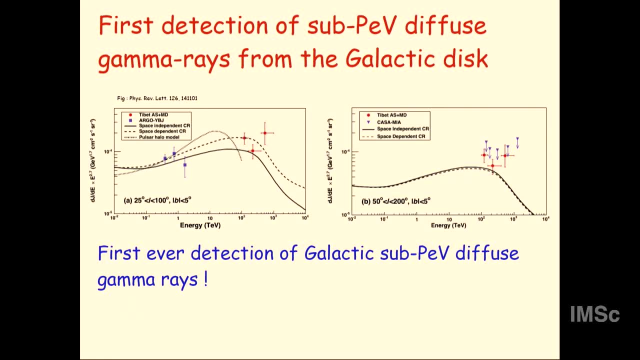 Some fancy ways to do it, but this is the flux of photons. This is a galactic latitude and galactic longitude. So we basically take the galaxy, divide it into latitude and longitude, just like the Earth. This is the galactic longitude and this is the galactic latitude. all right, 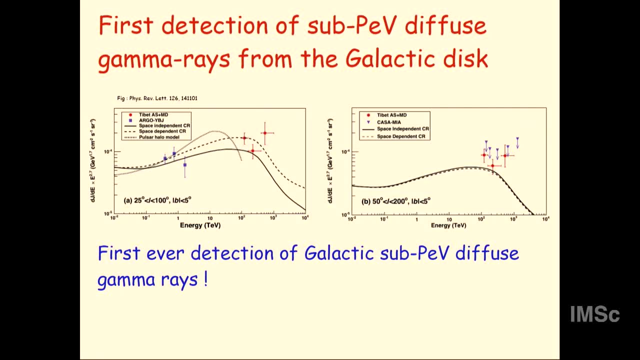 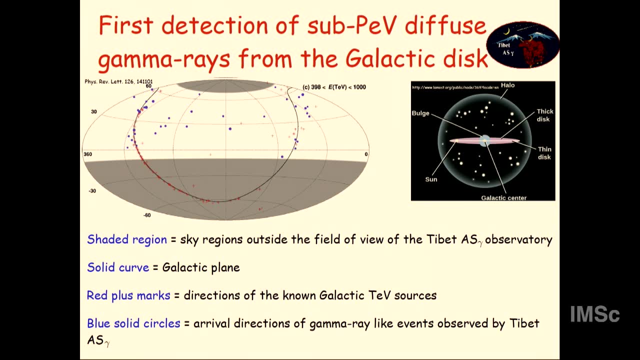 When mod V includes zero, That means you're in the galactic disk, all right. So let me tell you one thing. So in this thing, this is 0, 0,, all right, And this is sort of latitude 0.. 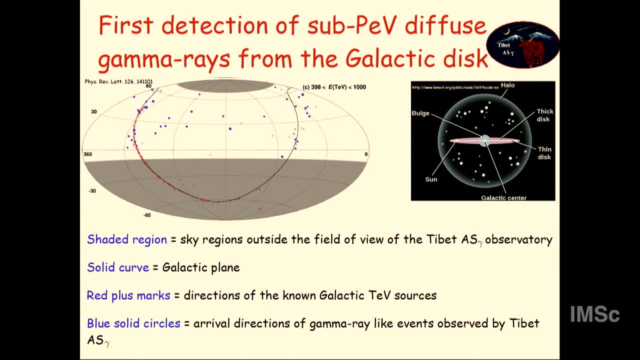 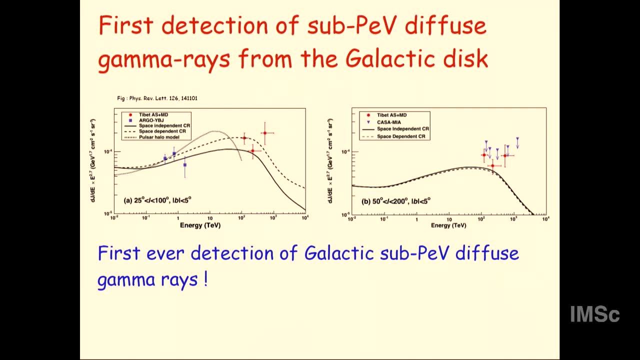 The galactic disk is latitude 0, exactly right, But the galactic disk has some thickness, so that's why they take plus minus 5 degrees. all right, You see there are very few data points here. More precisely, in this region there are three data points from TeV AES gamma. 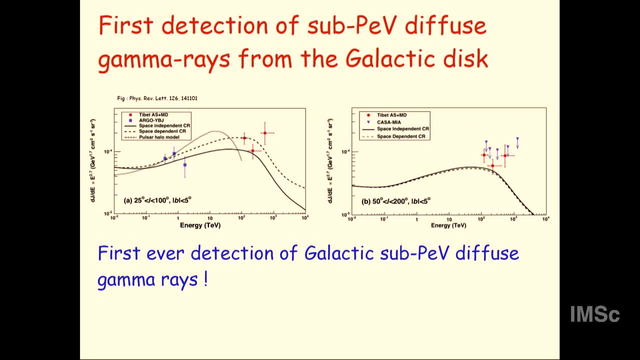 There's nothing else there. This is the first time we are seeing the Milky Way at in these energies, from approximately 100 TeV to 1000 TeV, 100 TeV to 1 TeV- the first time we were discovering it. 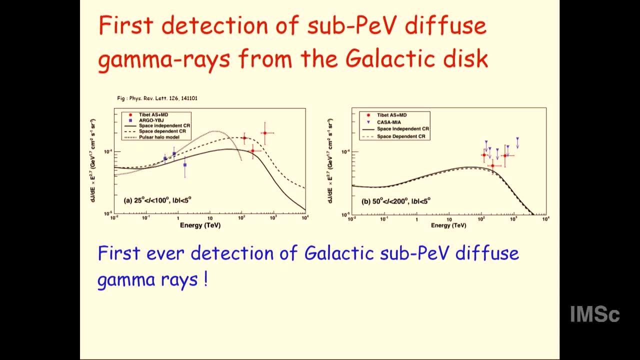 these are some old data points from the same part of the sky by Argo YBJ. they are at 1 TeV. remember I was telling you about TeV sources? this is actually not a source. this is actually a diffuse thing. I will tell you. 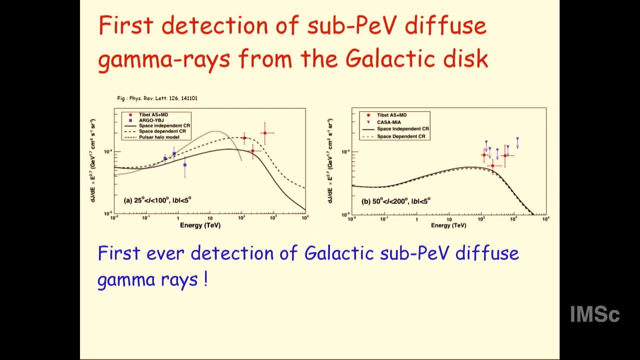 what diffuse is in the next slide, and these three lines that you see are various different model calculations of how the diffuse gamma ray will look like. look in the Milky Way, and there is something funny here. as you see, this is the first observation and this already rules out this model. 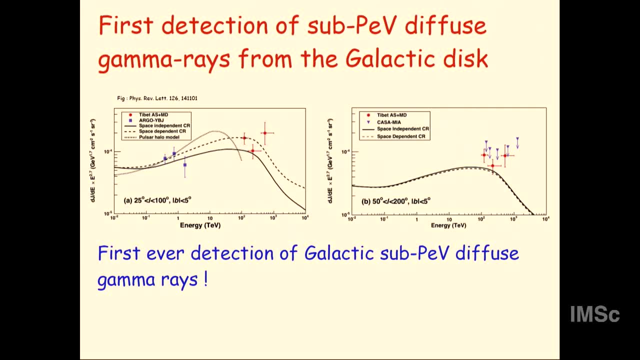 this pulsar halo model. you see this doesn't match the data set. this immediately rules out the first observation that we do. it rules out something that was viable before that observation. but there are other models which are viable. Tibet A is now also looked at- other part of the sky. 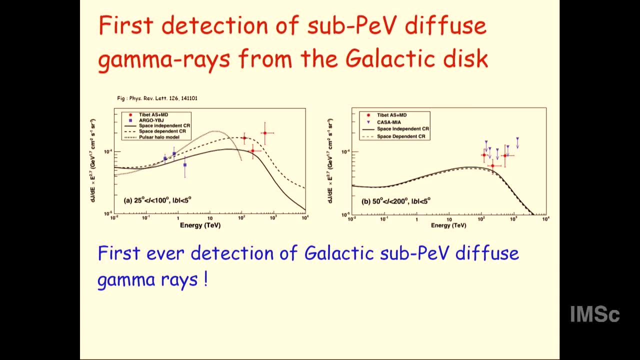 longitude 50 to 200 and mod B between 5 degrees. they found these data points again and in this part of the sky there was an old experiment called Casamia, where there are some upper limits. they did not find photons and they exactly found it. 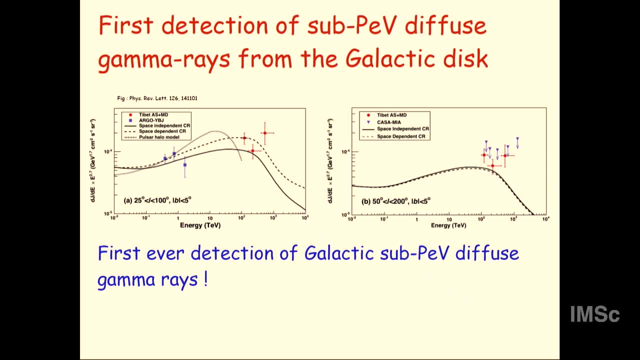 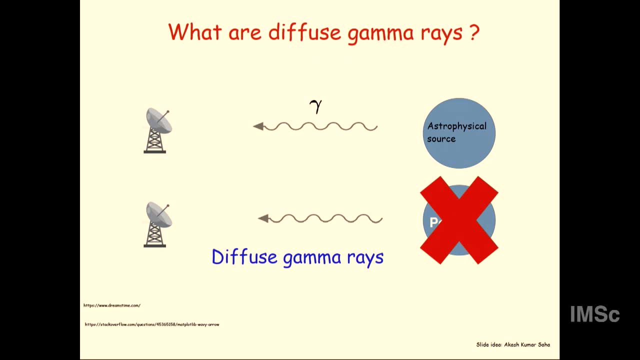 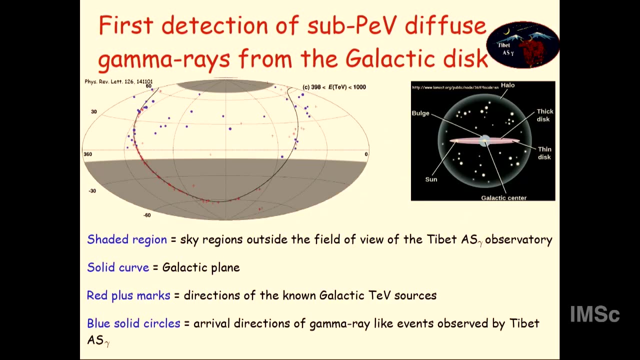 again, this is some prediction. this is the first ever detection of galactic sub-PEV diffuse gamma rays. what does diffuse gamma ray mean? in short? so diffuse gamma ray simply means that gamma rays do not come from an astrophysical source. remember, I showed you that plot. 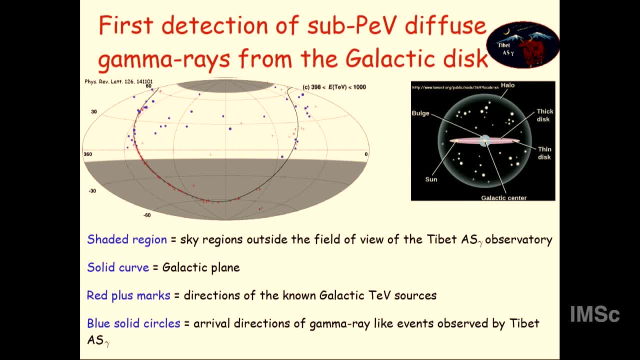 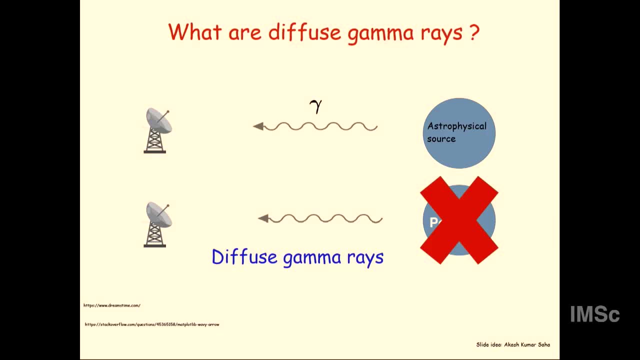 none of these blue circles here correspond to any other source. any source you can do, you can look at various catalogues. none of them correspond to it. so that tells you that this is a diffuse gamma ray. that means photons do not come from a source. if photons come from a source, we call it a point source. 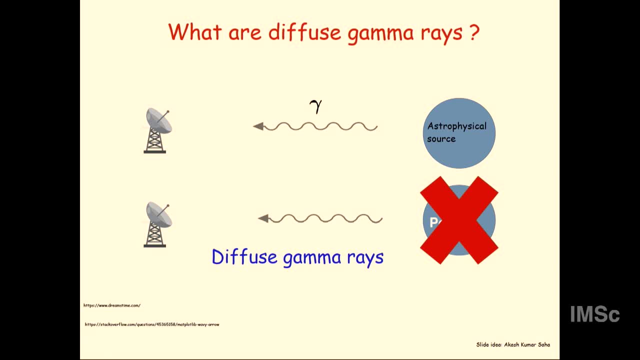 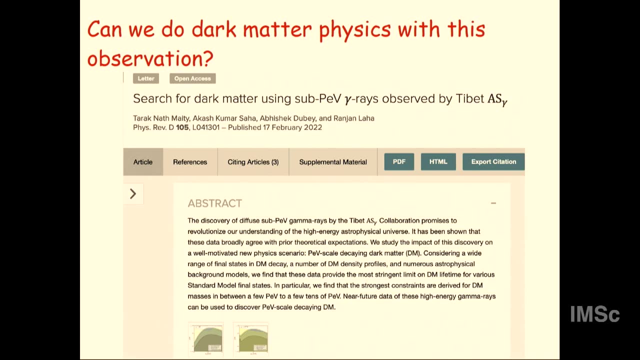 if photons do not come from a source, we call it diffuse gamma rays. alright, so last few things. so can we do dark matter with it? I've been telling you about dark matter, sorry, I've been telling you about dark matter. I've been telling you about cosmic gamma rays. 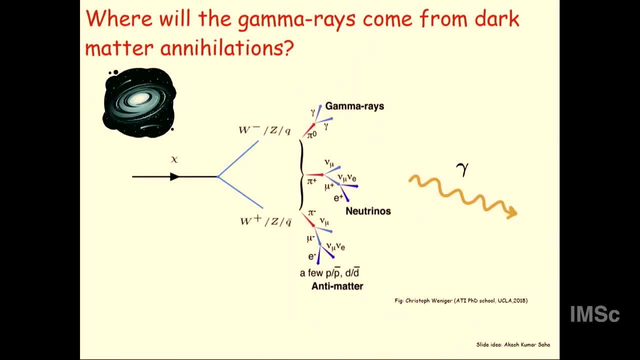 can we do dark matter? and this is what we had done. this was published this year so, as I said, dark matter can actually produce gamma rays. basically, dark matter can decay. I talked about annihilation and decay. let me talk about decay. dark matter can decay to produce various standard model particles. 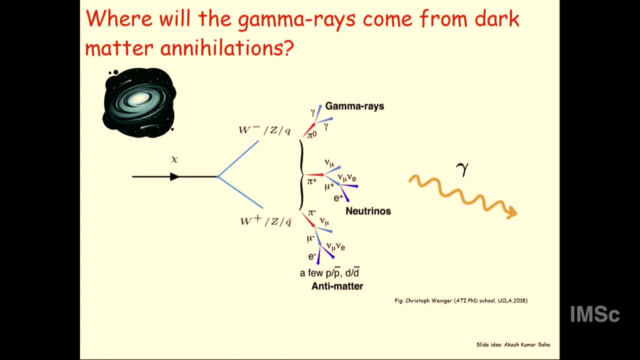 whatever the standard model particles do in them, you can get lots of photons. this is a very standard thing. this is the part that is unknown. can dark matter decay? we do not know. here I'm assuming that dark matter can decay. but once you produce these standard model particles, 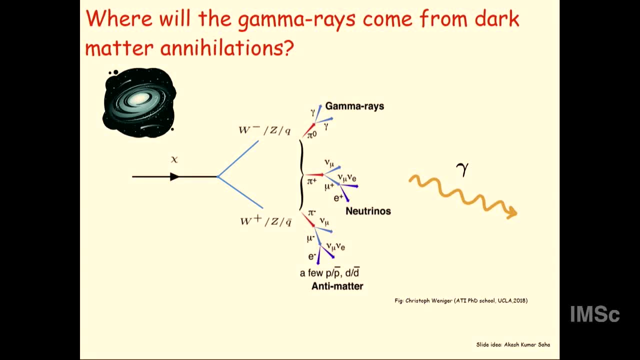 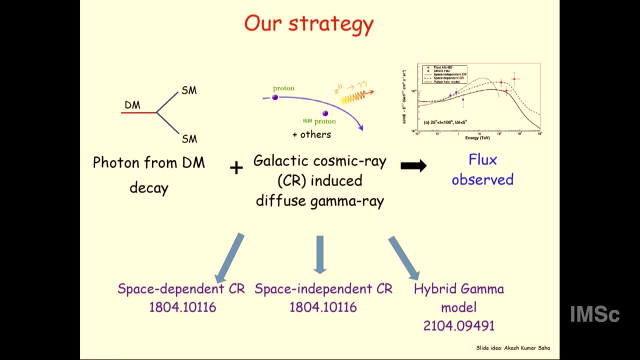 these W Z quarks, all of these things. they'll produce lots of photons. alright, now, given this new observation of Tibet Ace Gamma, we can immediately do this. we can say wait a minute, I have this plot right. this is what Tibet Ace Gamma has produced. 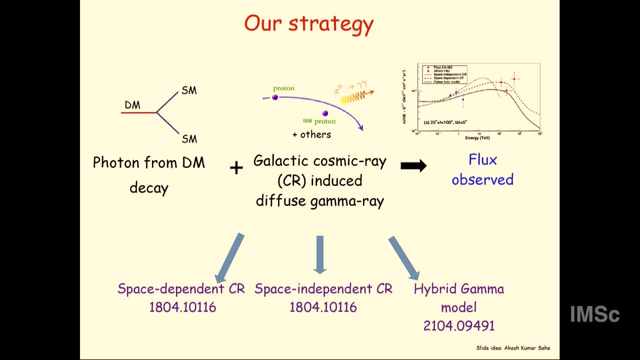 alright, let me assume that there are photons coming from dark matter decay. alright, we know these models existed, right. these two models remember this: space independent cosmically and space dependent cosmically. these models existed right. in other words, we know how to produce diffused gamma rays. 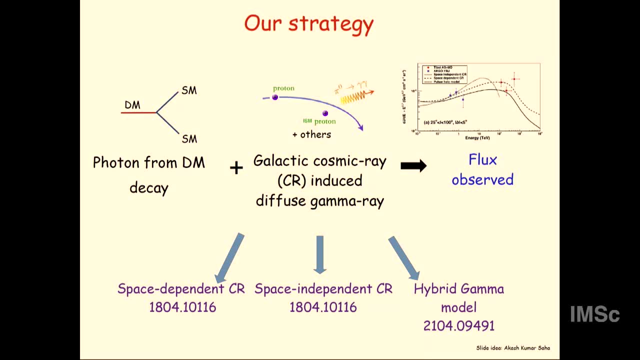 in the galaxy. we can add that, and then it should match this flux. alright, a simple addition, right? photons from dark matter, decay, plus photons from standard astrophysics should match this flux. in standard astrophysics there are various models, right, these are some fancy names. 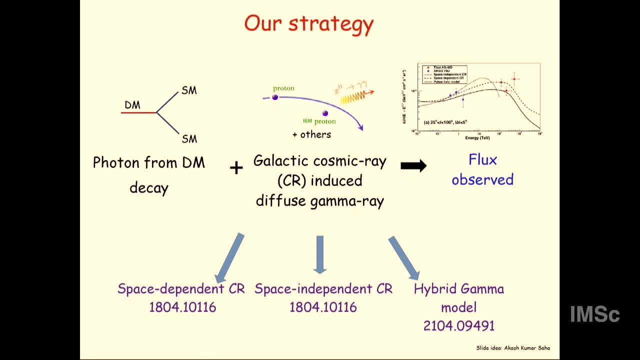 you don't have to worry about that. if you're interested, please ask me. I'll be happy to answer, but there are various models in order to reproduce this, this data set. our question is: can I, is there some signal of dark matter inside this data set? 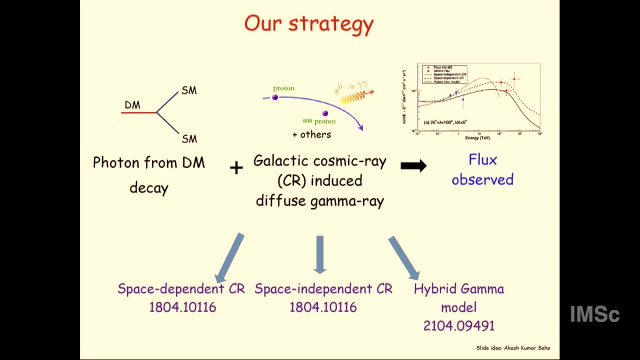 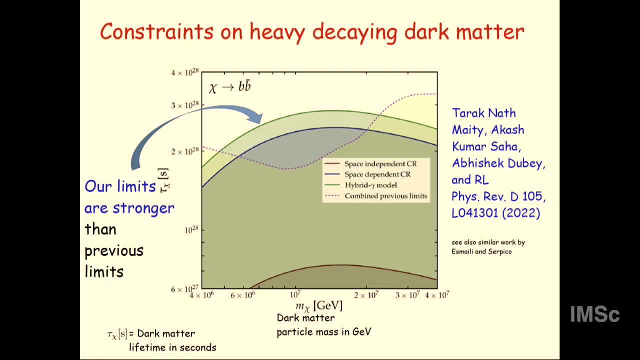 alright, we do some fancy chi-square to do these things, but the bottom line is we do not find any dark matter signal, unfortunately, right, unfortunately. so what we do is we limit the lifetime of dark matter that. how long can a dark matter particle live? what is spotted on the x-axis? 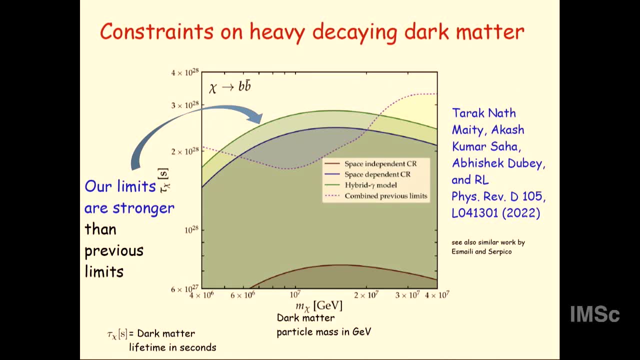 is the dark matter particle mass in GeV. alright, now this is 4 times 10 power 6 to 4 times 10 power 7, an order of magnitude and the lifetime of the dark matter particle. alright, and these are huge numbers. these are numbers, orders of magnitude larger than the age of the universe. 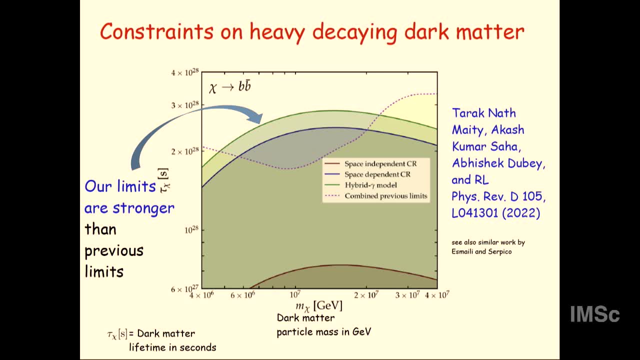 the age of the universe is roughly 10 power, 17 seconds. alright, this is 10 orders of magnitude, 11 orders of magnitude more than the age of the universe, and what we want is to. we want to find larger and larger lifetimes. this plot is assuming. dark matter, particles, decays to bb bar. 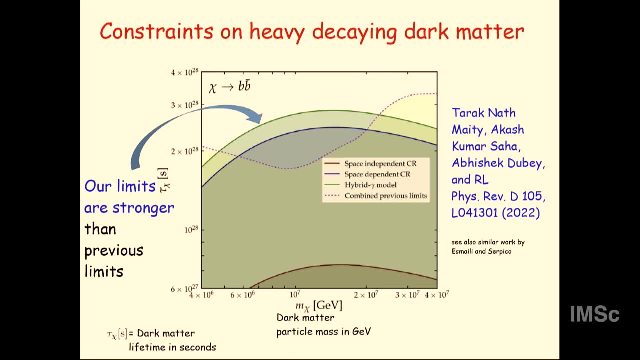 to bottom quarks, alright, anything that is shaded is ruled out. so this is the previous constraint that we had from other observations. right and now, what we did is we used this Tibet AS Gamma constraint to find this constraint: anything that was shaded is ruled out. 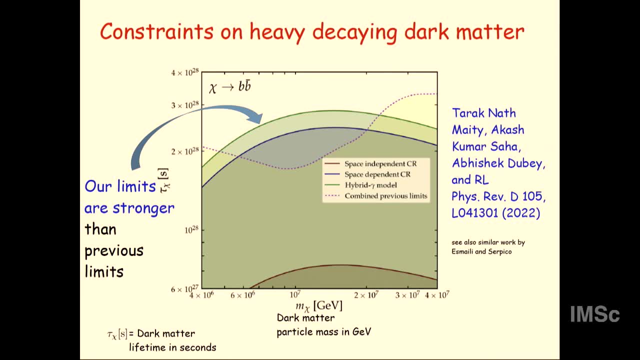 right. what we said is that between this range, which is roughly a factor of 3 or 4, dark matter cannot live. if it is, if it has this lifetime, lifetime in this range and decays to this bottom quarks, dark matter particles cannot be there. 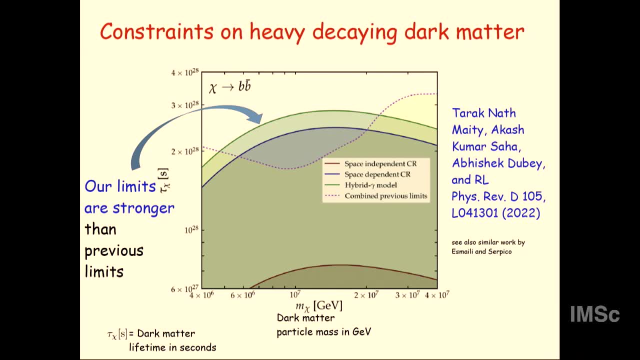 just by using this Tibet AS Gamma, the first measurements, we found this alright, and this at that, at the point of our publication, this was the strongest limit in the world, alright now, this is almost my last slide now, just to tell you the dark matter. physics is very interesting. 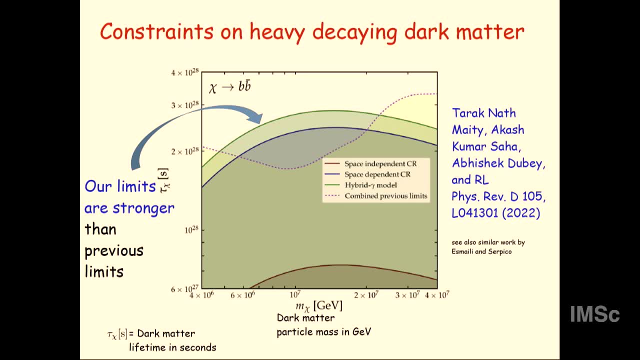 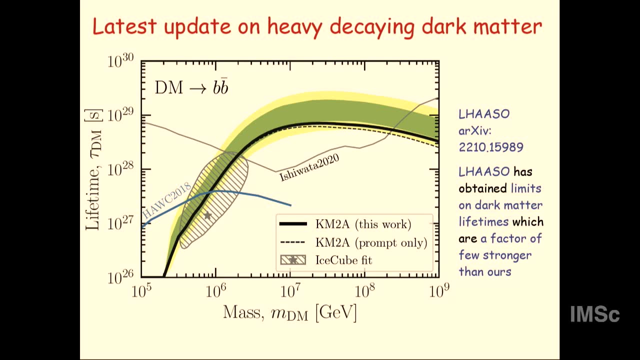 our, our limit was strong. strongest in the world for all of us. right, this was the strongest limit in the world. alright, now, this is almost my last slide. now, just to tell you the dark matter. physics is very interesting. our strongest in the world for one and half years. 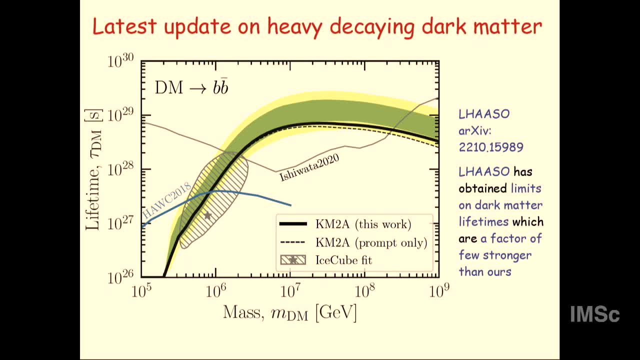 very recently, about a month ago, slightly more than a month ago- LASSO, which is large. this is a gamma ray telescope in again in China, which actually did the very same thing what we did with Tibet AS Gamma. they also looked at their data set and they have a limit. 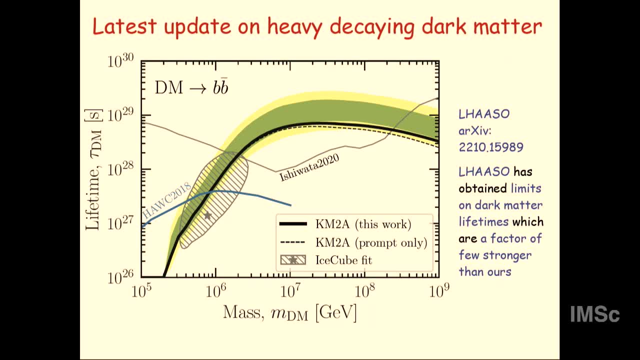 again, what is plotted on the x axis is the dark matter particle mass lifetime in seconds, and this is their limit, and this is their limit is a factor of few stronger than our limit, right? and, as I said, this is basically last month, right? so I started from dark matter. 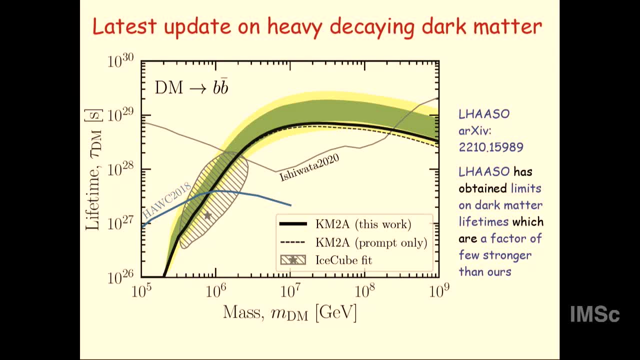 how dark matter was produced and I have brought you to what is happening last month in dark matter. in this mass range, I mean 10 power 29. now it is almost 10 power 29, assuming this bb bar. this is 10 power 6 to 10 power 8. 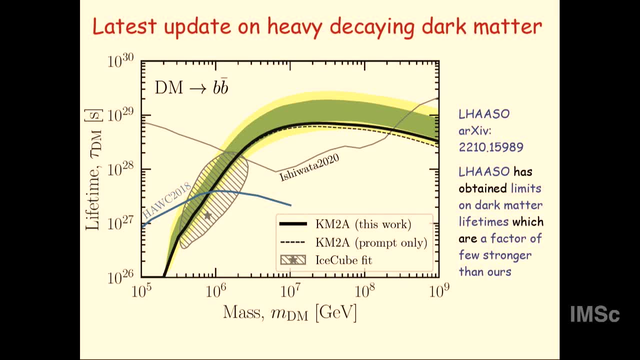 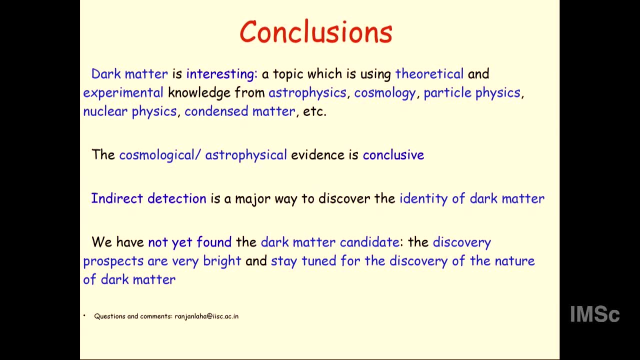 9, some this mass range. good, ok, so this is how I conclude. I hope I have been able to convince you. the dark matter physics is a very interesting topic of research. this uses both theoretical and experimental knowledge from astrophysics, cosmology, particle physics, nuclear physics. 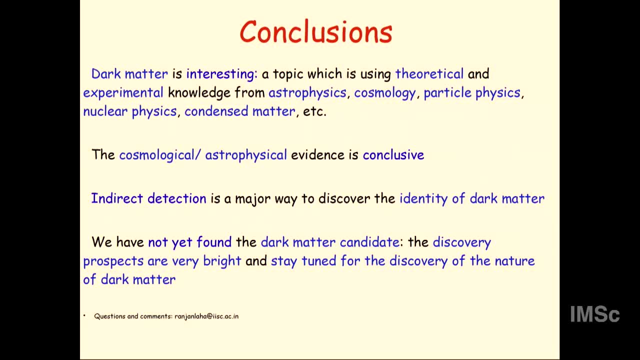 condensed matter, etc. the cosmological and astrophysical evidence of dark matter is conclusive, then we need dark matter, otherwise things break down. that's it, there is no question about it. however, what is dark matter? we do not know. I have already discussed indirect direction. I mean, there are various ways. 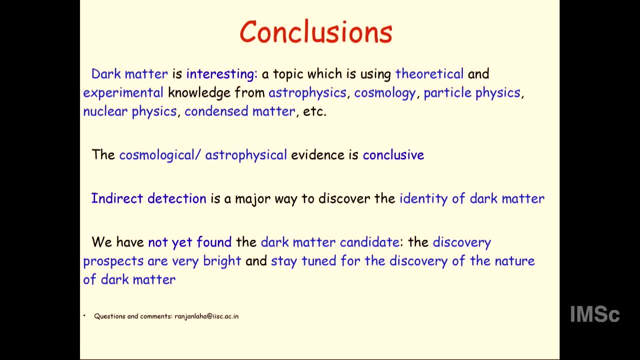 to detect dark matter. alright, there is not enough time. indirect direction is a major way to discover the identity of dark matter. although we have not yet found dark matter yet, the prospects are very bright. you saw, I mean last year, middle of last year, we got the best limit. 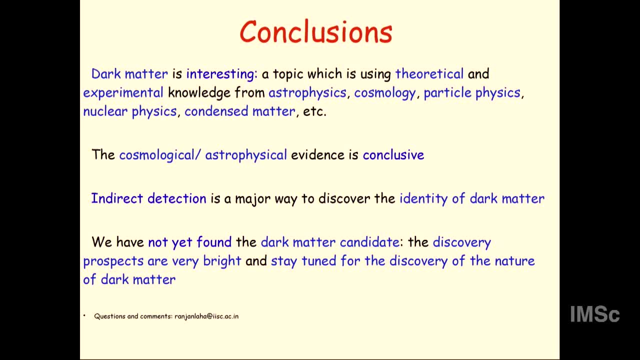 in the world. within one and half years, somebody became better than got a limit, stronger than us, right? so that tells you that things are changing very fast and we are actually having observations which can actually may be discovered. dark matter at some point, right? so stay tuned for discovery. 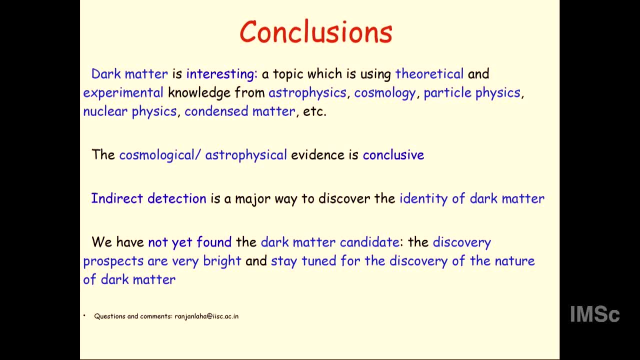 of the nature of dark matter. alright, sorry, over time, just saying thanks, Ranjan, for this fascinating talk and we are now open for questions. yes, hi, so you looked at the decay channel going to BB bar, correct? some other channel may give some other kind of cut offs as well. 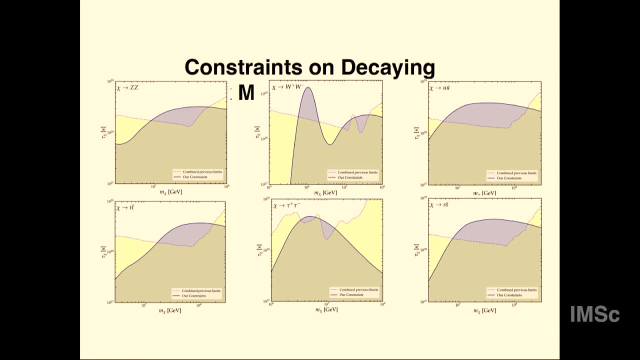 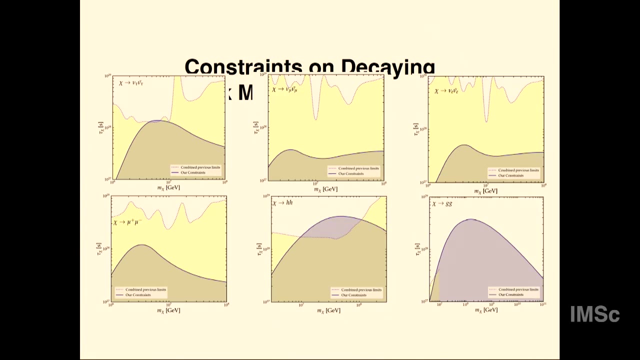 yes, good, good, how do we like this? is it ok? so sorry, so this is for various channels, ok, depending on ZZ, WW, UU bar, SS bar, tau plus tau minus tt bar. whatever you do, I mean, unless you are going for using the tibet as gamma observations. 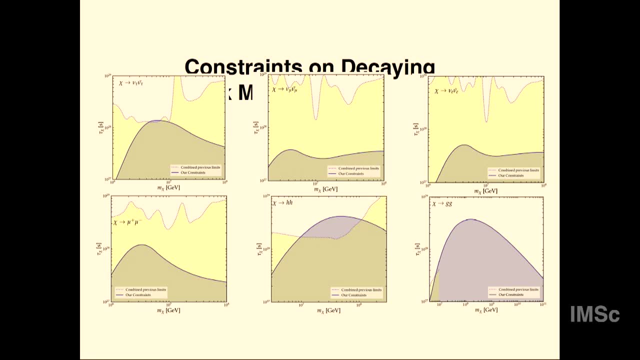 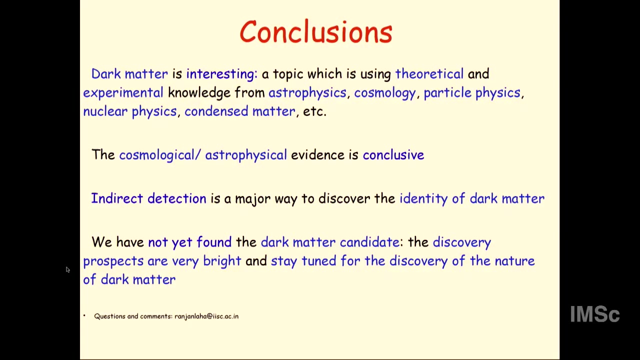 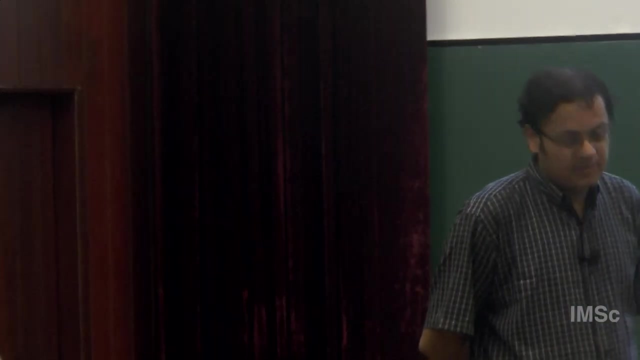 unless dark matter was going to first two generations. so either neutrinos or muons or electrons or nuvi bar, we always got the best limit. we got the best limits. now I think LASSO has sort of beaten us, but that was sort of obvious will beat us, That is all Correct. So that is why I started with the example of 21-22EV. 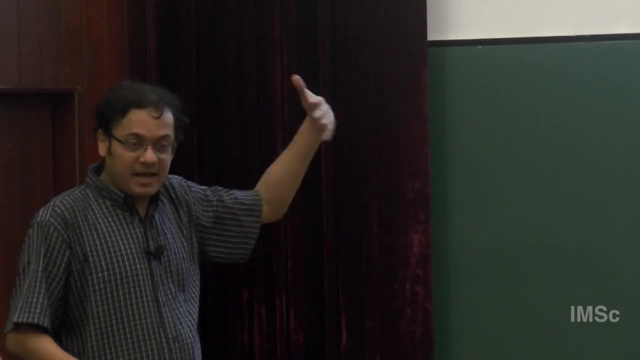 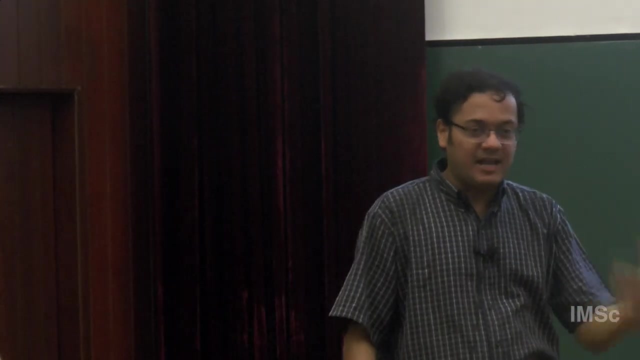 21-22EV there is. I mean we cannot whatever. as I said at the beginning of the, at one point of my talk, that there are techniques which will not be applicable to dark matter. Whatever I said is not applicable to find the lifetime of dark matter if it is mass. 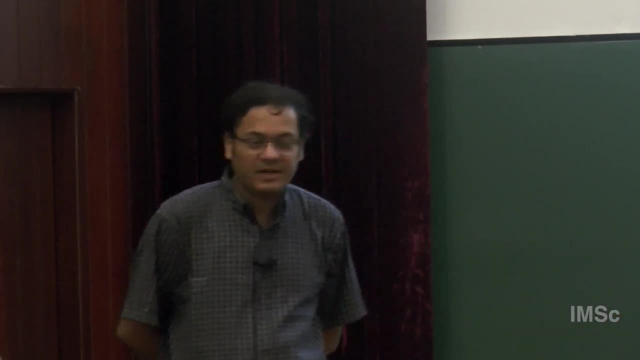 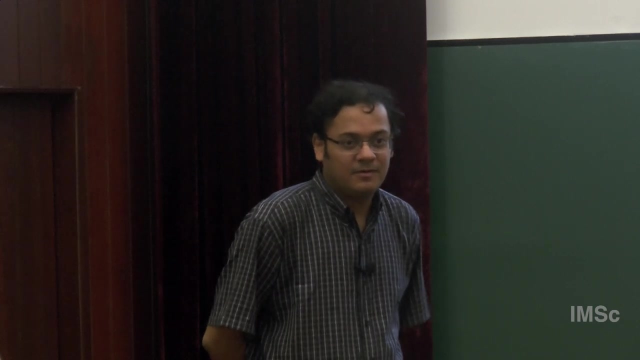 is 10 power minus 20EV. So if you want to find the lifetime of dark matter when the mass is 10 power minus 20EV, you have to do something else. I am happy to chat more. The profile which you get it has problems for all the. 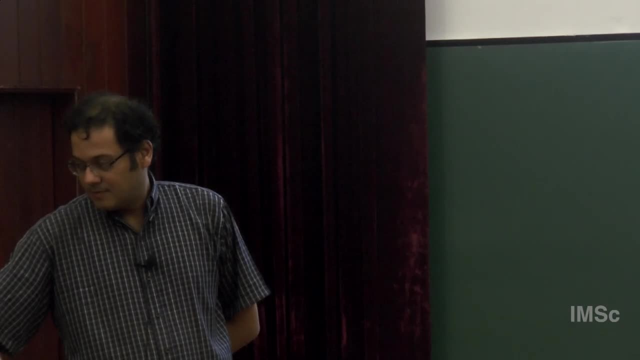 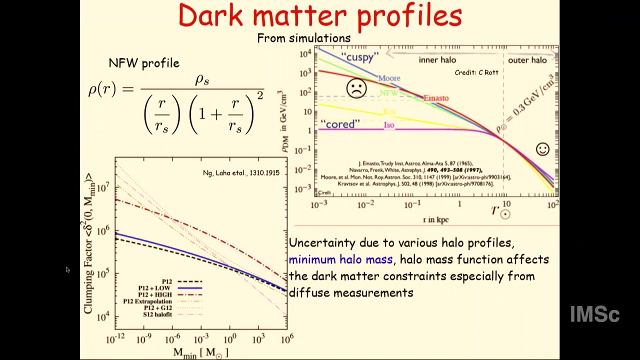 Correct, Yes, Which are not likely to be doing better? Yes, good. So let me answer the. let me rephrase the question for others. So remember I said that we have data from here, roughly from here, Where, where measurement, where simulations merge. Here we have no data right, So there, 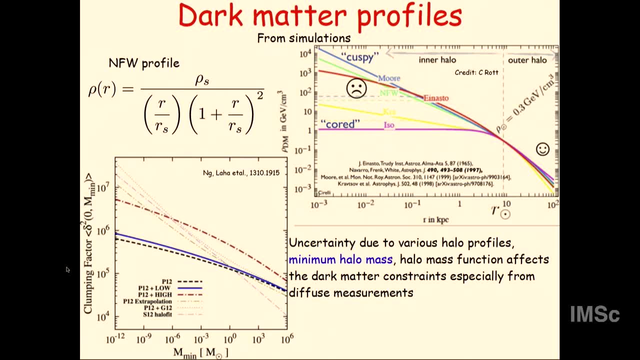 are something called Caspi profile. when the profile goes as r power minus 1 or even steeper, the core is r power 0. So there is something called a core and a core versus Caspi problem. The problem is basically when you do observations near the center of the galaxies, various galaxies. 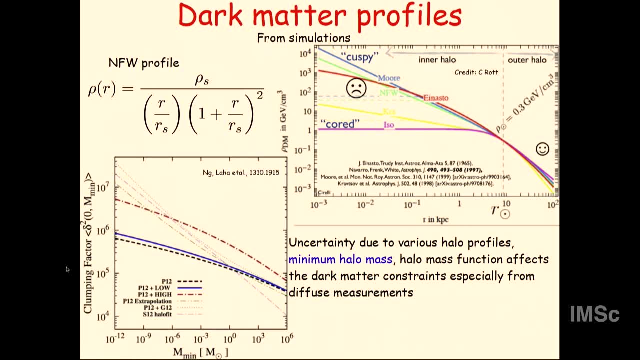 we do not know whether we get this or this, simply because the error bars are too large. There are astrophysical ways to solve it, And there are also There are particle physics ways to solve it, And ultralight dark matter is one particle. 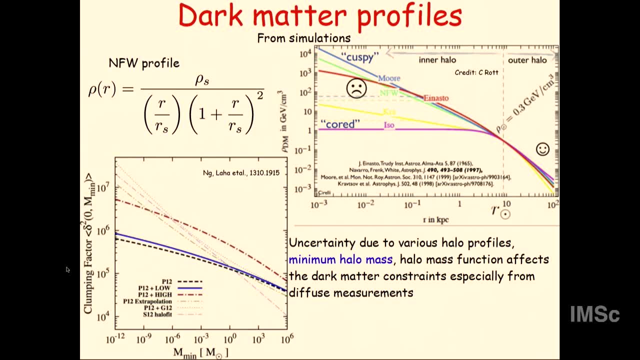 physics way to solve it, But there are also astrophysical ways to solve it. So I think that is the basic answer. So we do not know how it will get solved, But in principle, this ultralight dark matter is a candidate, is a particle physics way to solve this code. 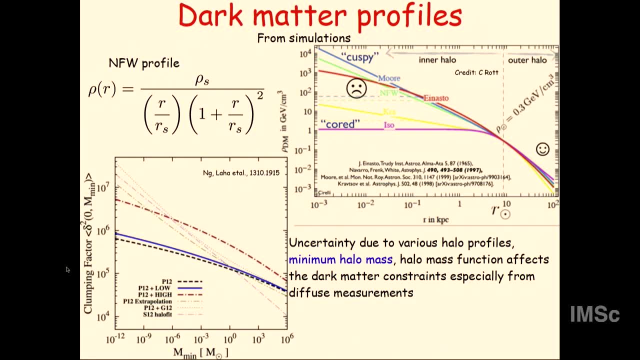 versus Caspi problem. I am happy to chat more. So initially you said that as the universe is expanding, these dark matter dark matter interaction will stop at some point, Correct. But then you said that for this indirect observations, you have these residual interactions that happen. What are those residual interactions? 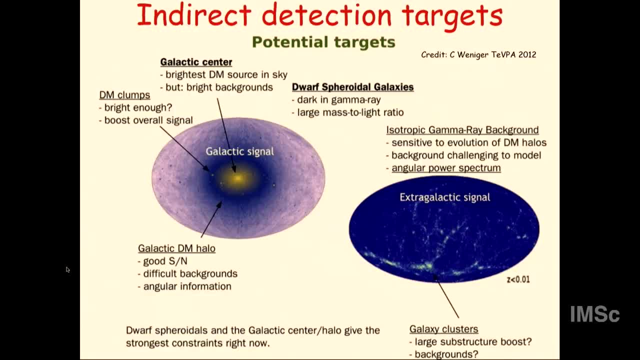 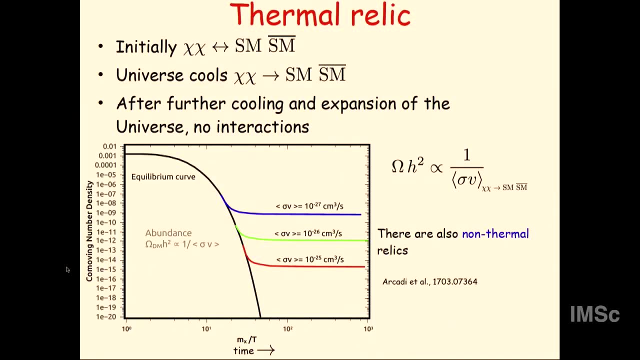 Actually, the residual interactions are still dark matter, dark matter interactions. Remember when I said this: this thing stops. I am saying it at the cosmological scale. The cosmological number density of dark matter is 4 or 5 watts of magnitude smaller than the number density. 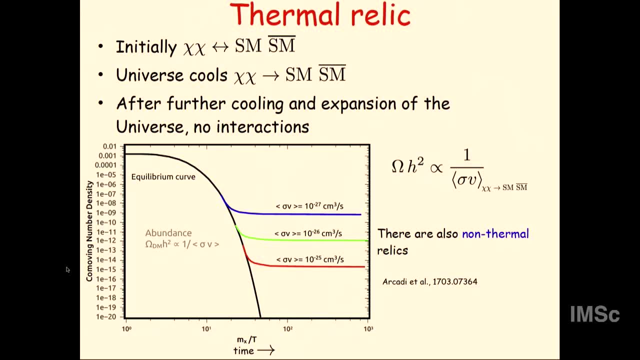 in the solar system. Since the number density in the solar system is 5 watts of magnitude higher, this you have to do a square right. Because of the higher number density, this analysis will happen, We will actually restart, But cosmologically dark matter will not happen. roughly I mean. 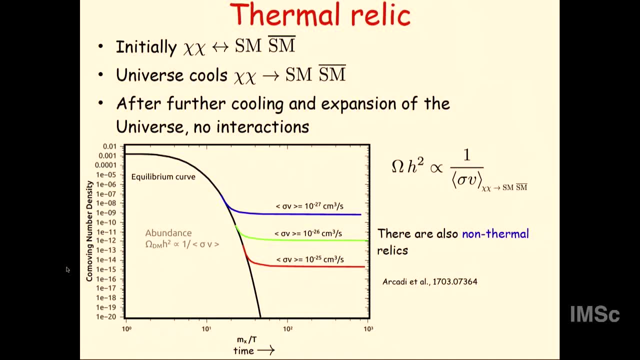 again, there are caveats. If you are interested, ask me I will. But that is the main point. Cosmologically this interaction stops. Cosmologically, that means if you look at the whole universe, this interaction is not happening. But if you look at certain regions of the sky where 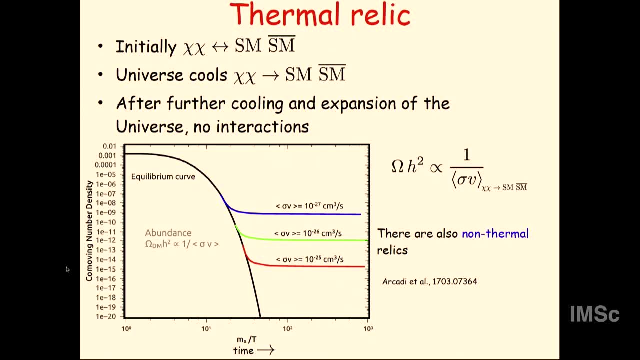 there is lots of dark matter density, then this interaction is happening Also. so This is one way to say, one way to explain this is basically: cosmologically, dark matter density is uniform, But there are pockets which are very high density. There are pockets of high density. 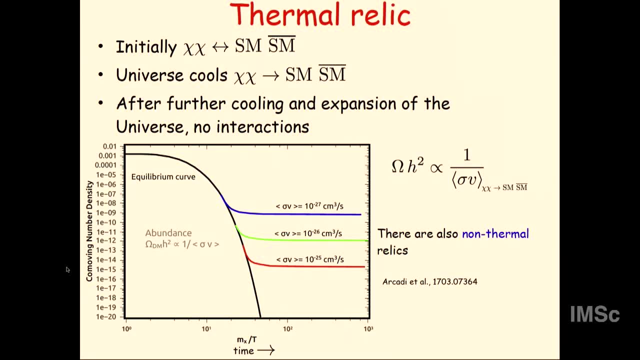 pockets of Low density, But overall it is uniform. Overall this interaction is not happening, But in high density regions this interaction is happening. That is the way to think about this. Also, these channels of decay, whether it goes to tau, to tau or bottom to quarks, they depend on the mass of the 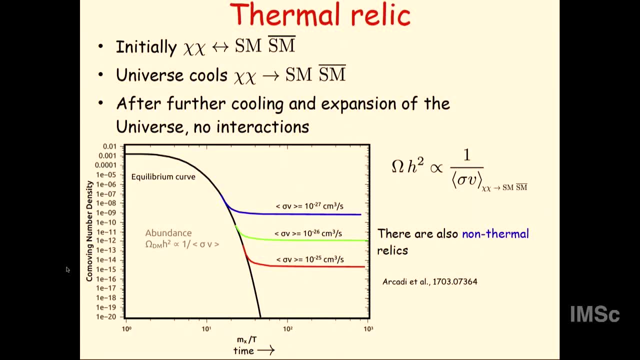 particle that are decaying, right, Yes, correct. So for massive particle you can have a lot of channels, Correct? What about the super light candidates of the particle? Good. Do they have same kind of modeling for this? Yes, good. So let us say I take a dark matter particle. 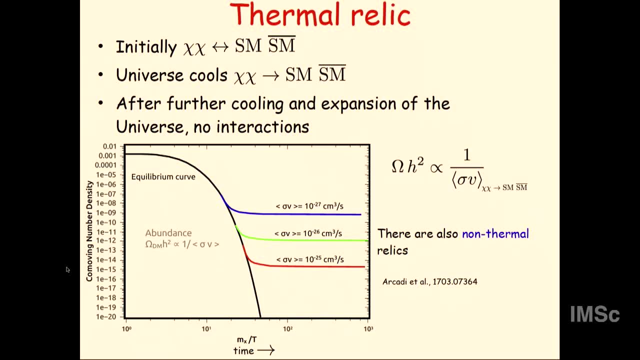 I take a dark matter particle with a mass of KeV right. Remember, dark matter is non-lativistic, so its energy is roughly KeV right. It cannot produce two electrons. That is it. So then, the only way to detect KeV dark matter in indirect direction is to look at gamma-gamma. 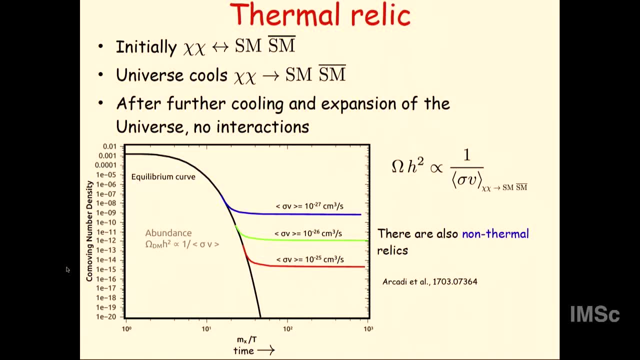 That is it, Nothing else. I mean in principle, neutrinogamma is also possible, Either gamma-gamma or neutrinogamma, So yeah, So what channels I am looking at? Remember there was this question: why am I only looking at Bb bar bottom-bottom, anti-bottom quark? 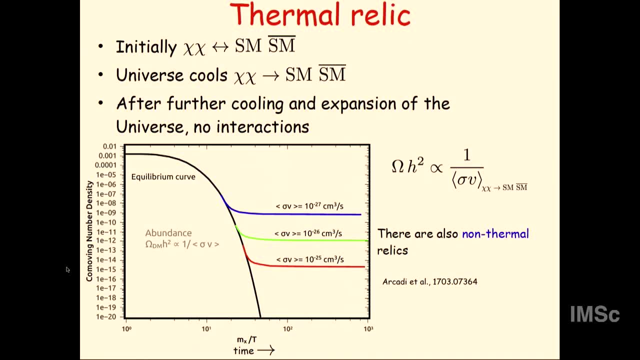 I can look at something else. That depends on what mass of dark matter particle I am looking at. Right, I mean light particles- can also look like this. Right, I mean light particles can also go to Nunu bar. The KeV dark matter particle can also go to Nunu bar. 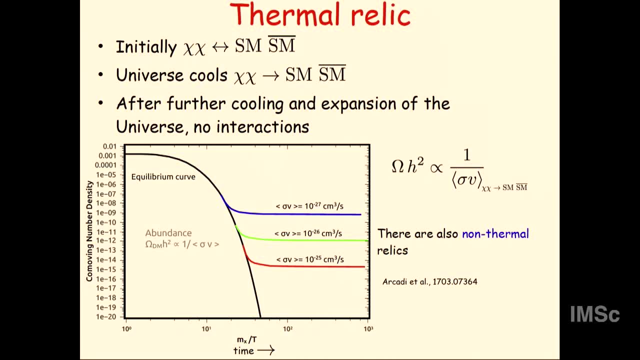 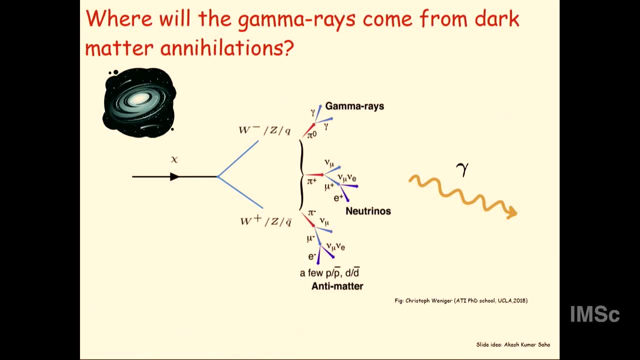 Right, So yeah, So that is a purely kinematic consideration. I mean, we were at masses of 10 power, 6 or 10 power, 7 Gb, Everything is allowed. That is why we, As an example I showed, 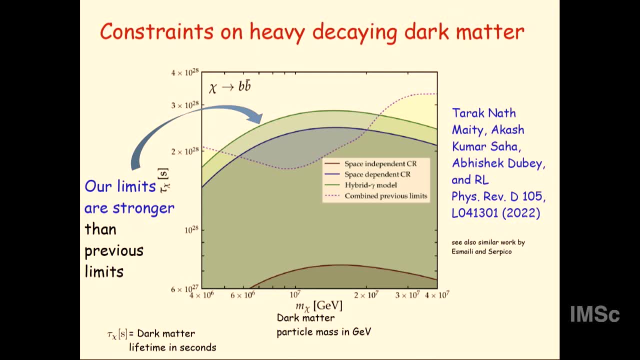 Yeah, For Bb bar, but I later showed like all kinds of particles are allowed, Right. Okay, Thank you. Yeah, You are welcome. It is not just the mass right, It is also the coupling Correct. 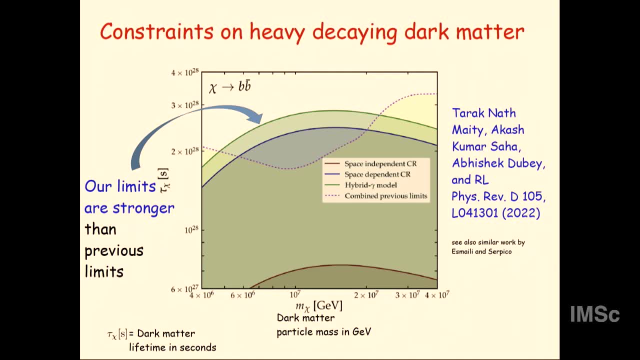 Maybe you have assumed that the coupling to all these particles is the same of the order of Yes, So that part I did not say, because that is a model-dependent statement, Right? So this is So given kinematically, this thing is always allowed. 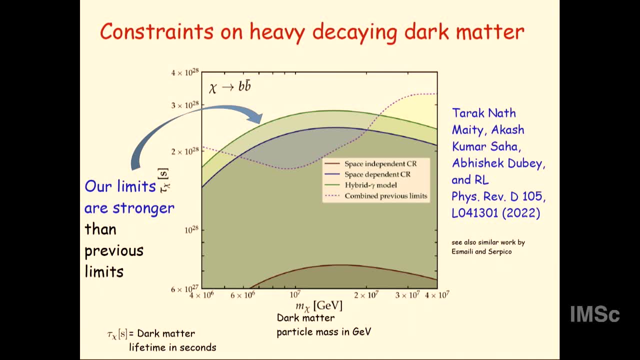 By using kinematics. But if you want to think of some model, this thing may not be allowed. All right, All that this masses. this thing will always be allowed by loop corrections. more precisely, Suppose dark matter goes to only neutrinos. 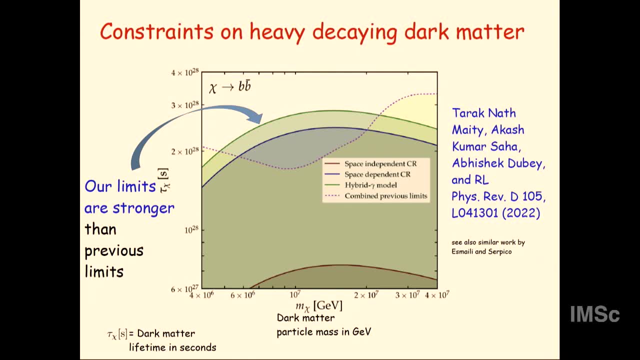 You can show by loop corrections. it will also talk to Bb bar Well W will come. No, no, Actually these people have done seriously, I agree, but it will be like No, no, no, No. 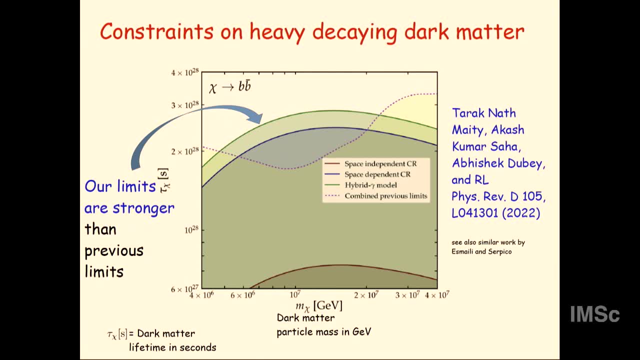 At this mass is actually super important. So this is technically what is called electroweak corrections. So that means, suppose dark matter goes to Nunu bar. Right, You can say Dm goes to Nunu bar and there is a W coming out. 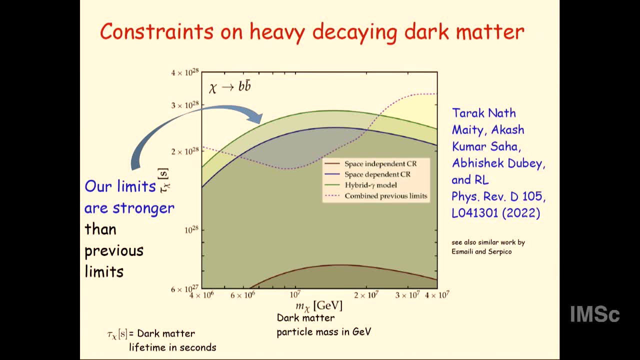 At what center of mass energy is this W coming out important? It becomes very important beyond 1 TeV. Actually, That is true, Yeah, So here we are at a mass where everything is allowed, Everything happens, because all No. 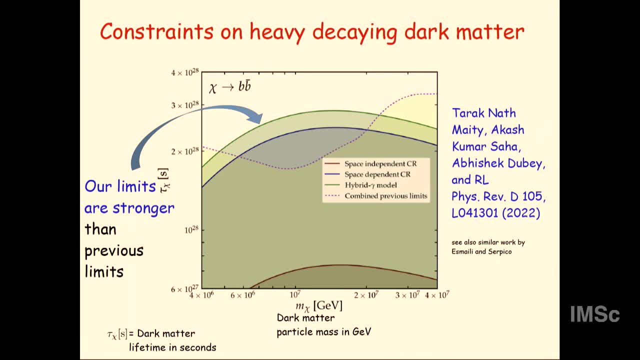 Lighter ones, Yes, Correct, Lighter ones. that will not happen. That is why I said kinematic. There is some particle phase thing, but I was trying to make it more simple In kinematic ways. that is allowed. 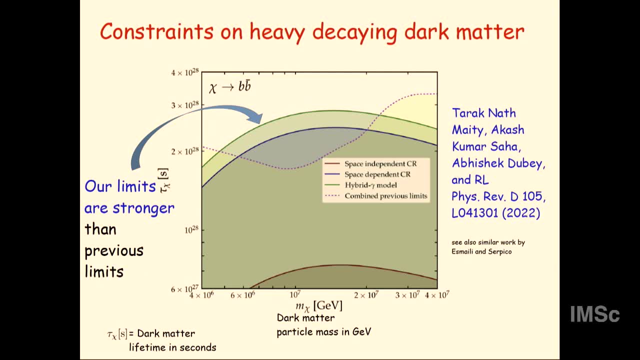 But yes, What Professor Indubhuti said is correct. There is also a particle physics argument, But if you are agnostic, So in this work we were sort of being model independent, In the sense that we do not care what model is giving it. 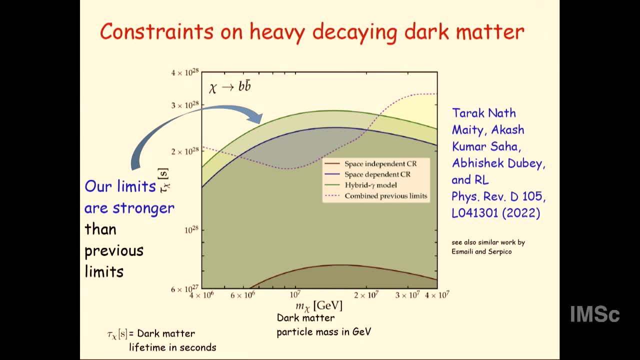 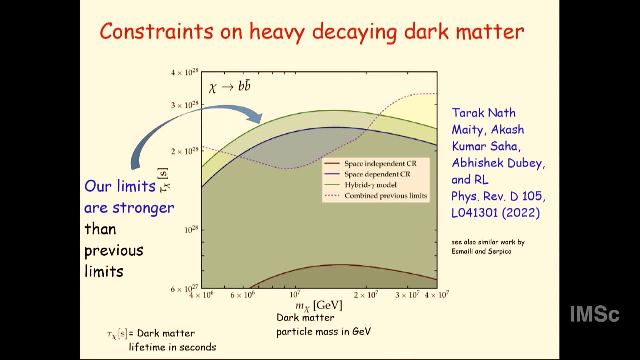 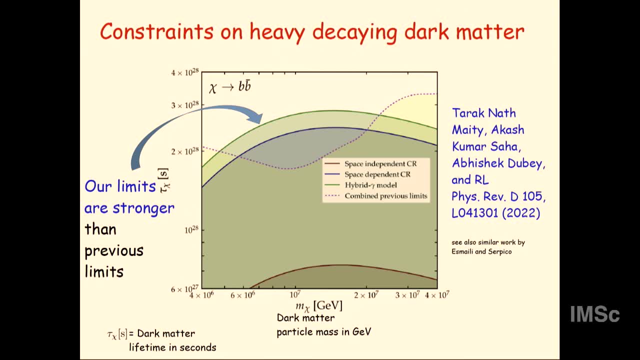 decay is happening in this mass range, then our limits will apply immediately if the lifetime is in this range. That is what I mean. So the interaction strength will determine the lifetime. I mean you can make the lifetime. You can make the lifetime much higher than that. 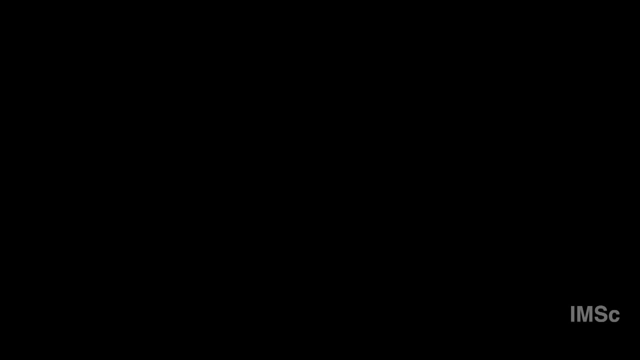 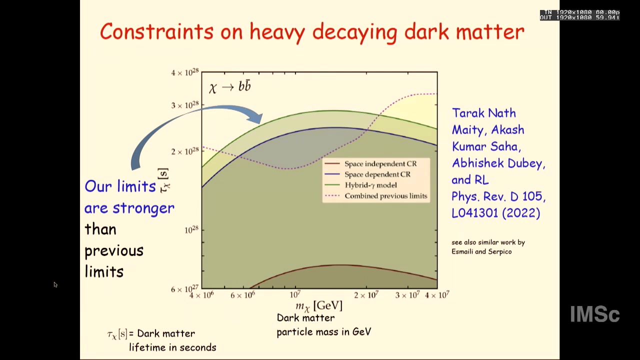 I cannot constrain it. I cannot constrain it. But if your lifetime is using your interaction strength, using your Lagrangian, if your lifetime is in this range, actually in this range, the whole thing, it will get ruled out immediately in this mass range. 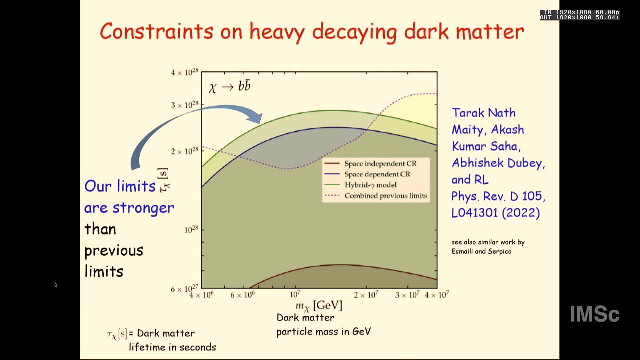 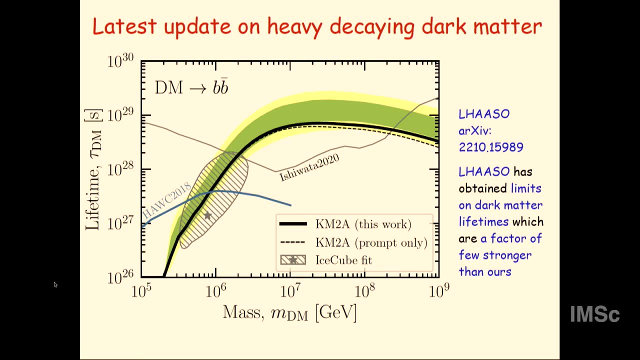 So that is what I mean by model independent. It is actually model independent, this Or even this result, this LASSO result. So if you make any dark matter candidate which decays to Bb bar in this mass range, 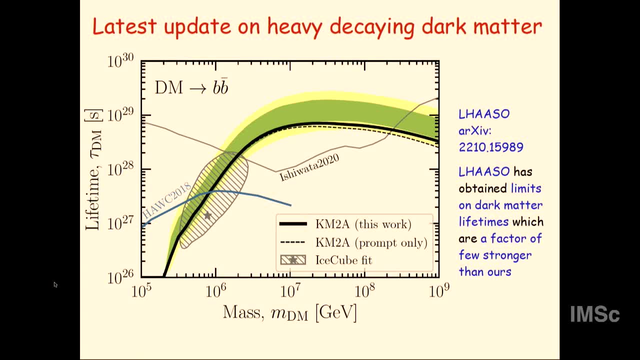 this whole region is ruled out. That means any lifetime smaller than this is ruled out. It cannot be there. 9 and 7,, 16,, 17.. So 10 power 17 is the age of the universe, Correct? 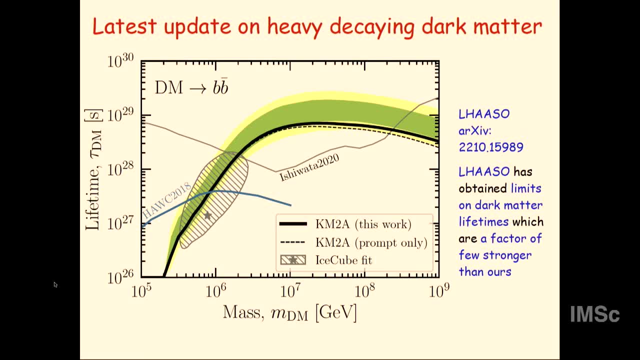 Correct. So this is 11 orders of magnitude. 11,, 12 orders of magnitude, Very huge. I mean, Okay, Yeah, Because dark matter is hardly decaying. This is actually one of the questions: Dark matter is hardly interacting. 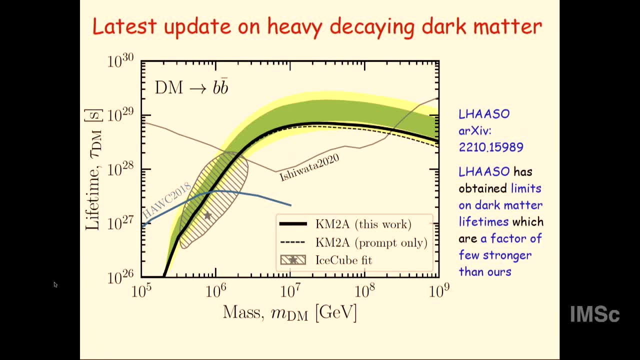 I mean this basically, is that dark matter is hardly decaying. But since, Why does this work? You can say, wait a minute. How come we know the life Something, lifetime of particle which is 11 orders of magnitude larger than the age of? 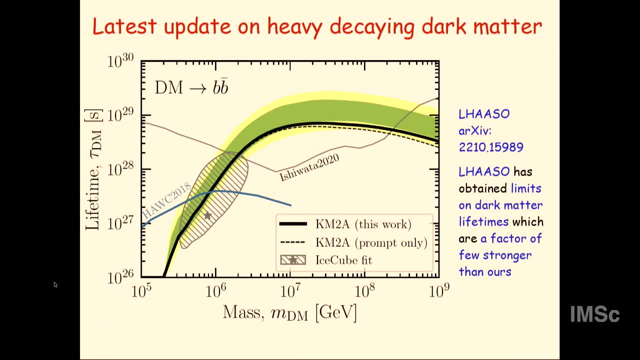 the universe. Well, this is just simple. radioactive decay right 1 over tau. If you look at large number of particles: 1 over tau. If you look at large number of particles 1 over tau. If you look at large number of particles, 1 of them can decay. 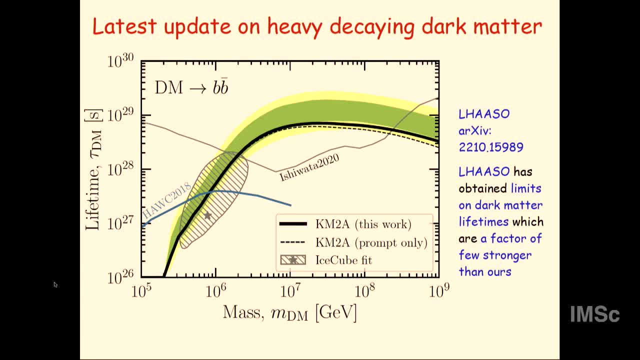 That is what actually is happening here. There was an online question. He asked: is it possible to understand the sluggishness of dark matter as due to its strong self-interaction rather than thinking in terms of its mass Good? So let me rephrase the question: 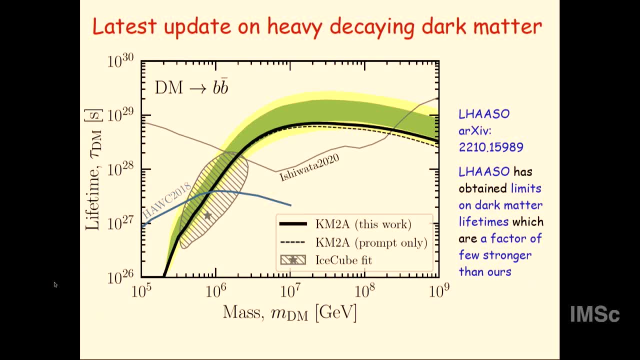 The question is: the dark matter is sluggish. that means dark matter is non relativistic, Can I understand? due to its strong self interaction, that means dark matter interacting with themselves. Actually, we do not have any conclusive proof that dark matter interacts with itself. We have some hints, but those are not conclusive proofs. 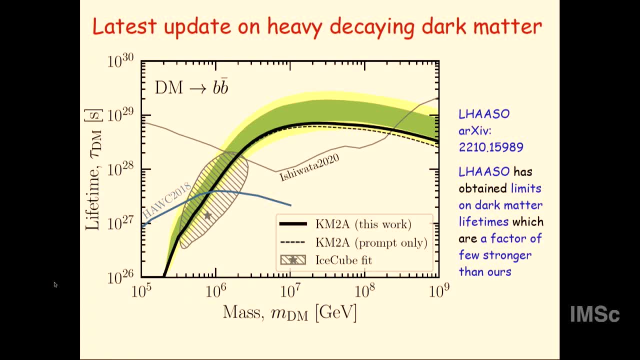 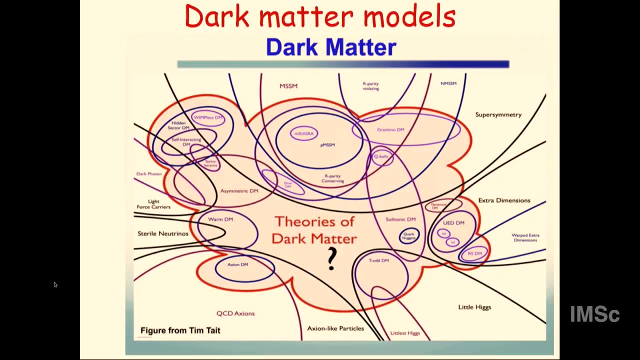 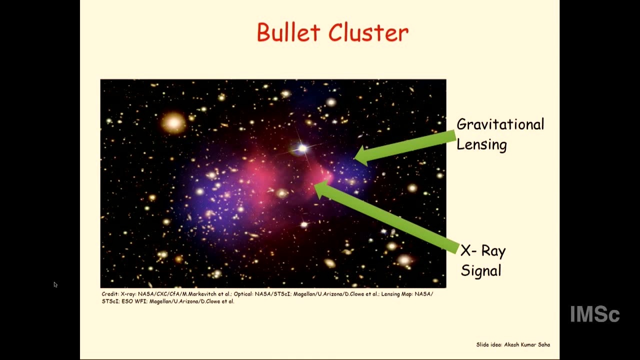 So dark matter is non relativistic simply because how it is produced. It is not due to its self interaction. In fact, I showed you a picture which I did not say because there is not enough time. I did not want to confuse you. This is a proof that dark matter does not self interact as much as baryons, as much as standard model particles. 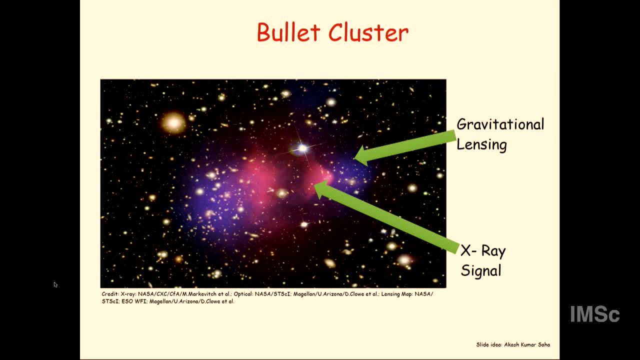 You see, standard model particles got clumped, got caught in the center. Dark matter particles have just zoomed past it. There are two blobs of dark matter and that blobs of dark matter have two smaller blobs of baryons inside them. This baryonic blobs got caught in between. 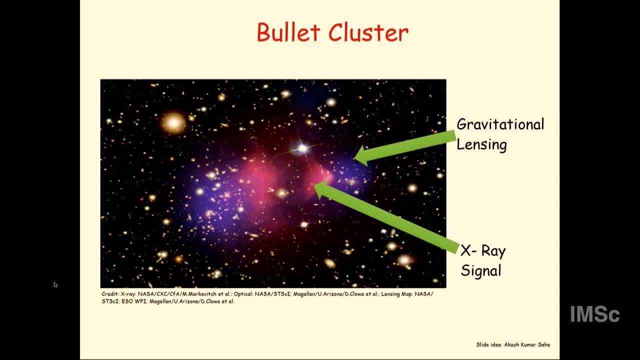 and that blobs of dark matter got clumped And they are stuck here. The dark matter blobs just went through. So this is a proof that the self interaction of dark matter is less than some number. I can give you the number in more detail, but let us 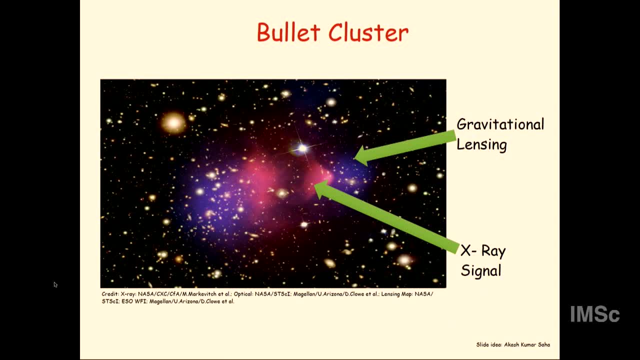 From this velocity can you say anything about mass of dark matter? No, So funnily, what happens is from this plot, what you get is the interaction cross section, self interaction, cross section by mass. You get that number, Sorry. mass of the dark matter candidate. 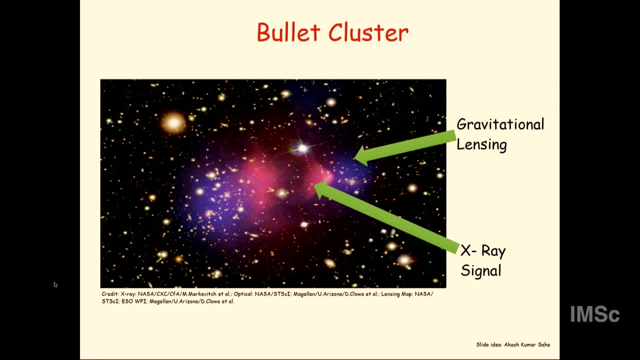 So you are saying that it is just another particle? Yes, Very like mass then for mass. Yes, So lambda by m is what you get. Yes, What you get is Yeah, Correct, I mean technically, Yeah, Correct, Yeah. 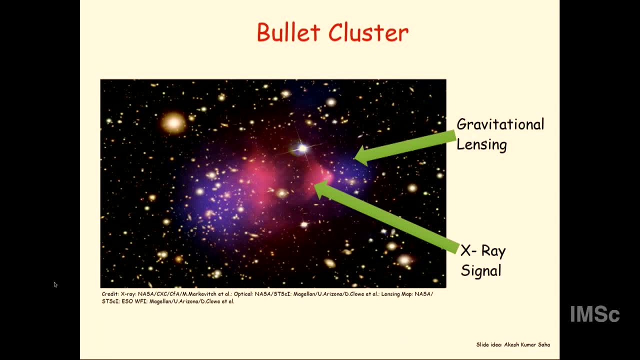 You get lambda by m, You will not get what is the mass. Yes, So no, Almost Almost no observations can tell you what is the dark matter particle mass. Almost no observation can tell you what is the dark matter mass. The statement is actually wrong. 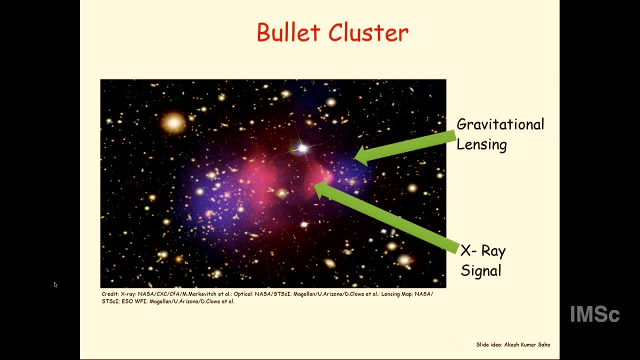 I am telling you: But how is it wrong? Yeah, There are ways to say it. I mean, actually, I can tell you in detail How Why this statement is wrong. Yeah, But mostly this statement is correct. Let me put it this way: 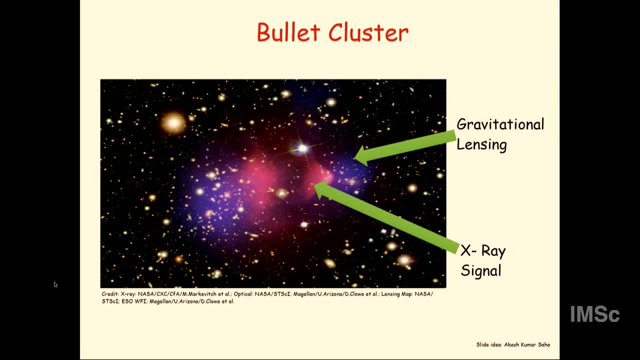 Yes, How do we know that? those blue circles dots in that Yes plot, Yes, are not due to any of the gamma, Not this: The Tibet, Oh As gamma Yes. Tibet As gamma Yes. 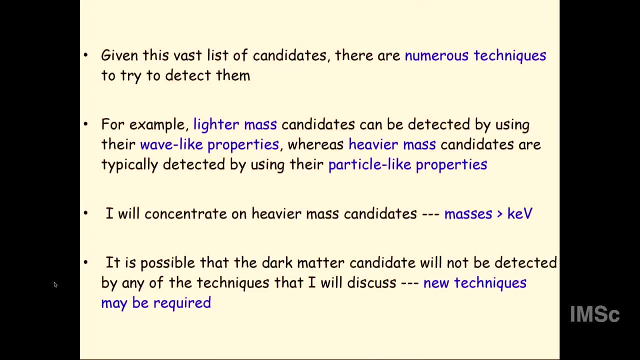 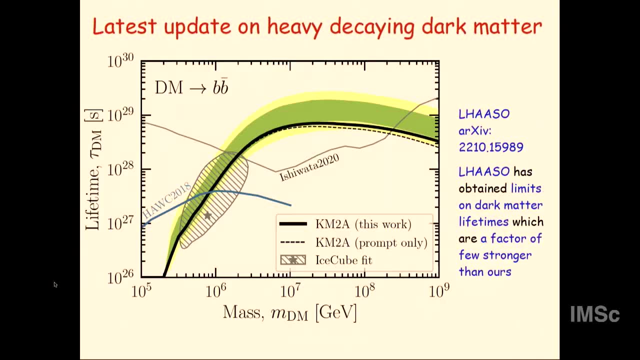 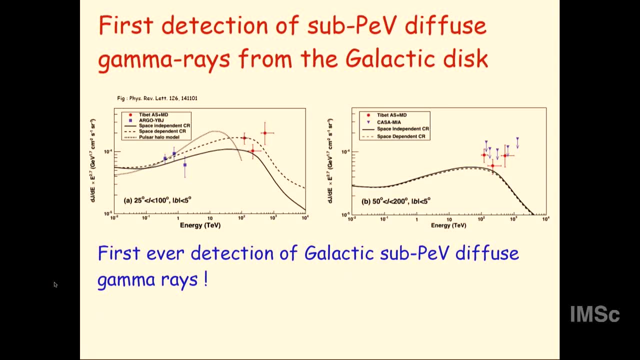 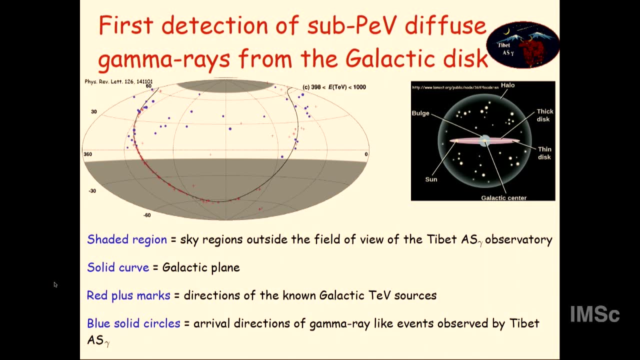 Yes, Yes, Yes, This one. Oh, Ah, Good, So you mean this, right? No, How do we know that the blue Okay is from Okay? Sorry, diffused gamma-ray flux, This one. 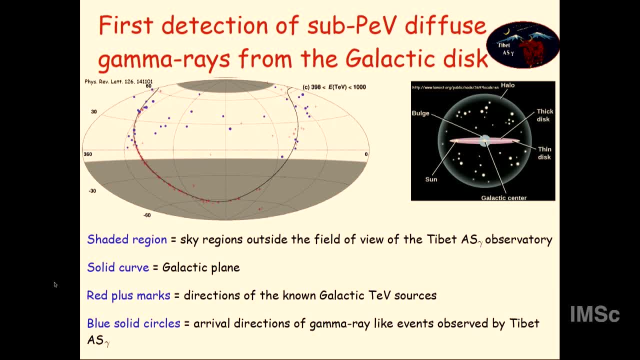 This one, right? Yeah, Yes, Good. So let me rephrase the question. Suppose you see gamma rays coming towards you, How do you know it is coming from a source or it is coming from a diffuse thing? that means not coming from a source. 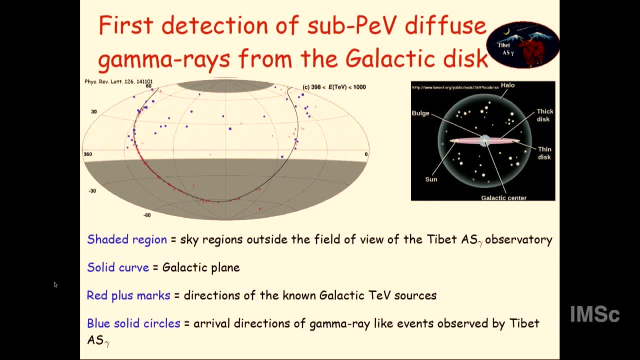 You would know it by doing further observations Right, Currently, since these data points are not coinciding with any known source, Okay, with any known source, we think it is diffused. In other words, it is very weird that a source 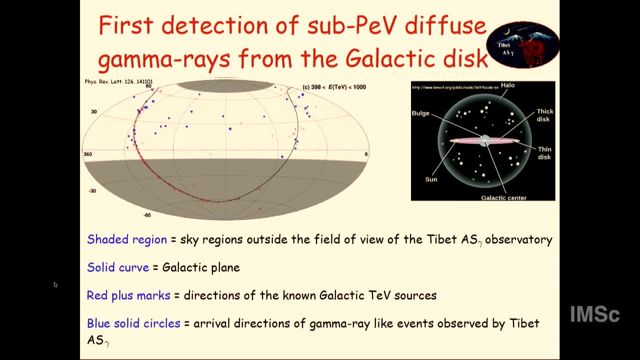 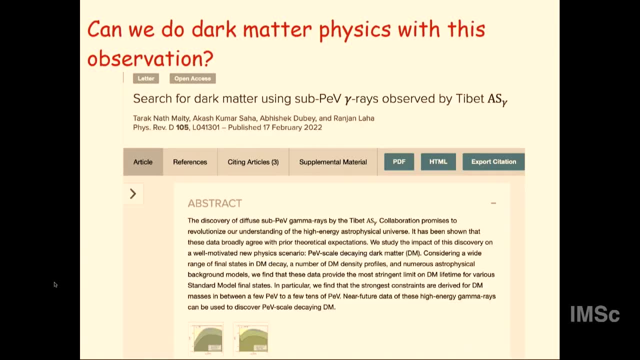 is emitting in this energy range and not emitting in anything else. That is extremely weird. Put it this way. Let me explain it this way. Okay, so no other frequency is observed. Yes, no other frequency is observed. Let me give it one line. So suppose this diffused? 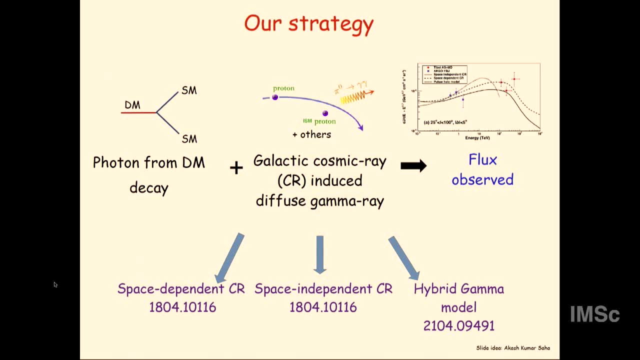 way to produce is this Cosmic ray protons interacting with interstellar protons and producing pi naught. So pi naught is giving gamma-gamma. The moment this happens, you will say: wait a minute, pi plus, pi minus will also get produced. They will produce. 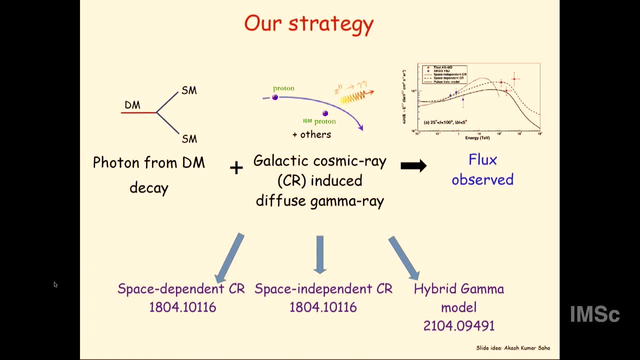 electrons. These electrons will produce, they will do synchrotron radiation. How come we do not observe that? We do not observe that? That is it. That means it is not coming from a source. Every source that you see produces all other frequencies. So these sources most. 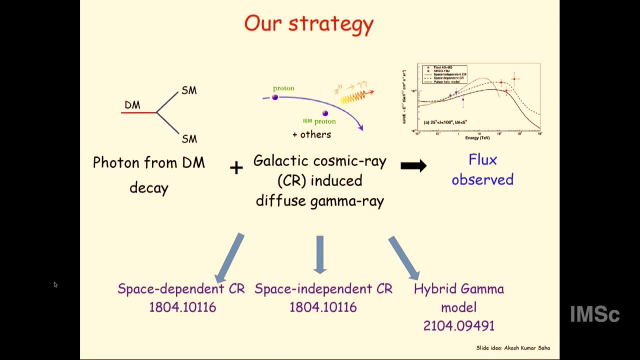 probably are not producing other frequencies, So this means this is diffused. See, what is diffused is actually diffused. It is actually a time-dependent statement in the sense that we do more observations, Sometimes we actually see a source like that. So currently we think these sources that 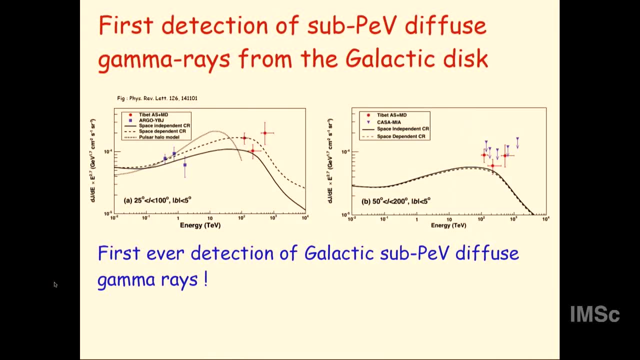 means this thing are diffused. So that is the current understanding. So the diffused People have actually tried to look for. actually, only recently, last week, Ice Cube tried to search for photons from sorry neutrinos from last, from last sources. They did not. 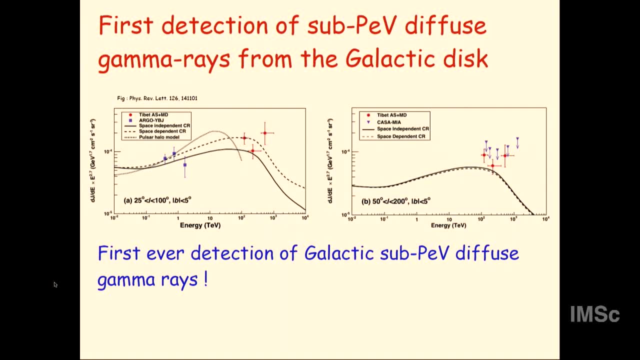 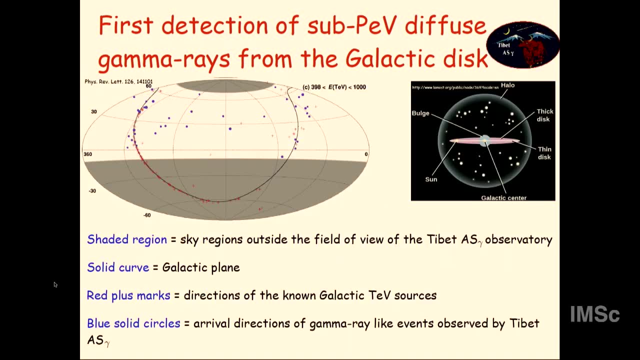 find anything That produces a constraint. but yes, that is how we found it. So, if I, if I followed correctly, these blue circles are observed only in the AS Gamma experiment. Correct? Like the other experiments, are insensitive to diffused gamma-ray flux or white like. 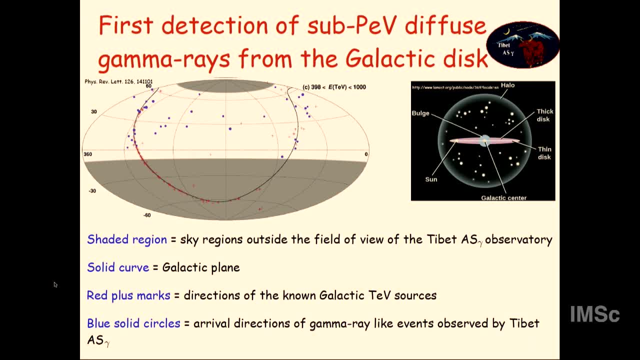 So the other experiments, first of all, at this energy range, only Tibet, AS Gamma and LASSO are working. Okay, All right, Yeah, And there is something else I did not say. I can say it now, since you asked: LASSO has. 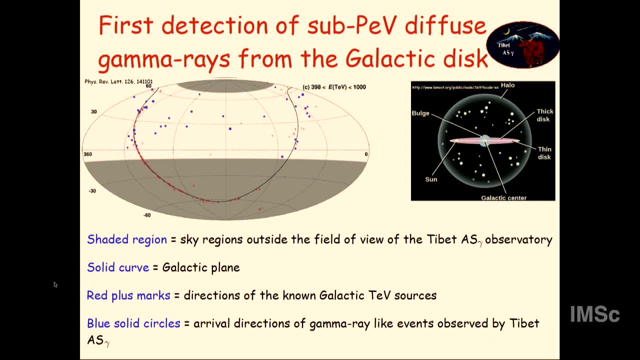 also observed these photons. All right, Yes, There is preliminary data set. LASSO is observing these photons and they also do not find any source, So these are two completely different experiments. LASSO is much better than Tibet AS Gamma, As you saw right, their first data set. they just beat us. 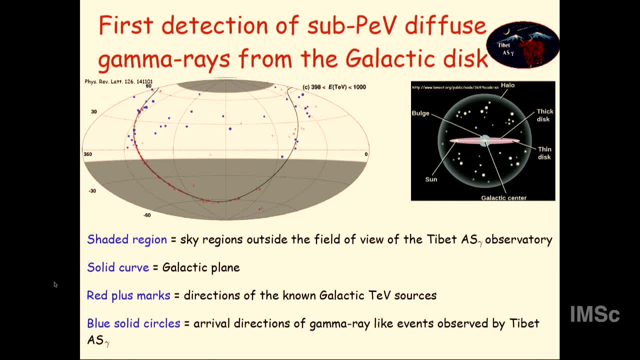 Sorry, Where is LASSO? It is in China, It is nearby, Yeah, So so they, they also do not find anything. And, and and you can, and there are other TV gamma-ray source, there are other TV telescopes, All. 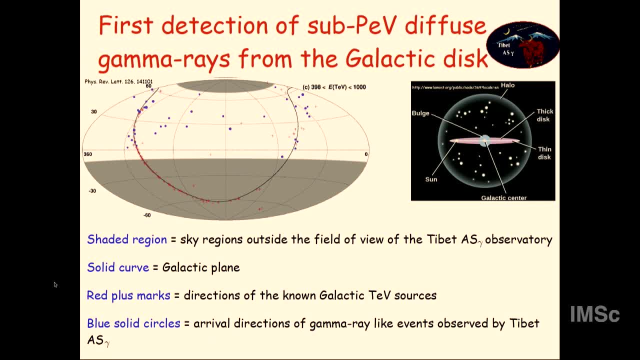 right. So there is something called. there is a telescope called Hawk. They also do not find anything here. by the way, There is no source that they find here, So no other telescope is finding anything here At at other frequency. at this frequency LASSO is also not finding. 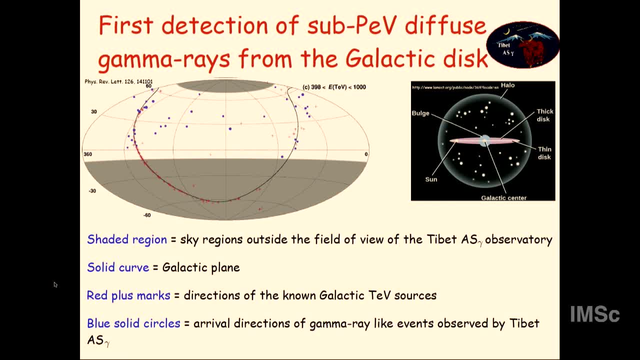 it So so this is actually. there is actually a collaboration of this thing. This is not yet published. It is preliminary, but it is almost certainly. they are not finding anything, any source there. That means it must be diffused. 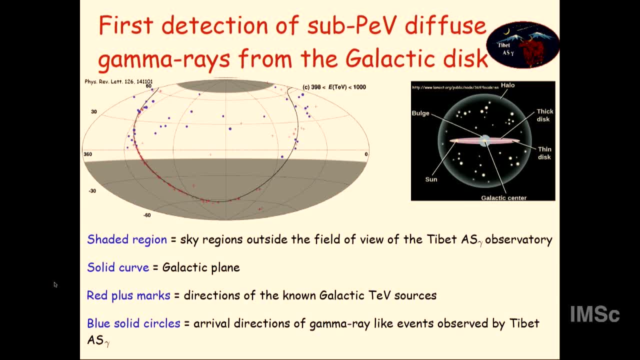 Okay, Yeah, Right, Thank you, I mean you can also, by the way, in principle it can be. it can be a source. You keep on observing it. Suddenly you see more and more photons say from here, And, and, and and. 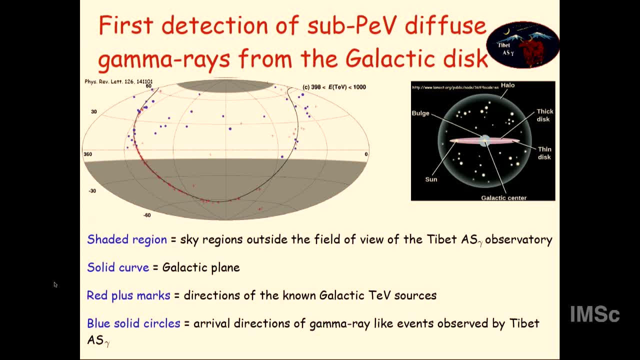 suddenly you see more and more photons say from here, not from here, That that is how you find that it is a diffused thing. Diffused means it is all spread out. Source means there is a bright, so you so you pixelate the sky, You pixel the sky and then one pixel. 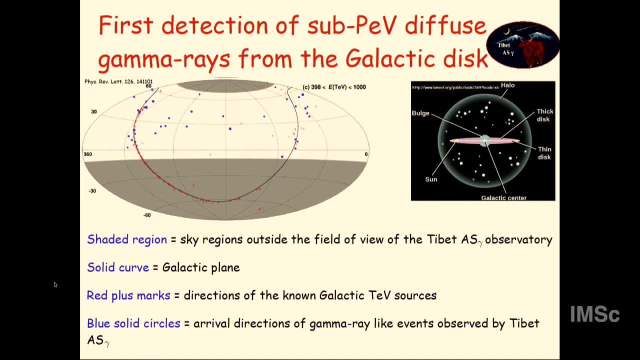 will have many photons. The next pixel will not have photons. Think of it that way. Right, If that happens, then then we know that there is a source, There is possibly a, there is possibly sources here. Currently we cannot say that: All right, That is a. it is a confusing. 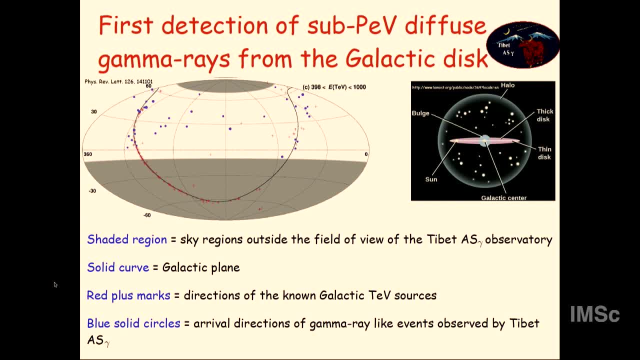 situation, but that is what it is. It is, it is last year's discovery, So it cannot be simple. Sorry, I need to cut this discussion and I request you to continue it in coffee and biscuits. Yeah, And thanks, Ranjan, again for this fascinating talk. Thank you And thanks for coming. 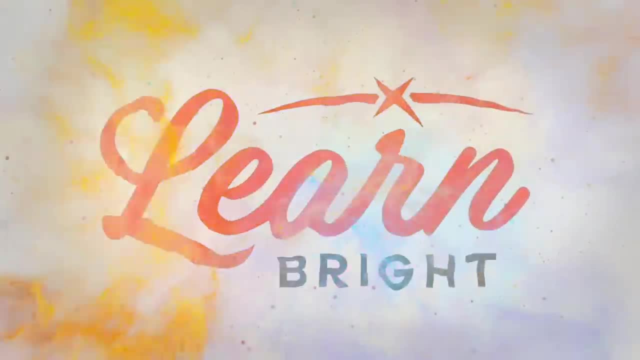 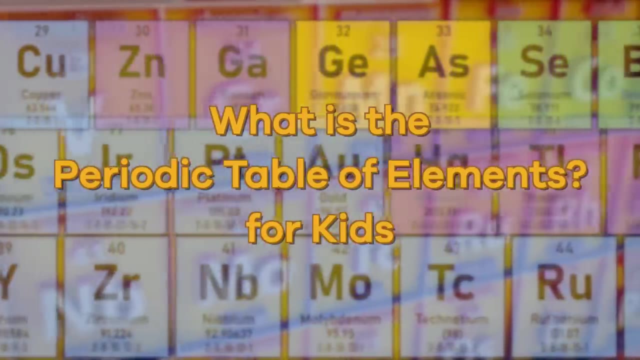 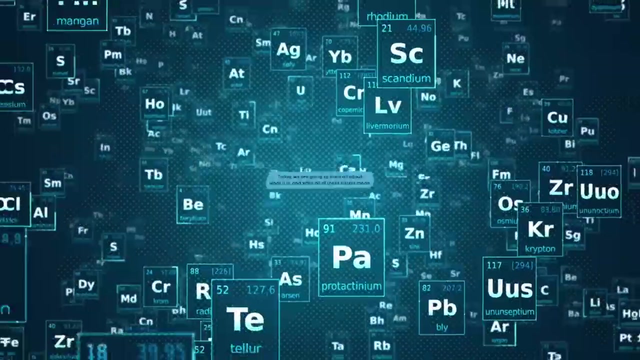 What is the Periodic Table of Elements For kids? Have you ever seen one of these charts before? This is called the Periodic Table of Elements, And today we're going to learn all about what it is and what all of these letters mean.